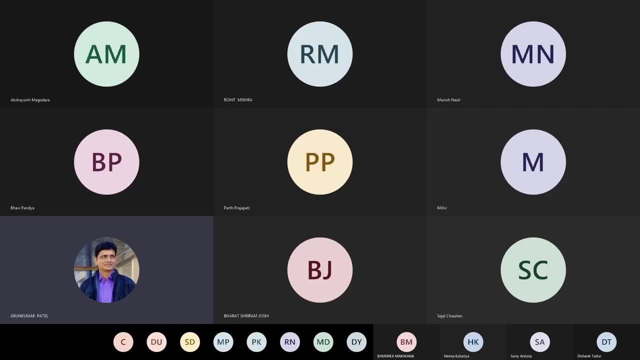 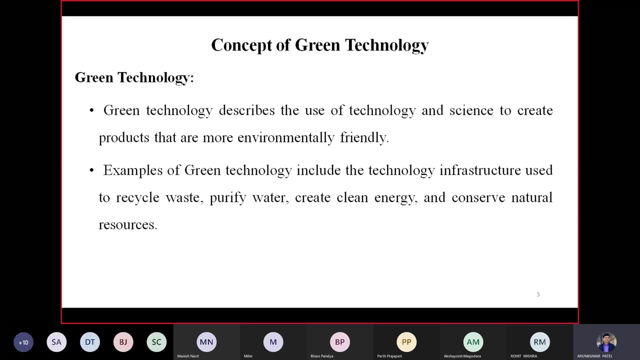 Utilize in a such a way that it can recycle that waste. We can purify that water and other contaminants. Moreover, that which creates clean energy and conserve the natural resources which is related to energy conservation, As we know, we have that so much natural resources. 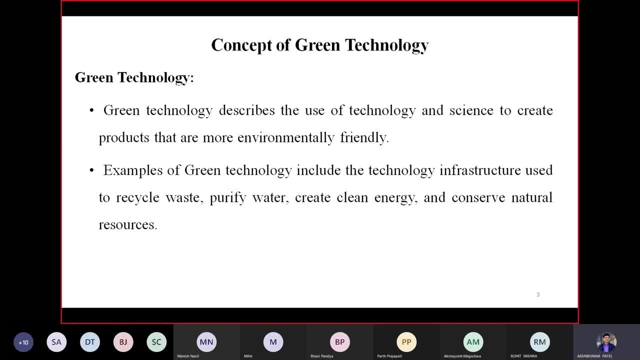 is depleting very fast, That conventional resources, which includes that basic oil, gas and other- I mean coal, that even nuclear resources, that all resources are depleting very fast. So we must have to conserve them for the future use also And whichever resources. 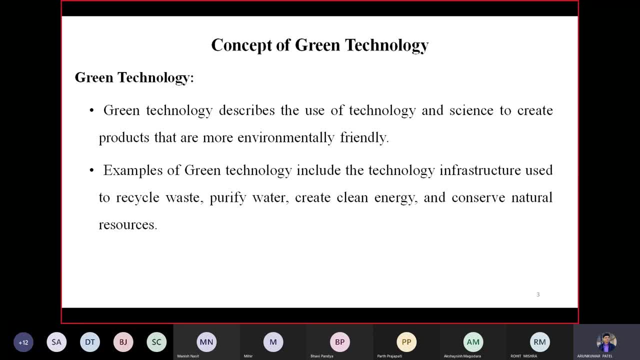 easily available naturally. which includes that- different conventional resources- Right now that research is more focused on that- which includes that: solar energy, You can say biomass energy or other mode of that energy. geothermal energy, You can say ocean energy. These are the different mode of energy resources which we can utilize in a proper 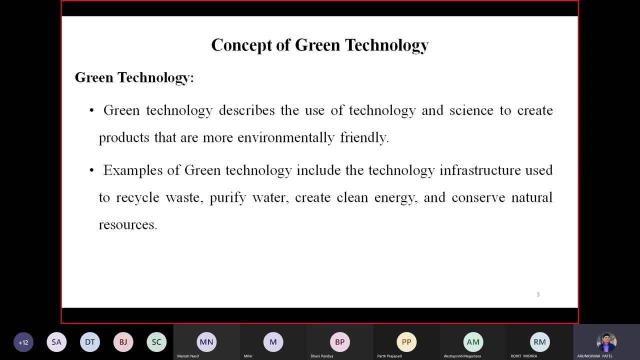 way, So that it is available in abundant form and we can- I mean- properly utilize and we can save our that resources which are very fast depleting, and that kind of technological aspects we can have to adapt, and so that by use of that kind of technological aspects, we can move towards. 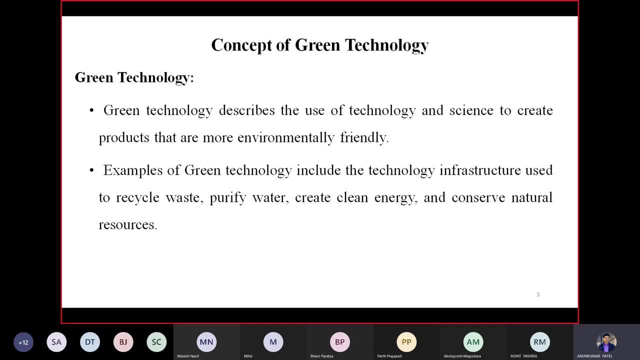 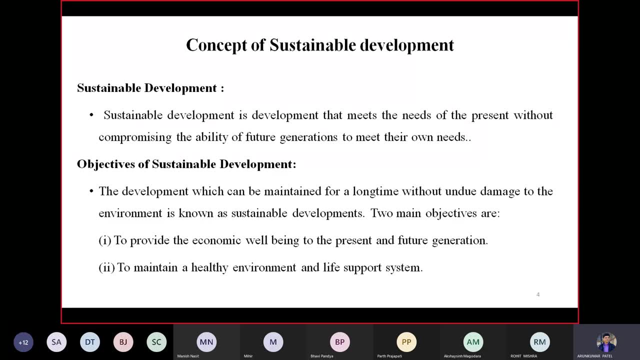 that green technology. So that is the basic theme of that green technology. Now we will come to sustainable development. So sustainable development is the development that meets the need of the of the present without compromising the ability of future generation to meet their over needs. 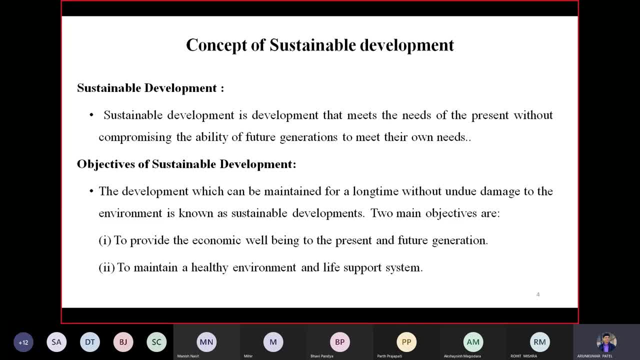 As I shared about that, resources which are very fast deflating. So sustainable development means which kind of development we must have to adapt so that we will have to fulfill this present needs without compromising that future requirement which will be required for the future generations. 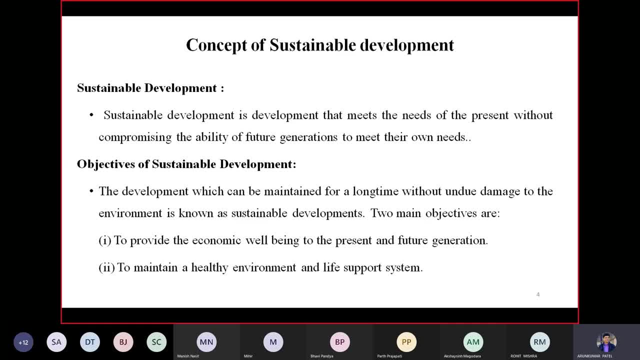 So we have to utilize that resources in a very economical way, or you can say very- I mean- conservative way, so that we can preserve them for a long period of time. So, and with that there will be a kind of that Growth, or you can say industrial growth also. we can achieve and economical aspects, or you 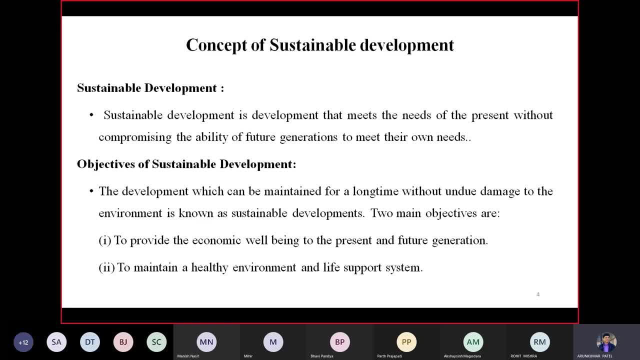 can say development aspects also. we can achieve So that kind of growth, we can say that sustainable growth in that sustainable development also. So which are the objectives which we have decided for the sustainable development- very important topic, The development which can be maintained for the long time without undue damage to the 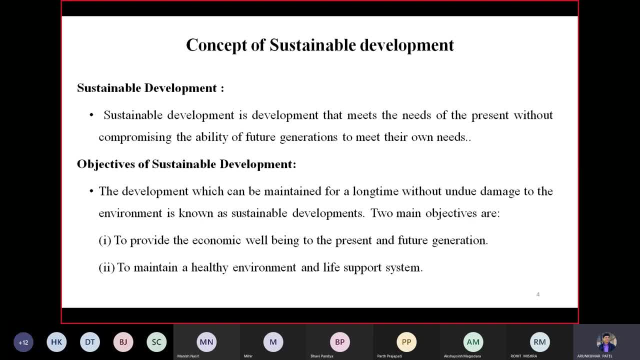 environment Right. So this is one of the more term of that sustainable development known as a sustainable development. That means we will have to preserve that, all the resources, without undue damage And by these resources what we can have to achieve that objective, that two main objective. 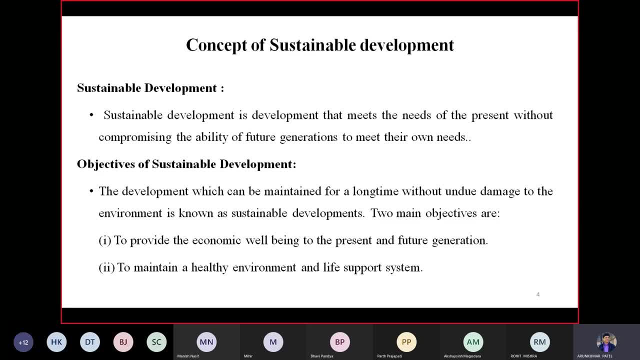 are to provide a economical well-being to the present and future generation. So economical well-being means so that we have to utilize the resources. We have to utilize that in a such a economical way that we can give, that we can fulfill that present requirement as well as future requirement by the optimum use of that kind of resources. 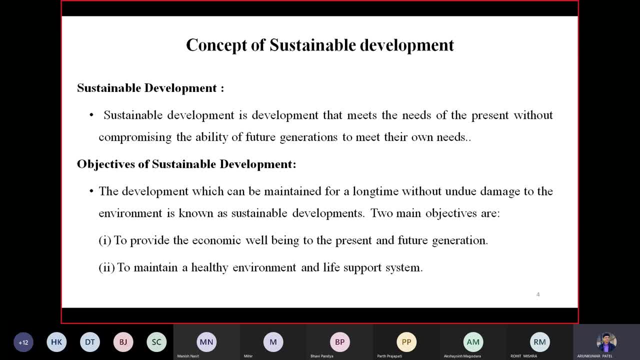 Right To maintain a healthy environment and life life support system. it is also one of the most important aspects Right. So right now we can see that kind of situation arising around us. it is really very deteriorate because We can see Right. 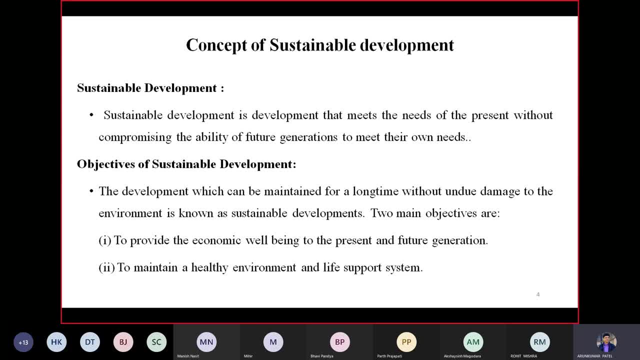 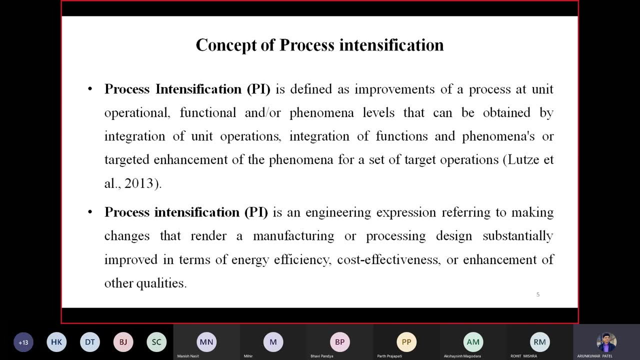 There are so many things which demanded more and more but we are not fulfilling that demand. So this kind of situation, it will be not happen in case of that. sustainable development objectives Right. So these are the objectives. Now we will move to that process intensification, concept of that process intensification. 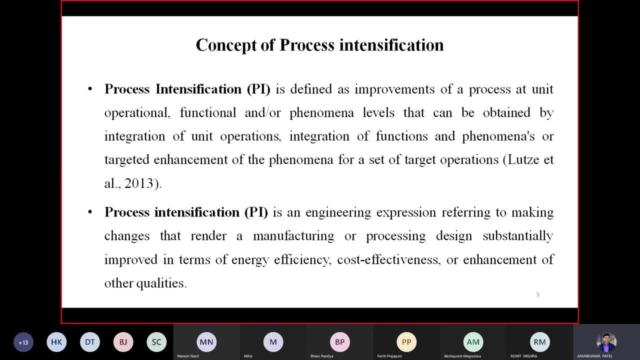 So as in when that green technology and sustainable sustainable development There must be coming to picture that process intensification to maintain that green technology and for the achieving that sustainable development We must have to play with that conventional processes So that we can modify that processes and develop new processes in a such a way that we can 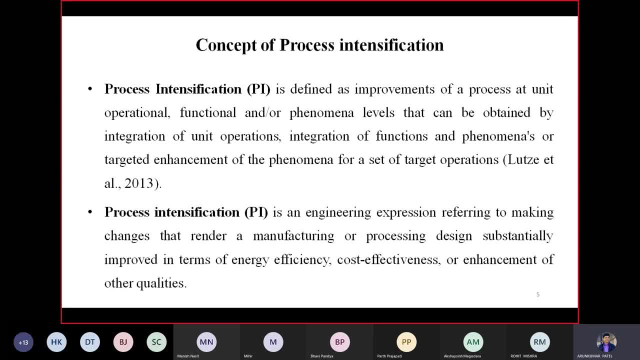 achieve That, whichever our requirement, or you can say product or processes which can give us that product in a very economical way, very efficient way and very energy saving way. So this kind of steps we are calling as process intensification, Let us move towards that process intensification, as we know that process intensification is. 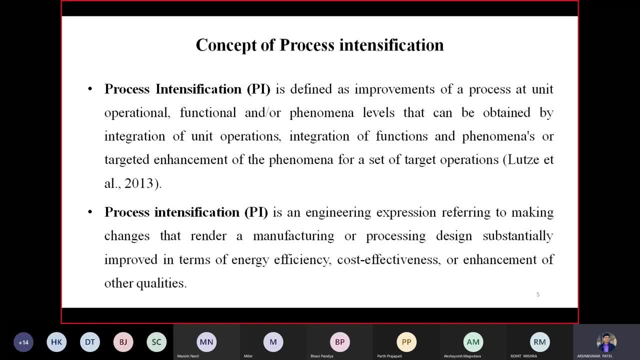 defined as the improvement of the process, as I said, At unit operational, functional or and phenomena level. that can be obtained by integration of unit operations, integrations of various functions and phenomena, or target enhancement of the phenomena for a set of targeted operation. It has been defined it by Lutz et al in 2013 means process intensification. we have a set. 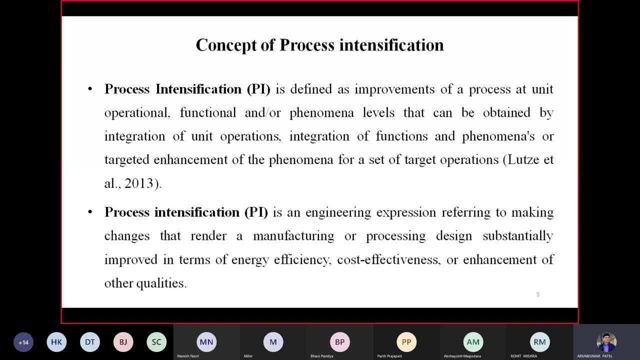 a goal In a such a way We can utilize minimum resources and we will obtain that desired product with efficient way. and for that, whichever technological change in terms of, you can say, unit operation or, in case of that, integration in processes, integration in various equipment design or 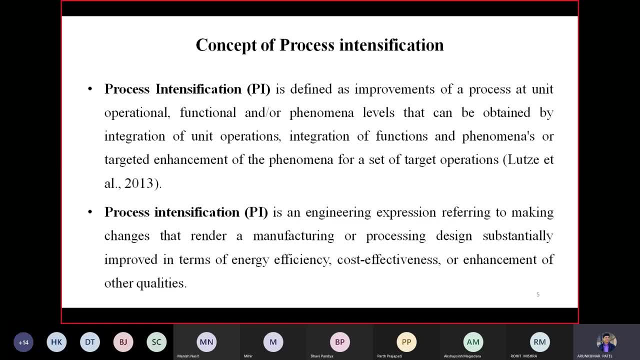 in various phenomena. We are doing little bit changes and we are modifying that path of process, or you can say equipment design or any other mode. So that is what we are trying to achieve And by that aspects we can do that various, we can develop that process in a such a way. 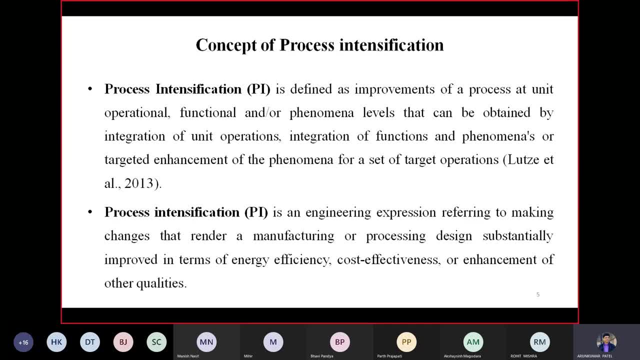 that design product we are obtaining. So this kind of changes which we are doing to make it economically viable and visible product, This is called process intensification. So in other way, process intensification is an engineering expression referring to making changes that render a manufacturing or processing design substantially improved in terms of 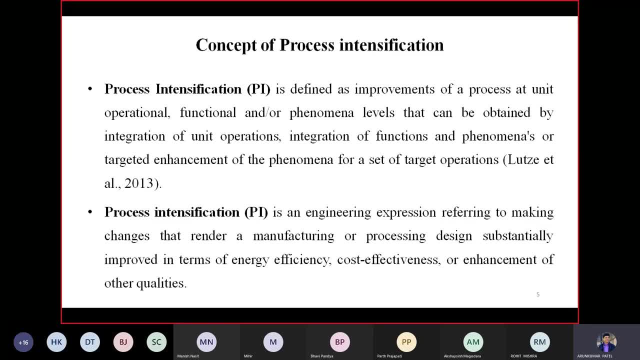 energy efficiency, cost effectiveness and or enhance of the other qualities Means. these are the parameters which must be enhanced whenever we are doing that kind of process intensification. So, as and when that process intensification term will be coming to a picker, we will always 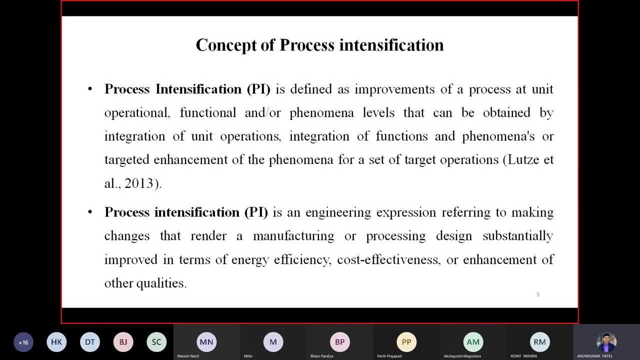 think about that. energy aspects: is it energy efficient technology? more over that also, we will think about cost effectiveness. is it economically viable? other quality parameters: is it maintained? more over that in case of that process intensification. we have seen in our previous lectures also that whichever technology we have adopted, is it a green technology. 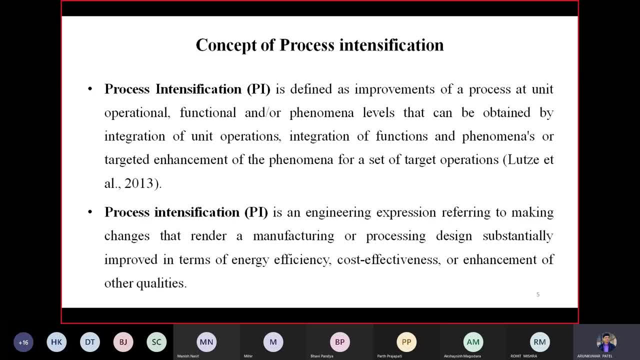 it is So we can say less polluting technology. whichever product or processes we are adopting, is it a really green? that kind of all aspects we are considering in this process- intensification- and ultimately our objective is to obtain that product or processes in such a way that 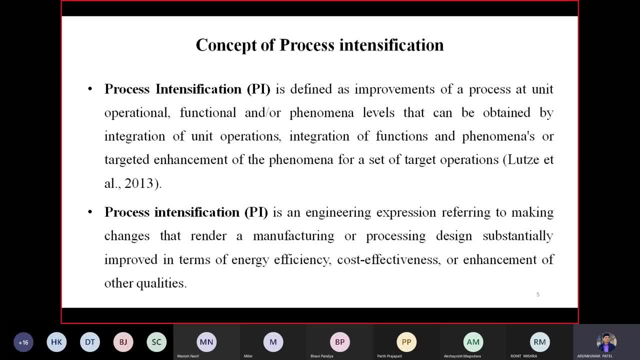 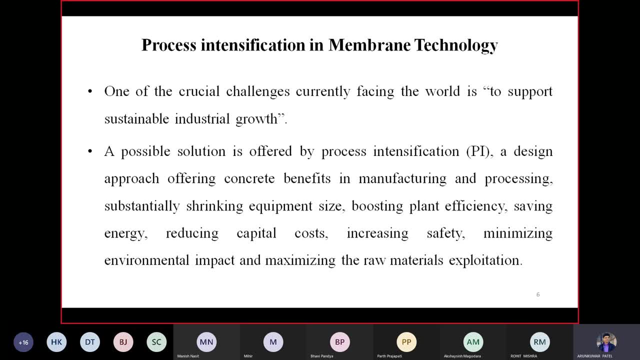 it will be efficient, cost effective and also maintain other qualities. Now we will come to that process intensification in membrane technology. So we will gradually move towards that process intensification. We will gradually move towards that our title of this session, that process intensification. 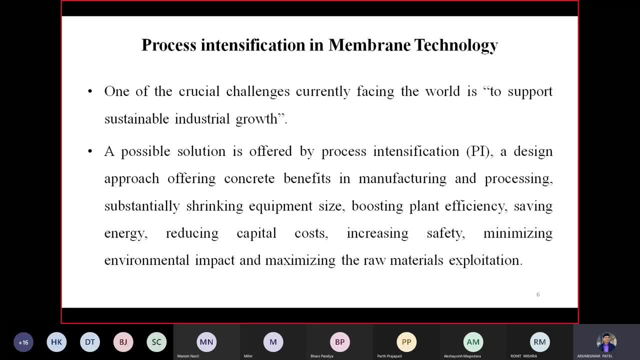 in membrane technology. But moving to that membrane technology aspects, we will see about the certain terms and basic fundamentals of membrane technology also, which includes various components of membrane processes, how they can club and how we can move towards the different types of processes and how we 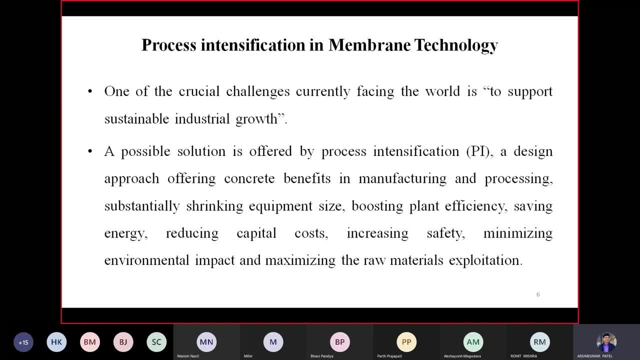 can club one process to another So that we can achieve that kind of process intensification. So we will see about that. also. One of the crucial challenges currently facing the world is to support sustainable industrial growth. It is right now, we can say, big challenges for all of us to support sustainable industrial. 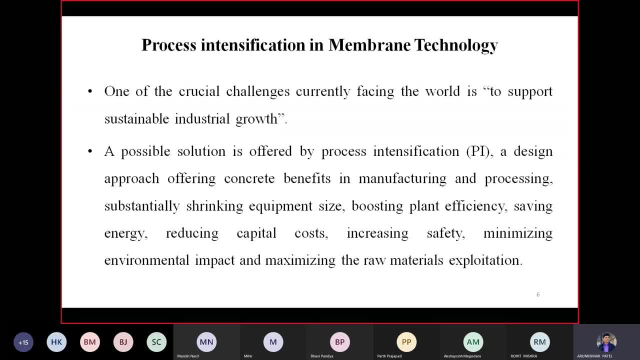 growth. I mean viable industrial growth. A possible solution is offered by process intensification, as I said earlier. also A design approach. A design approach, A design approach, The design approach is offering concrete benefit in manufacturing and processing which is related to adoption of that various process as well as product. 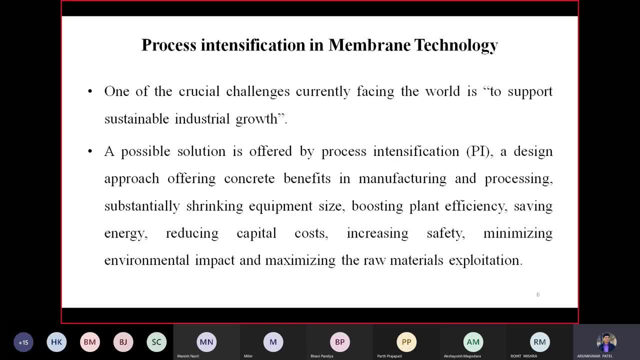 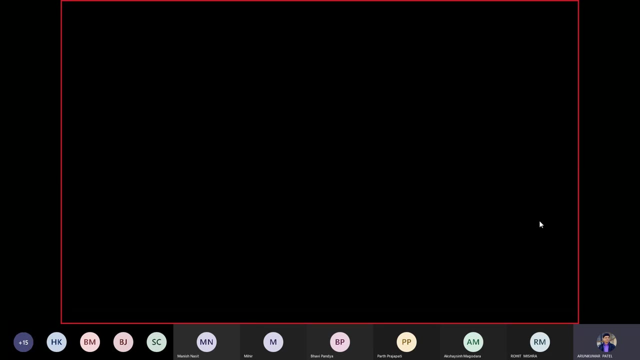 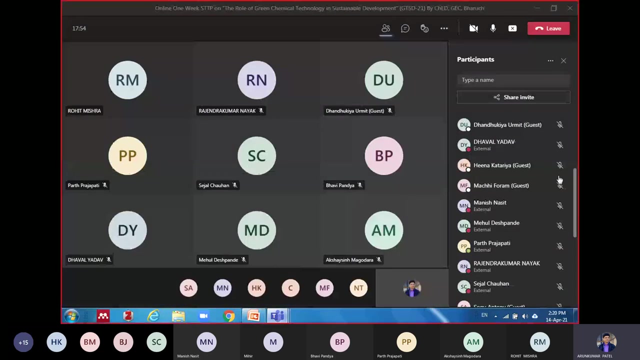 Sustainably shrinking equipment size, boosting plant efficiency, saving energy, reducing capital cost, increasing safety, minimizing environmental impact and maximizing the raw material exploitation. just wait for a minute, because I will have to do it in a recording mode. sorry for interruption. please bear with us, please. so I just come to know I will have to do that recording also. sorry for. 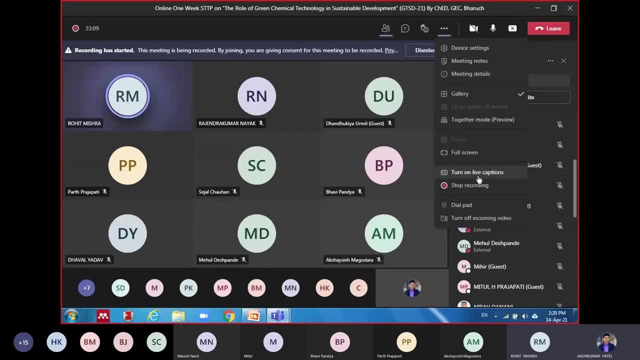 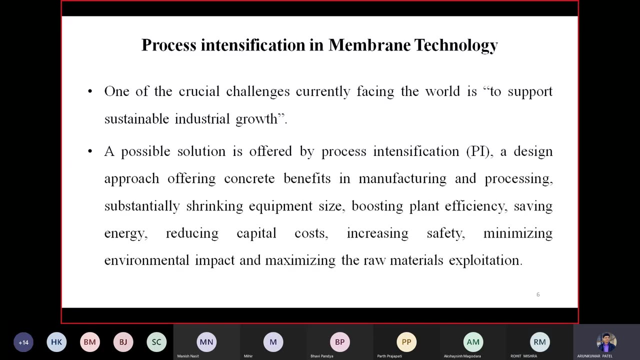 interruption because our whole recording okay, okay, just, I have seen you have started, sorry, sorry, because our team is also having yeah, yeah, yeah, sorry, sorry. so even our team is also having little bit problem. so we are coordinating our level best and our team members also. two to three. 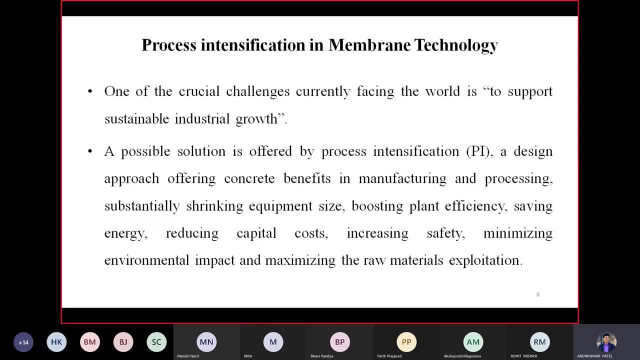 team members having also severe problems. so they are facing- and that's why little bit problem we are also facing at our end. even myself also. some participants know uh, I have also at my home- I mean positive patients also as well- as uh few difficulties from my side also. so please bear with us and we are trying to. 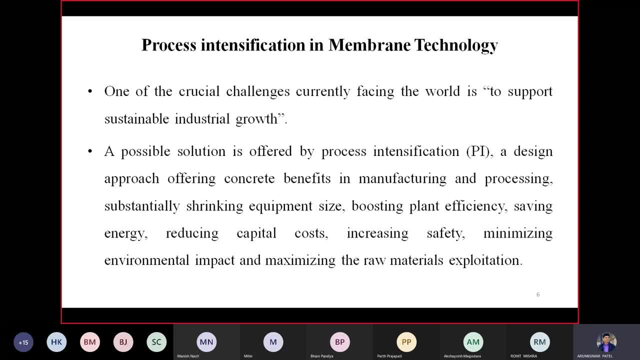 do whatever best possible from our side. and even I come to know that even participants also having affected in COVID-19- few participants also, I come to know they are positive. but please, I am really happy that even that situation also, they are attending this STTP and it's really 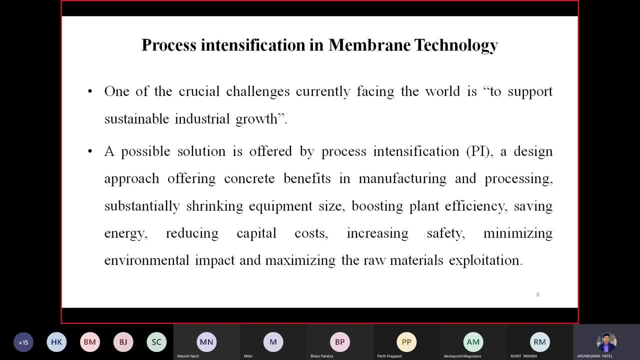 I mean happy moment for me that even in in in such kind of very deteriorate situation, we are conducting the session but hope we will do it in a proper way. so anyway, we will move ahead and we will complete it in a proper way. so let us come to our point: process intensification in membran technology. so 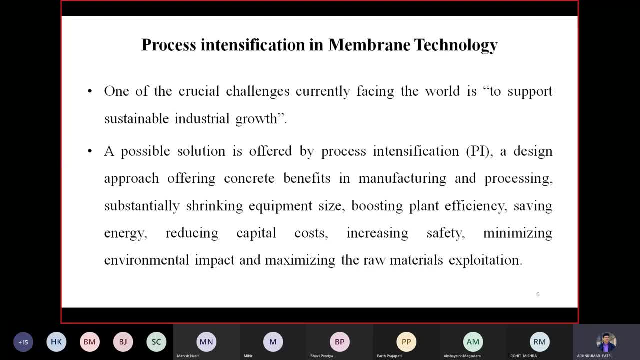 as I shared that whenever, whenever we are discussing about that process intensification, uh, and I do know, when I had using this 그러 pedagogical headings, that I was snake potentially. In that case, as I said that we must have to think about that, manufacturing, I mean. 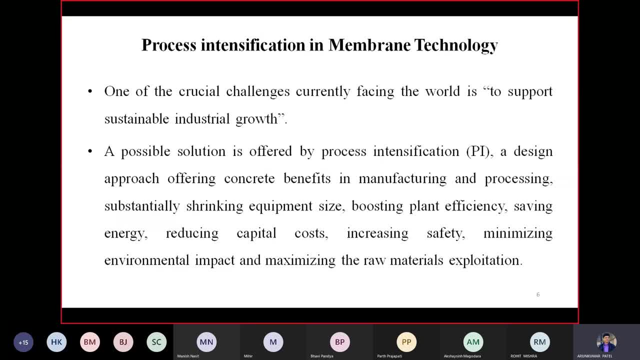 product as well as processing. Moreover, that if we will have to boost up that plant efficiency, we must have to think about that equipment size, various design aspects also by which we can save our energy, or we can say we conserve our energy And this way we can reduce our initial or capital cost. we can also increase the safety. 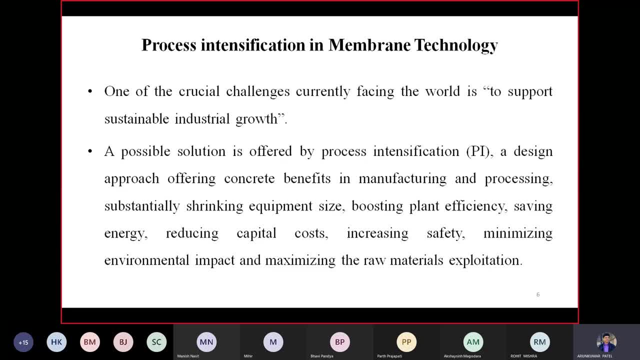 also And same time we can do the minimum, or you can say minimize the environmental impact which related to that pollution and that pollution generation, and I mean green aspects and maximizing the raw material exploitation Means. we will have to choose that way. So we have to process in such a way that all the parameters of that process and product 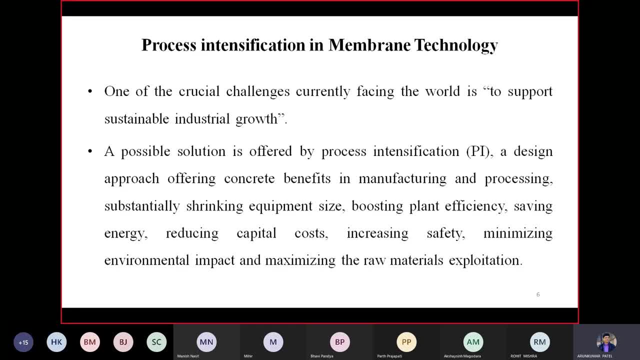 development must be optimized. So, starting with, as we know that in case of that, I mean, in terms of that, green technology, whenever we are starting with our raw material to product, we must have to think about the raw material, or you can say alternative raw material which we can utilize for the best. 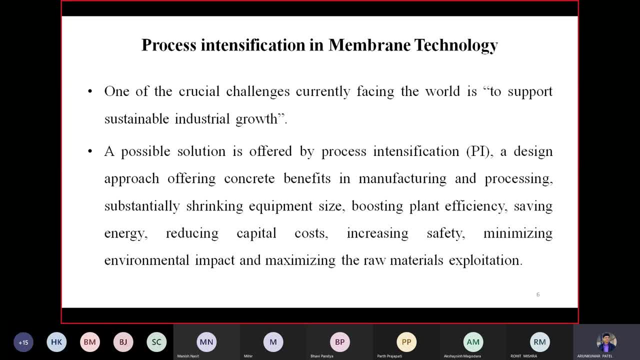 suitable and minimum polluting process also Okay. So we must have to think about that solvent also, so that it must create less pollutant, Even whenever there will be a side reaction or product development. the kind of reaction mechanism also we have to select in such a way that whenever we will come to end of that 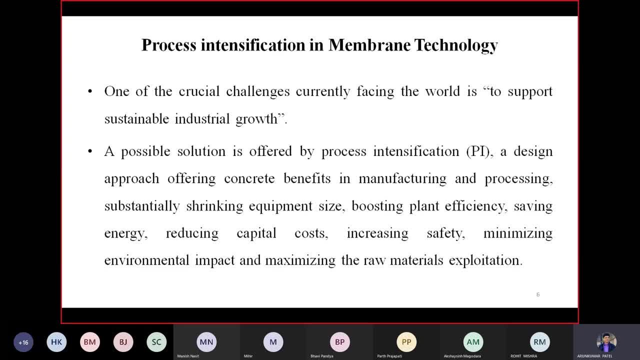 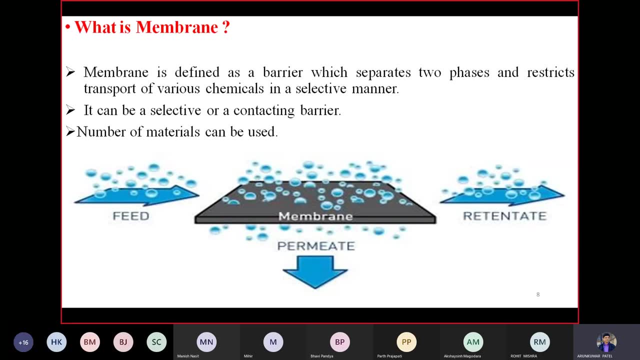 process and at the stage of that product development we can generate minimum waste and utilizing minimum energy. This way we can do that process intensification. Okay, Now come to that conventional membrane technology. So I have to just go through that basic terms of that membrane technology also. 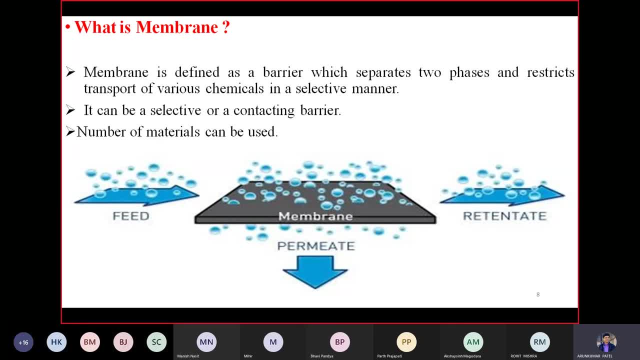 As we are knowing about that terms, membrane. membrane is defined as the barrier which separates two phases and restrict transport of various chemicals in a selective manner. Means, when that term come into picture, that membrane, we must think about the kind of filter, medium, Right. 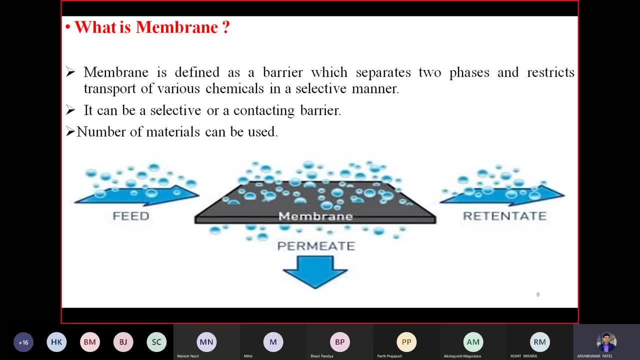 So it is not a conventional filter medium, what we think? because it is a simple kind of septum. whenever that membrane come into picture, everybody- I mean it is with reference to, I mean students I am talking about- they just imagine that it is a simple kind of that. 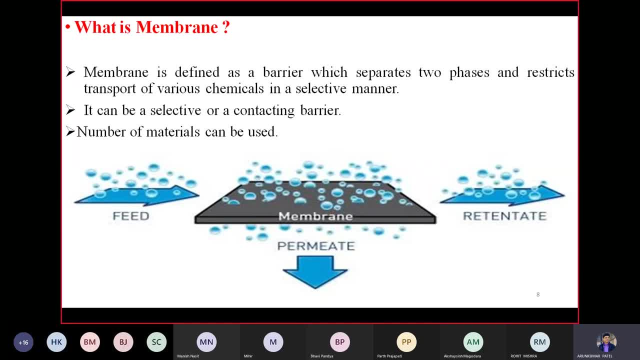 barrier which will restrict. it is not like that. So it is having a multiple layer septum on which we can have, we can retain that selective layer, So that means the particles in a selective matter and whichever permeate will be that. 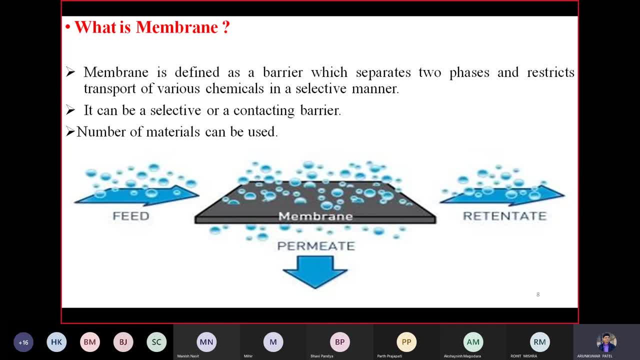 that will be passed through it. So it will be behave in a selective manner which will restrict certain particles in a certain way, based on its characteristics, And it can be either a selective or contacting barrier. So number of different types of material which can be used. 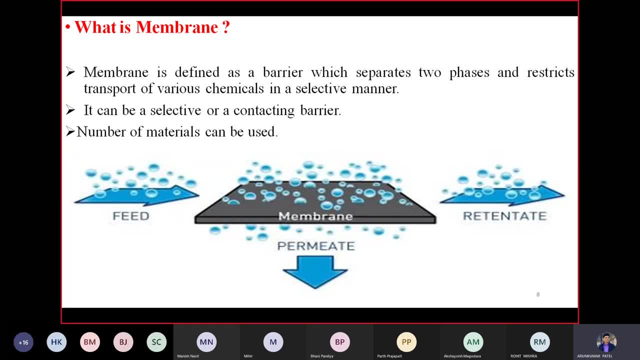 You can see over here how we can carry out that membrane separation processes. Initially, field will be there, passing it over the membrane surfaces. you can see that over that surface area and whichever retentate will be there, they will be retained on that surfaces and whichever permeate will be there. 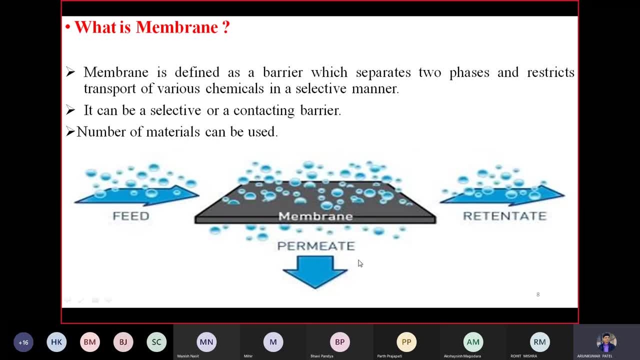 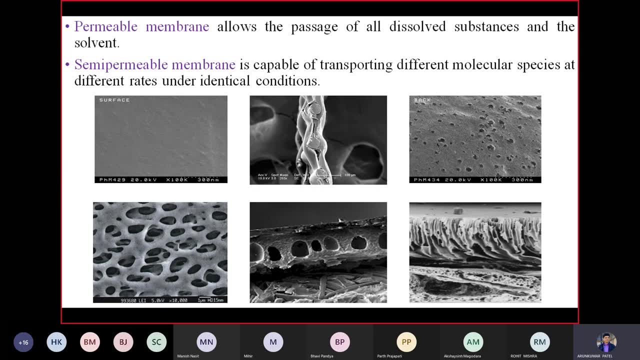 there will be permeate through its pore, membrane pore, right, so it is kind of terms even in membrane technology also permeable membrane and semi-permeable membrane. permeable membrane allow the passage of the all the dissolved substances and and dissolvent i mean whichever. 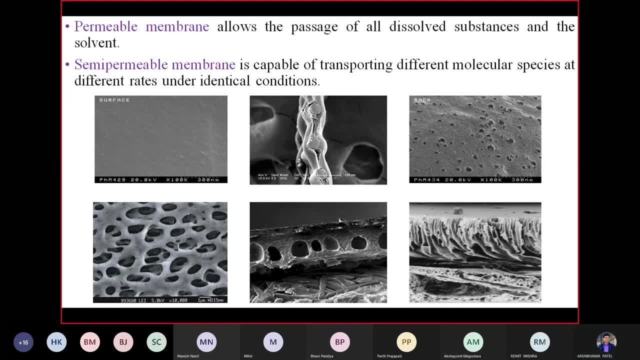 that dissolved substances and solvent will be there. if it will be a permeable, then it will be allowed to pass through it, but in case of semi-permeable membrane it is capable of transporting different molecule spaces in a different rate under identical condition whenever we will see. 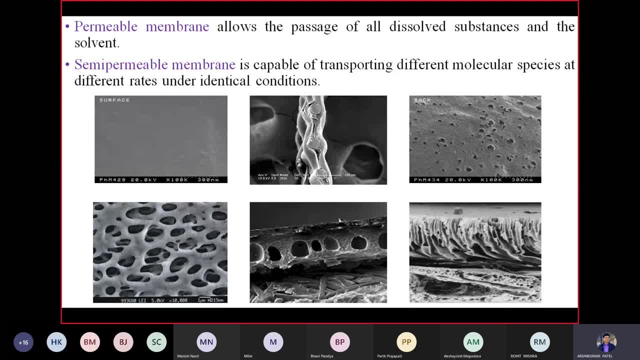 about that characteristics of that membrane, so that membrane, surface and even material have a certain kind of permeability, so that membrane, surface and even material have a certain kind characteristics which will retain certain particles and which will allow certain particles to pass through it. this, this image- you can say same image which i have put over here- how that pore. 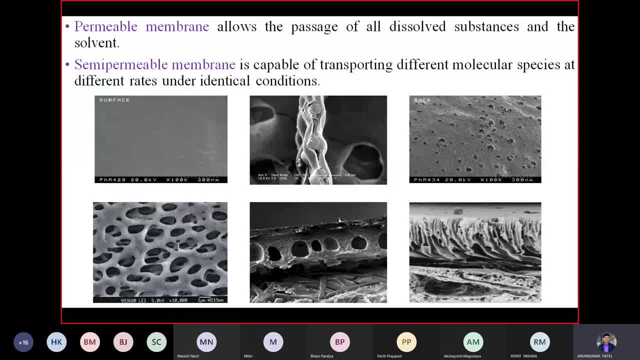 size we can visualize it is. i mean micro porous, nano porous, or even more than that pore size. i mean less than that pore size. so this, this porous structure that we- it is shown over here through that same image. we can see that this is the perimete from which that perimete can be passed. 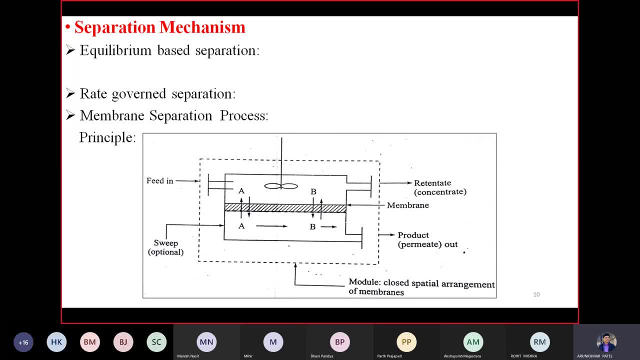 so it is basic separation mechanism as we are familiar with that equilibrium based separation, uh certain things which already kaushik nasa has also discussed in his presentation. so equilibrium based separation in mass transfer, that conventional operation we have seen. once that equilibrium will be established, then that power, i mean uh process will be stopped. so in that case we can see that we 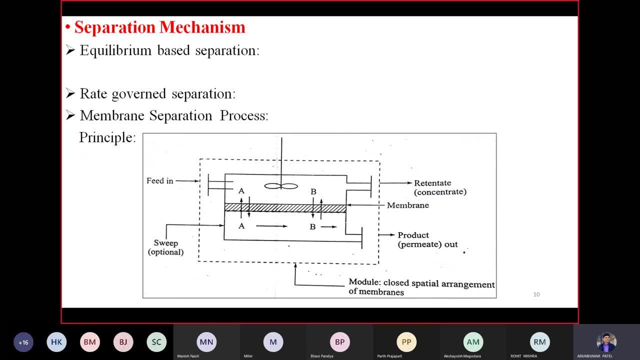 can see that and then that is where we can see that this is the perimete, which is the perimete. so in that mass transfer operation, but over here in membrane separation, it is rate govern separation technology. so that means there will be a certain driving force which we must have to apply. if you 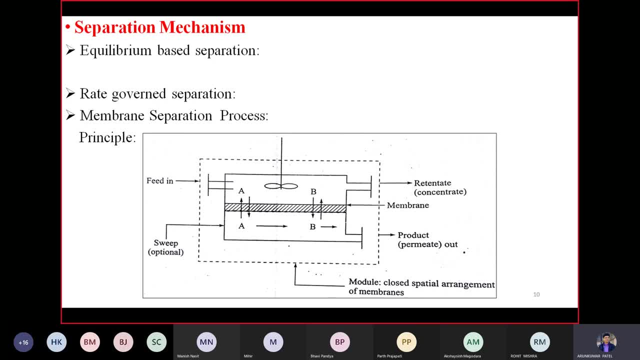 will apply that higher driving force, then there will be a higher separation. so depending on that driving force, there will be a separation will be taking place over here. you can see in this it is kind of module which we shown over here in schematic diagram. Over here we are passing. 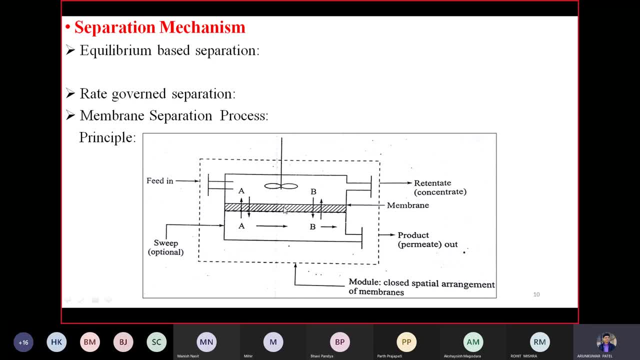 that feed material. It is a membrane, it is supported on a structure and we have that A and B. It is two spaces which we will have to pass through that membrane. One space is that will be retained on membrane surface as a retentate and other one will be passes. 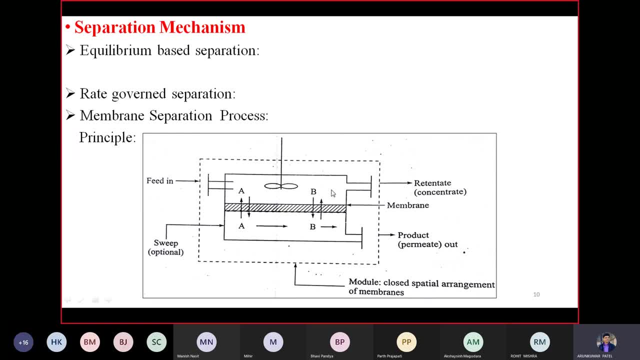 as a product. But whenever that retentate and permeate that will be separated, that retentate particles that will be retained over the surface of that membrane and that product which we will obtain as a permeate that will be passed through that pore of that, 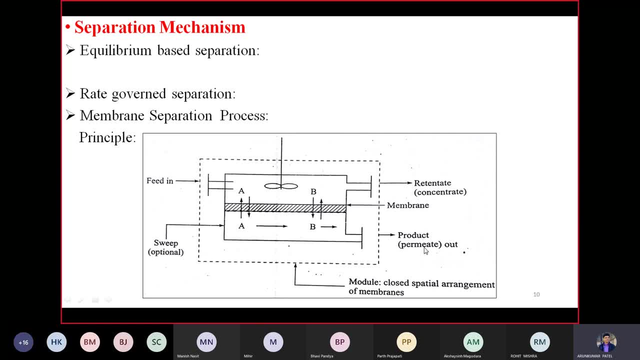 membrane and ultimately we will get product from here. But over here you can see both arrows which show that certain particle, micro or you can say nanoparticle- that will be mixed up with very minimal amount. So that is why both there will be a kind of little bit mixing. 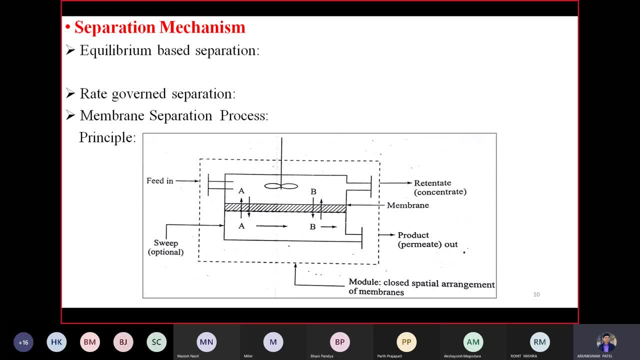 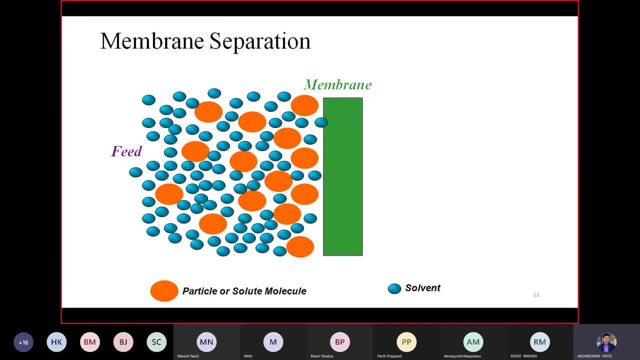 or you can say permeation of that undesirable component will be also possible. So this is the basic separation process. You can see over here, membrane, how that separation will be taking. You can say particle or solute molecule and solvent. Solvent must have to. 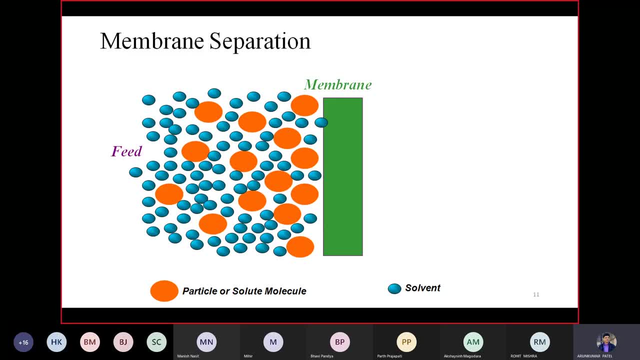 pass through that membrane or you can kind of permeate, which we must have to allow. So this way it will be moved and very little amount of that particles, very less amount. you can say that will be passed through membrane but almost that permeate, which is our desired. 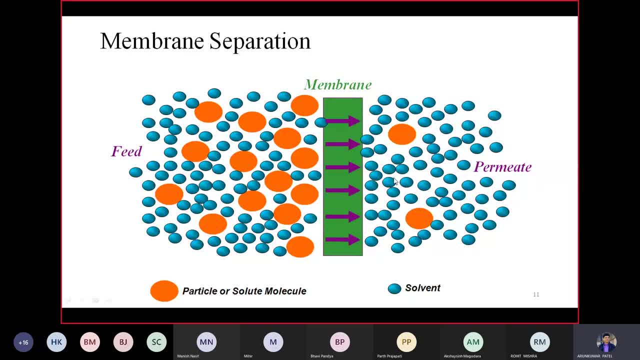 product which we are expecting to pass through that membrane pore. that will be obtained as a permeate And remaining whole particle that will be retained at the membrane surface So that larger particle which you can move, you can pass through that membrane. So this: 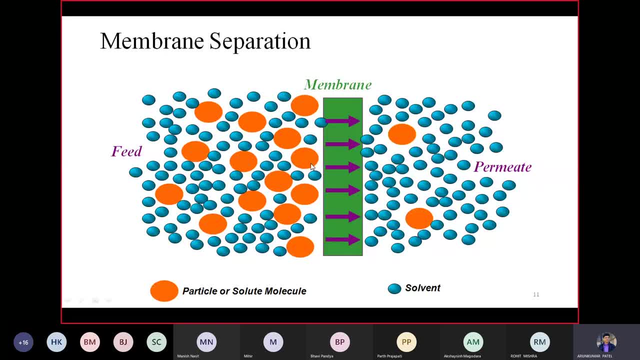 is the basic separation process which you can show, that orange bubble- that all will be retreated on that membrane surfaces and only permeate, having smaller molecules that will be passed through that membrane pore. This is the basic separation mechanism. But to carry out this permeation there will be a 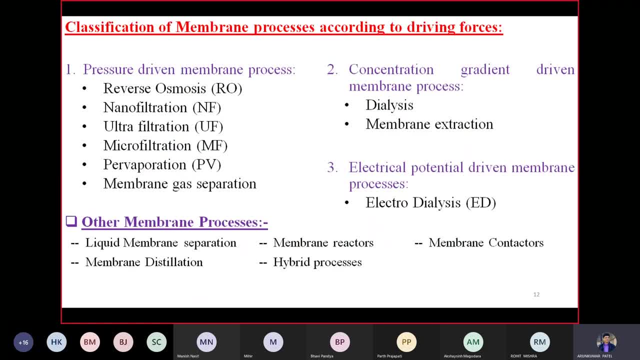 driving force required. So based on that driving force, we have classified different membrane processes according to its driving force. As we are familiar with that, we have that pressure driven membrane processes, concentration gradient driven membrane processes, electrical potential driven membranes and other membrane processes also. Professor N R Vagalasar has also explained. 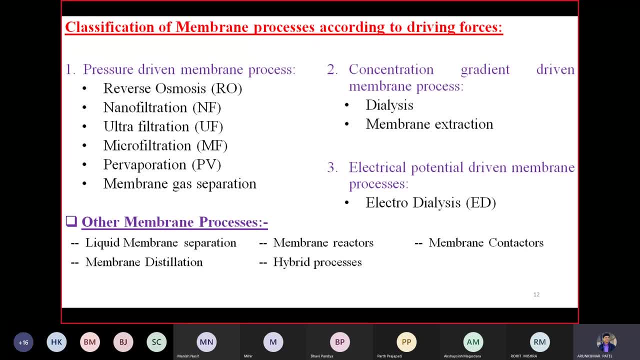 about the electrically driven, that separation mechanism. So in case of pressure driven processes we are familiar with that reverse osmosis, nano filtration, ultra filtration, micro filtration, pervaporation and membrane gas separation. These all are pressure driven membranes, Means in that case driving force will be pressure and that concentration gradient. 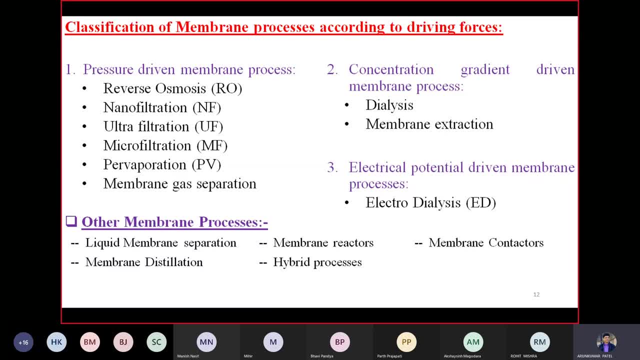 between two solutions that will be arise. In that case also, there will be a kind of balancing situation will be arise and that moment of one solution to other solution will be happen based on its concentration gradient. that includes dialysis and membrane extinction. Moreover, that electrical potential driven membrane with that phenomena will be occurs based on 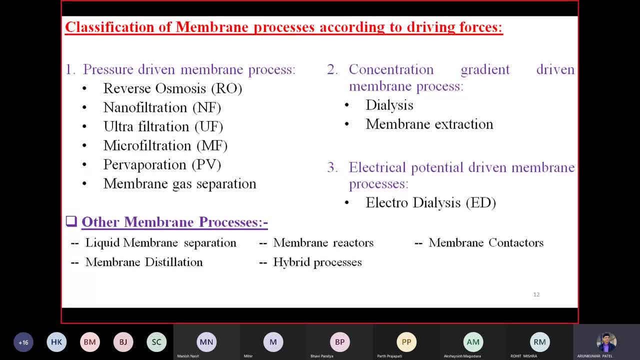 electrically charged atoms, or you can say ions, that positive charge and negative charge, ions. that is electro dialysis process. But this process we will more discuss on that pressure driven membrane processes, which is industrially more viable and more usable technology. Moreover, that other membrane processes, which includes liquid membrane, separation membrane. 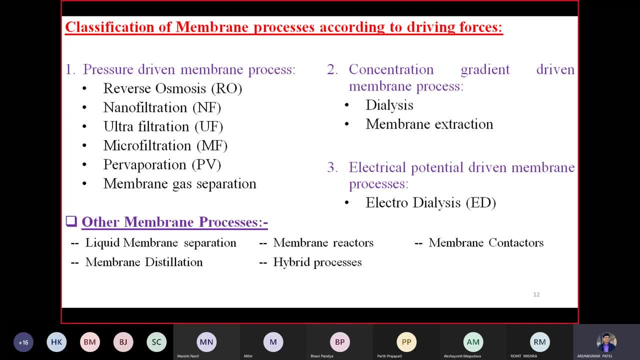 reactor, membrane contact, Membrane distillation and other hybrid processes. It is more or less you can say: membrane reactor, membrane contact and membrane distillation. It is also one kind of that hybrid processes in which we are doing I mean reaction as well as separation. So this kind of processes we are. 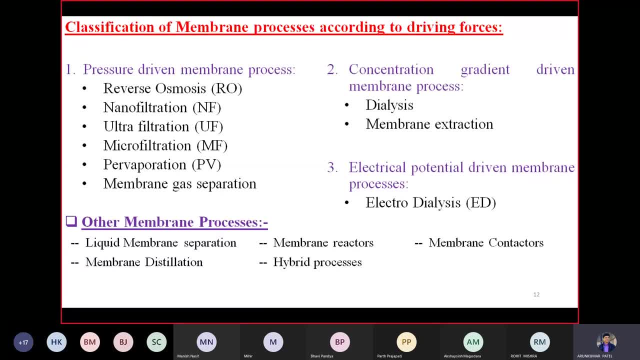 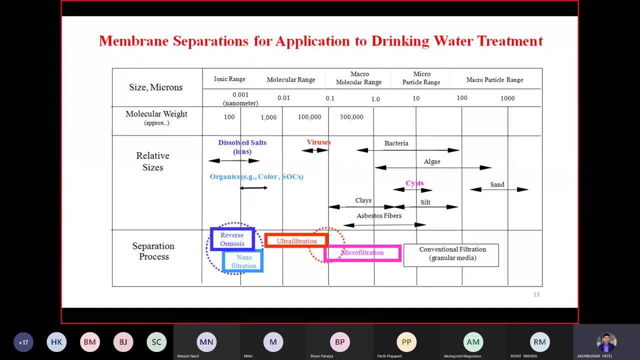 calling as that hybrid technology which we are utilizing for the process intensification purpose. This chart I have shown over here That membrane separation for application to drinking water treatment. over here, that size exclusion mechanism. Suppose it is a pressure driven processes, in that case you can see at the top size micron size over here: 0.001, 0.011,. 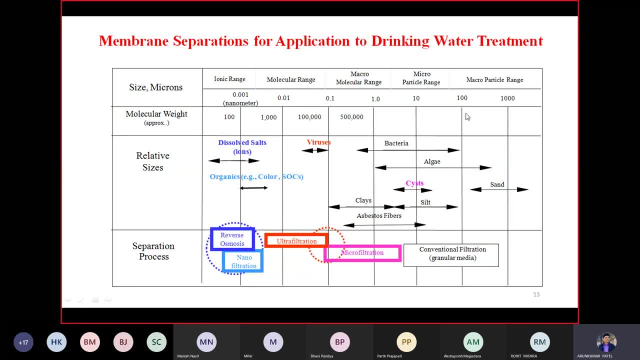 1, 1, 10, 10. this is micron size, given in micron. So based on that various relative size particle We can separate out over here you can see it is macro particle which includes that sand that we can filter out by the simple conventional filtration method. 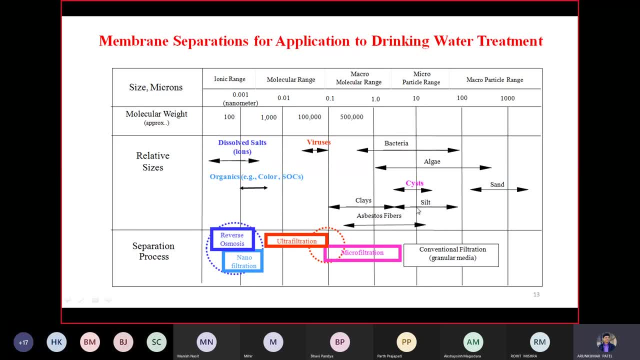 Moreover, that bacteria algae crust right shells, clay and asbestos fiber. it is having that size, of micro size. So for separation of this kind of molecules we can utilize that microfiltration, but beyond that, if that I mean molecule size, will be very less. in that case we will viruses even. 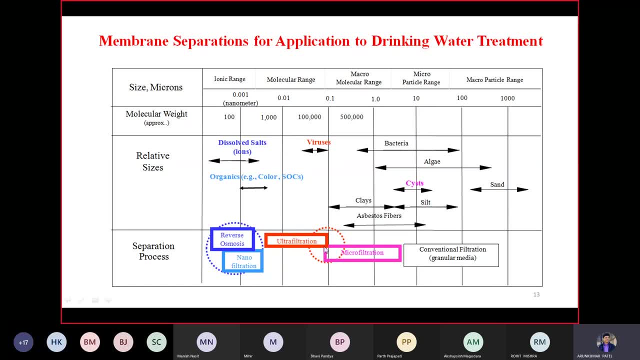 that has size of 0.1 micron or less than 1 micron. So in that case we are utilizing that ultrafiltration and ions basically that dissolve salt and organic Other separate out, that we are doing that reverse osmosis and nano filtration I mean. 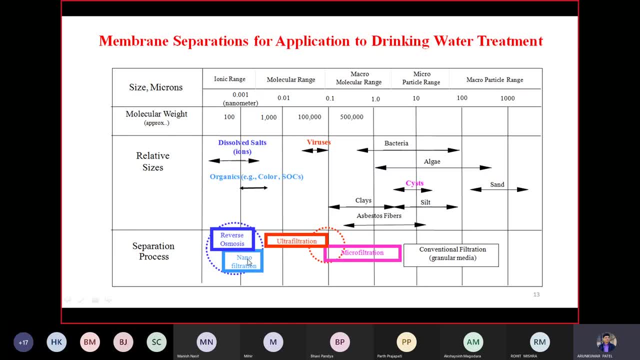 monovalent and that we are generally separating by that reverse osmosis process, That nano filtration which is intermediate operation of that reverse osmosis and ultrafiltration. So sometimes we are calling this ultra osmosis instead of that nano filtration. 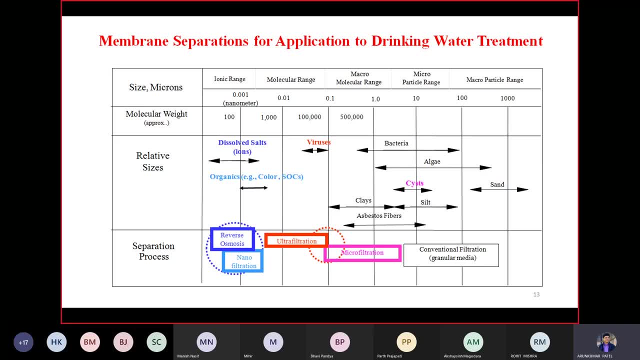 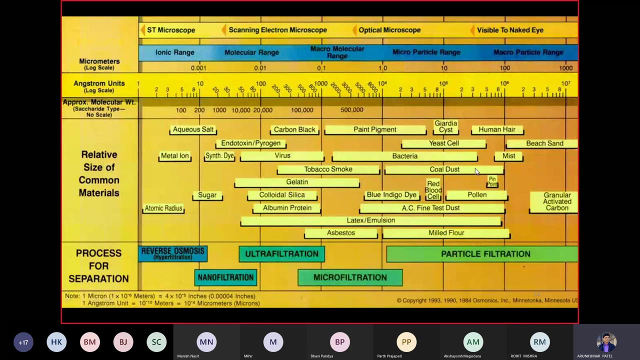 So these are the separation processes which That will be driven by the pressure gradient, I mean, and that various size exclusion will be taking place based on its particle size. right over here It is similar kind of you can say the content which you are observing over here. 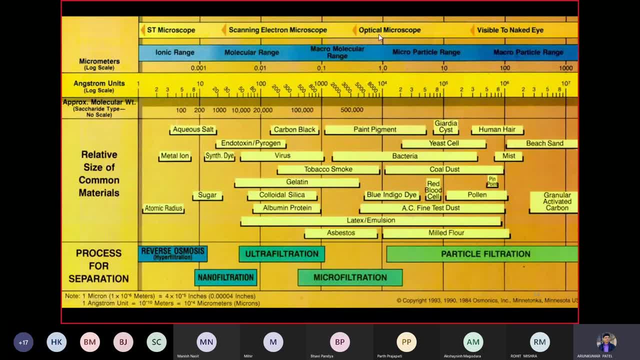 It is macro particles which is visible to neck-tie, even that. particle filtration, conventional filtration, granule activated carbon, bent sand, mist, human hair, even you can imagine, right, These are the- I mean different materials which we can conventionally filter. by that 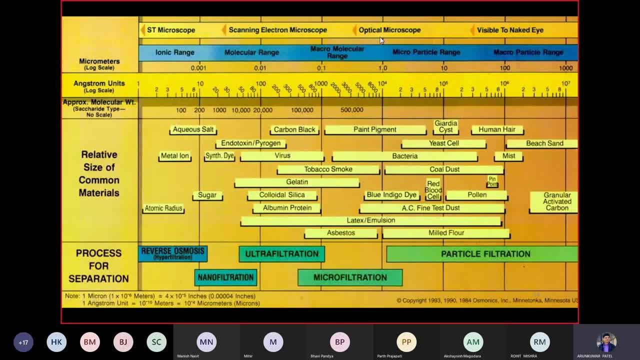 particle filtration and which can be visible to neck-tie, But beyond that it is visible by use of that optical microscope scanning electron microscope, ST microscope, And these are the ranges by which we can carry out the detection. So that is what we are doing. 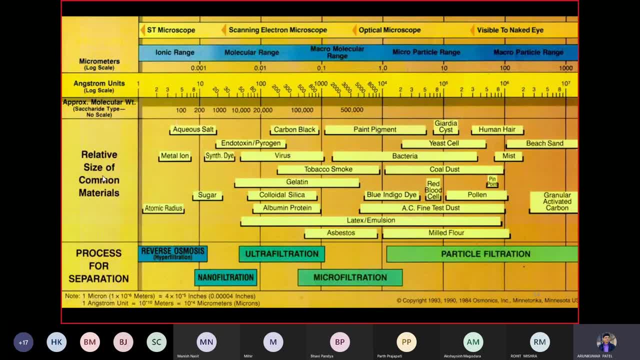 We can carry out the different processes. It is similar to that previous one, but over here that common material- it has been mentioned over here- like paint and pigment, it can be separated by that microviruses. it will be separated by ultrafiltration and nano filtration: sugar, metal ion or even atomic radius monovalent. 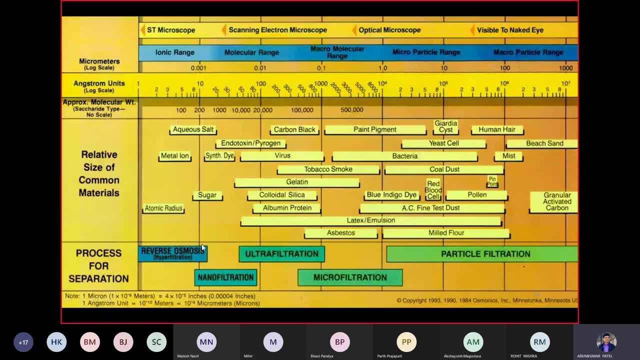 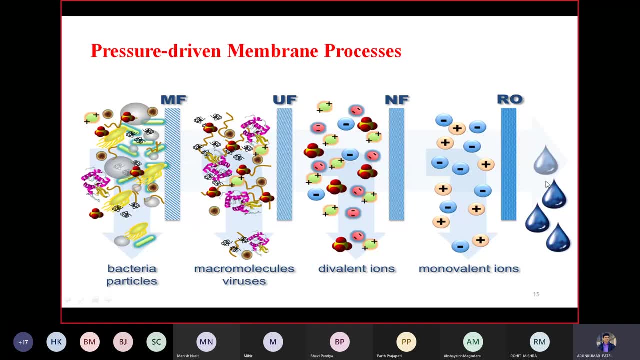 type of that atom that can be separated by your osmosis. right Over here you can see how that particle filtration can be done. So that is what we are doing: How that particle will be retained and ultimately, that pure water we can achieve. or water, or 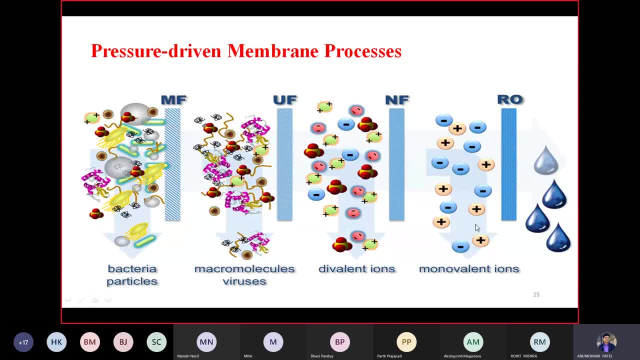 you can say that monovalent ions that we can achieve through this pressure driven mechanism Over here, that micro size particle will be retained- ultrafiltration, nano filtration- and ultimately, that spaces will be retained, step by step, and ultimately you can get that pure water or whichever your desired product. 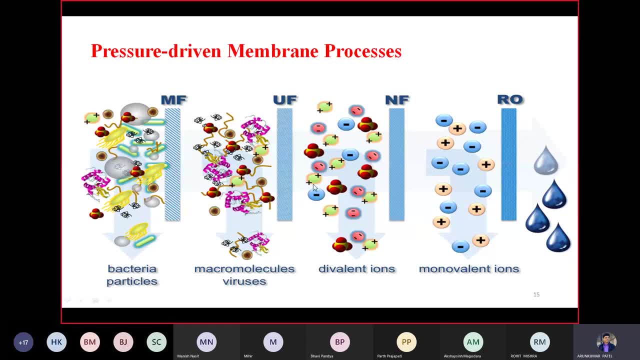 Okay. So sometimes you cannot directly use that RO. in between that also you can couple that micro filtration or ultrafiltration based on your feed material requirement. So that why we need to go in this way also. it is also just. I am sharing example of process. 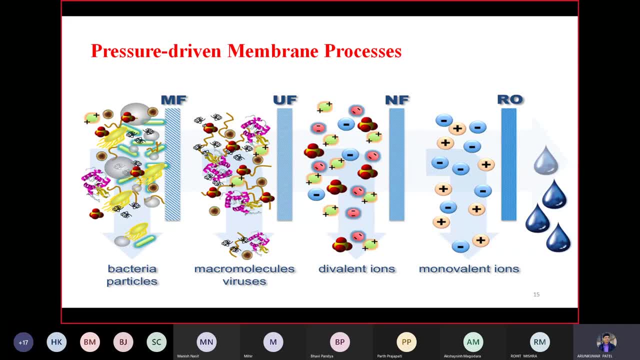 intensification. Why? Because whenever there is no need of that kind of reverse osmosis process, it requires very less amount of spaces which will be retained on ROs. So better is the process, Okay, Okay. So after that you can utilize beyond that previous ultrafiltration or microfiltration. 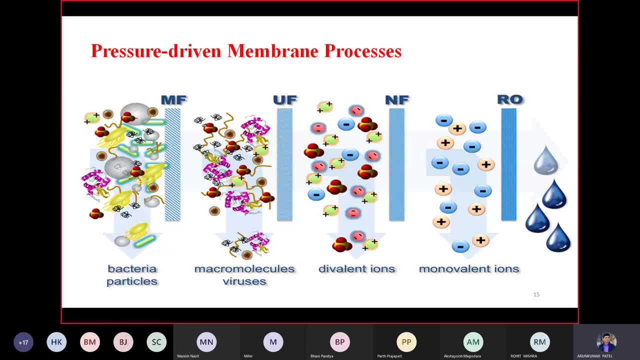 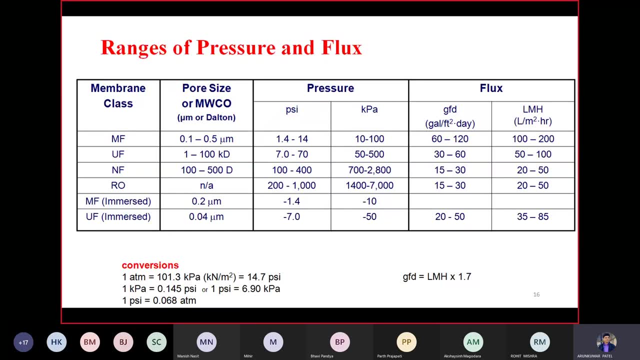 and after that you can retain that remaining spaces on that RO module, RO module. So this way also you can separate out by clubbing that various technology. So over here you can see it is similar pore size: microfiltration, ultrafiltration, nanofiltration. 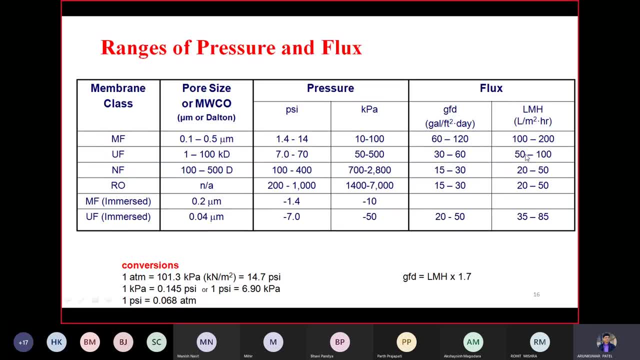 RO Over here, just whichever flux that will be retained. Okay, Okay, So the flux that will be remained, it is the volume. flux means whichever permeate that will be passed through that membrane surfaces, the volume of that permeate, which. 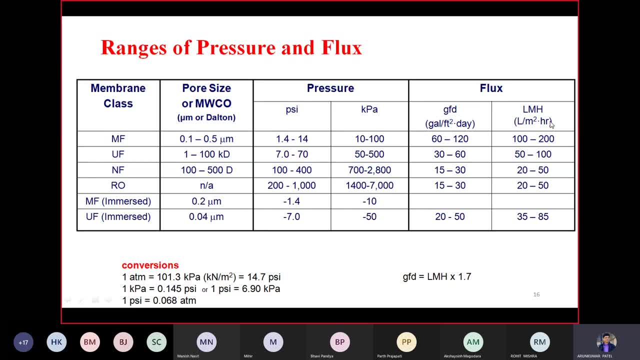 will be passed per meter square, with respect to time per hour or you can say any unit. you can say So: volume divided by its surface area. So volume divided by its surface area is equal to volume divided by its surface area. Okay, 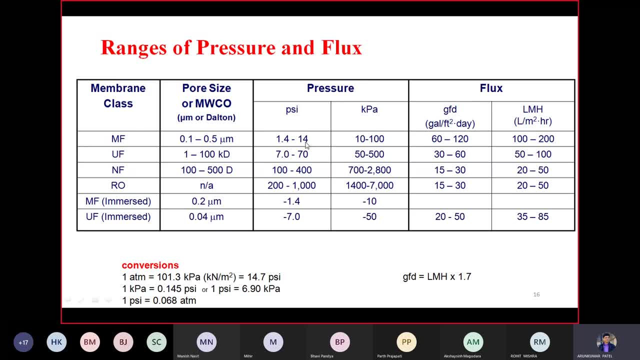 Okay, And whichever that desired product, we are getting right So this way, and its capacity, So how? even that pressure requirement? over here you can see how we are applying that pressure, As gradually you will move towards that microfiltration to reverse osmosis, gradually we are increasing. 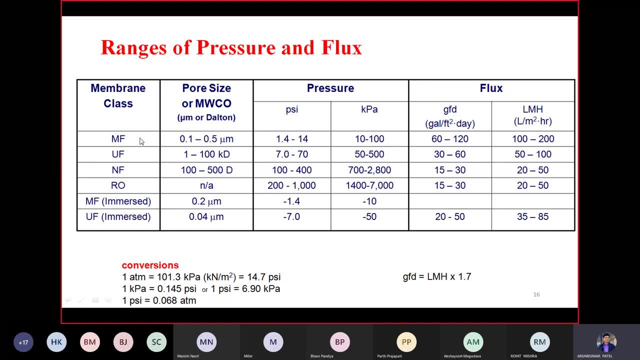 that pressure. So in pressure driven technology, membrane filtration required very less, Okay, Okay, Okay. So pressure compared to that of RO, and as that pore size will be reduced and particle will be retained in RO, that energy requirement, what I mean to say over here, that energy. 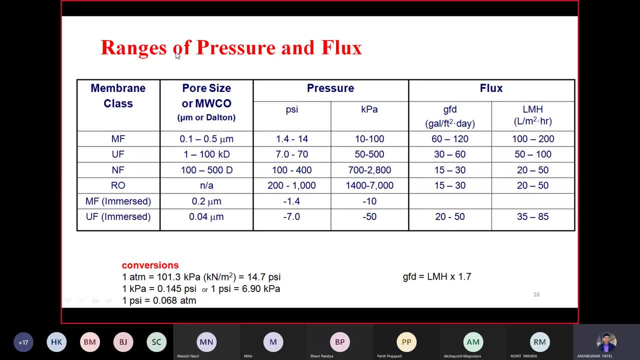 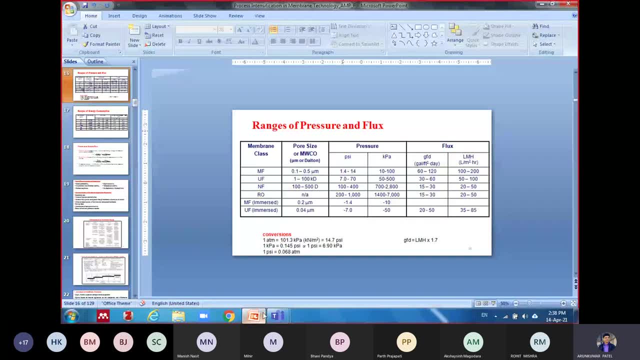 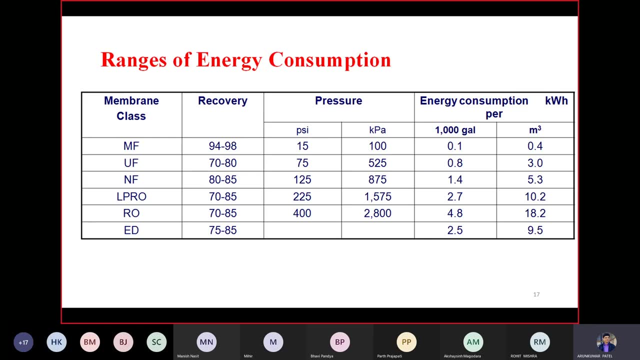 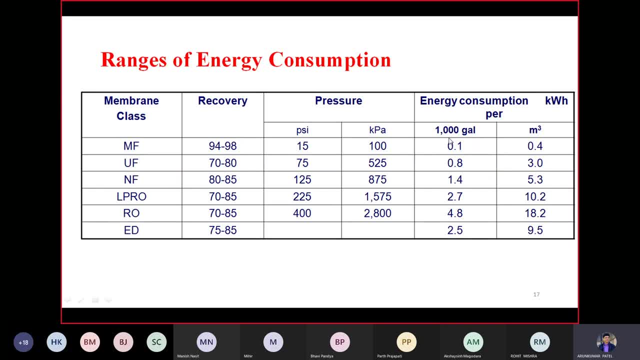 you can see over here, Energy consumption will be for the energy consumption per 1000 gallon or per meter cube volume of that permit. You can see over here membrane filtration: it will be 0.1 kilowatt hour UF in case of .8.. 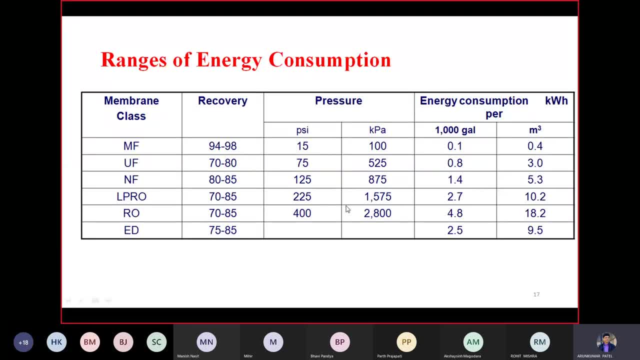 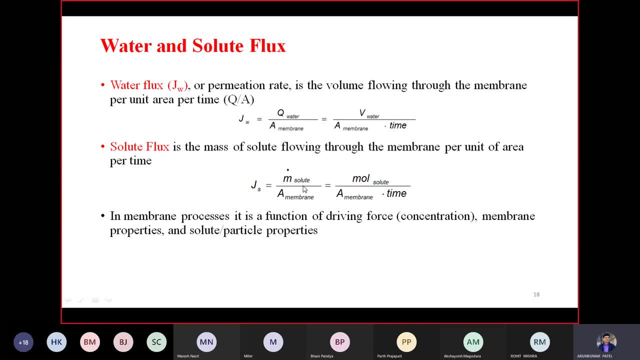 NF 1.4 kilowatt hour In case of that RO. it will be highest in case of pressure driven technology over here. Now, as I said, that water flux and solute flux, whichever permeate we are getting through that membrane, that will be our permeate flux. it is the volume flowing through the membrane. 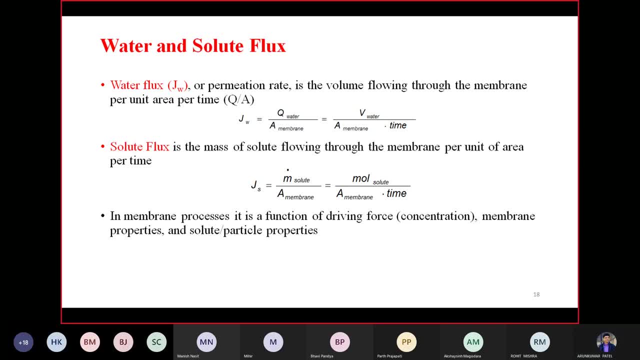 per unit area. per time means whichever amount of volume we are, that permeate we are collecting. per unit means it will be a membrane surface area. Can you know that we have the different types of- I mean membrane module also? that also we will see. 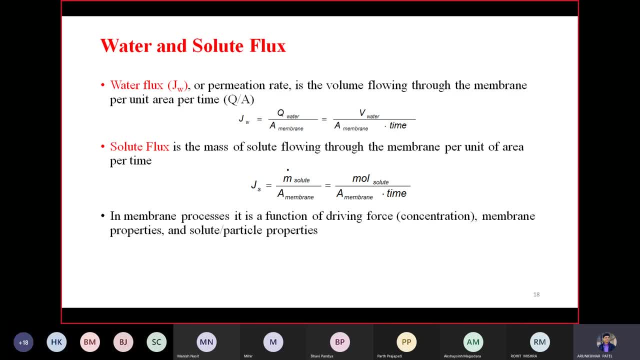 So that surface area from which we are passing, that also matter a lot. So, this way, that whichever amount of that water- I mean water or you can say permeate flux- we are getting, moreover, that solute, the mass of solute flowing through the membrane. 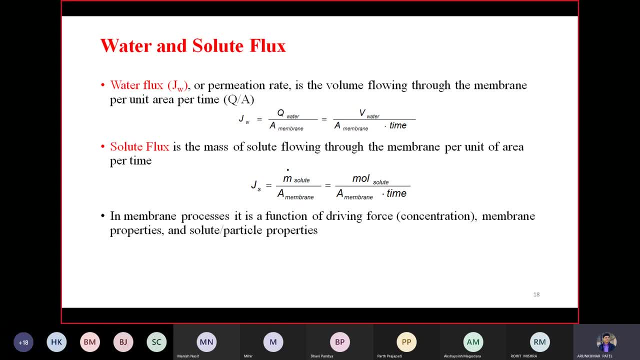 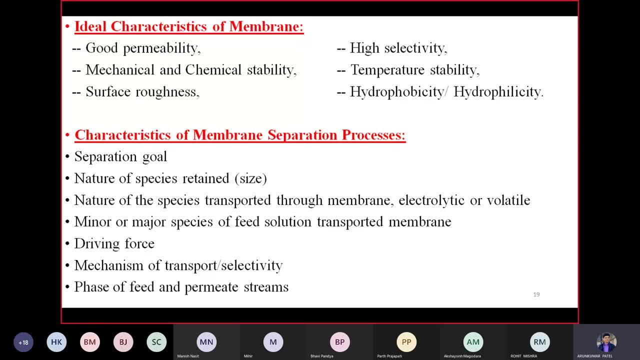 per unit area, So the surface area per unit time. it is similar to that, So it will be a flux which we are getting through that membrane processes. So which are the ideal characteristics of that membrane? So the ideal characteristics of membrane which includes good permeability, mechanical and 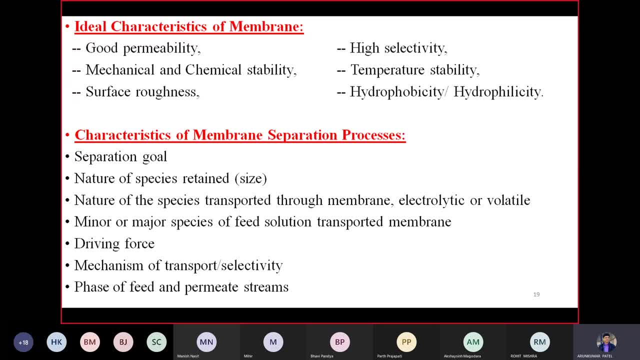 chemically, mechanically as well as chemically stable, surface roughness, high selectivity, So that in that case only we can get that desired permeability. So we will see that, Okay. So in that case I do not think that this kind of main objective 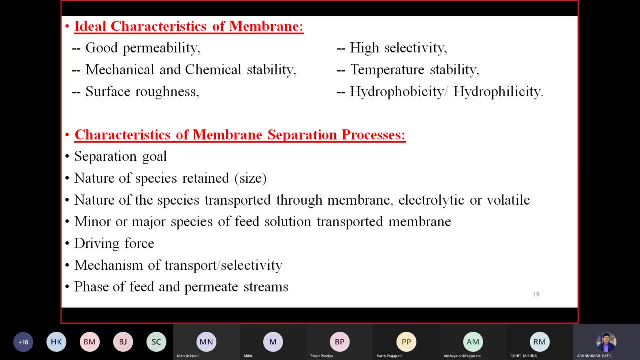 So any other further? yes, So. So again, you know- this is almost gushing down- thatiye, wet layer, wet institution. Therefore, there are so detailed steps to be taken to make sure that this is up-to-date, is made available to all, therefore, as a complete solute to use. 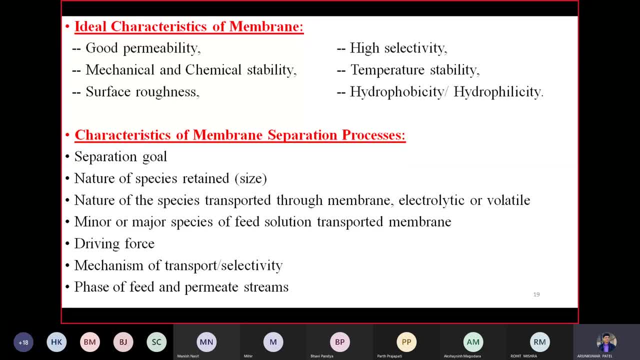 Next slide, please, Okay, Okay, Thanks. mean that process, which are the characteristics so we have to decide our separation goal. nature of the space is written. i mean on which basis we can select that processes, so which are the spaces which we have to retain. nature of the space is transport through membrane. 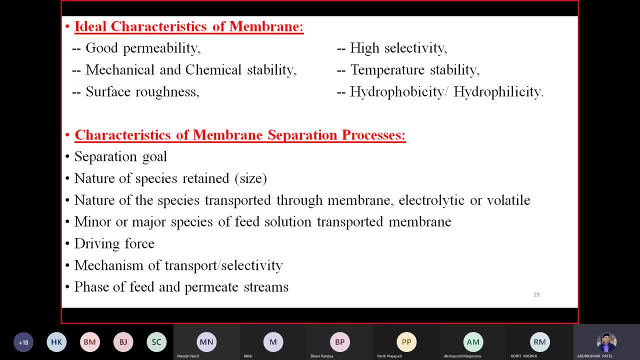 electrolytic or volatile, and based on that also, we will select that technology, which we will have to utilize, minor and major spaces of the field. solution, solution transported membrane. moreover, that which will be the driving force, we will select a mechanism of transport, selectivity, by which mechanism we can do the transportation of that field to permeate side phase of the feed. 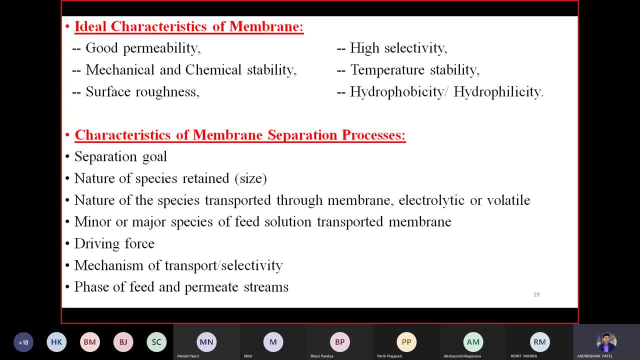 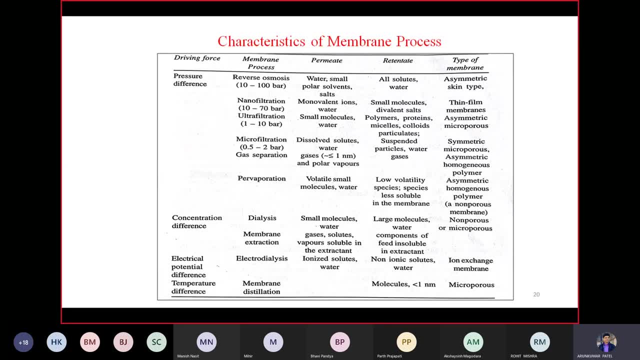 and permeate stream. i mean either it will be a vaporized or it will be a liquid form, or that phases also matter a lot for the selecting of that membrane processes. over here you can see some statistics. data is given. suppose driving force will be pressure difference and reverse osmosis we are adopting, then that process which we are utilizing will. 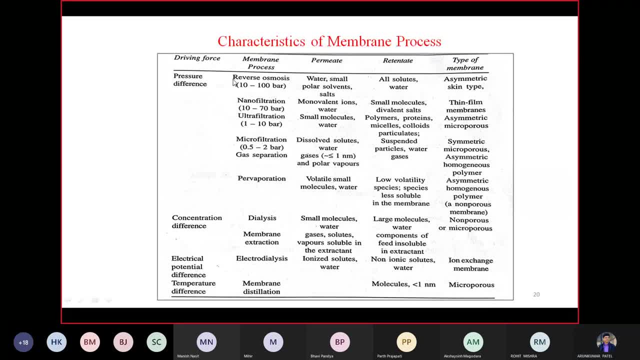 be 10 to 100 bar in case of pressure that reverse osmosis, but in case of nano filtration it will be 10 to 70, ultra filtration 1 to 10 and micro filtration 0.5 to 2, over here and whichever. 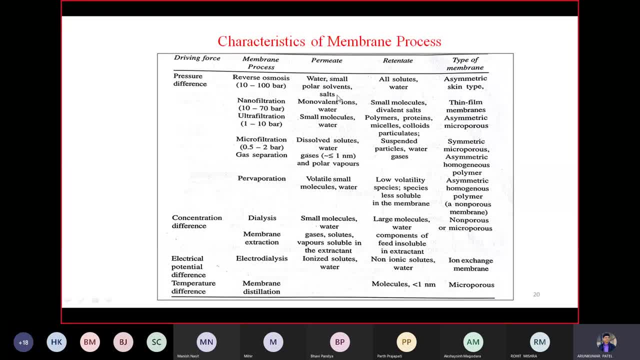 way we simplyery the process by which it across sample, by every single process that either process through prayed various test. so above the excesses it has preation using with forward souffle. vibration is a fixation zone in goshawk functionality inside the placement cozy. 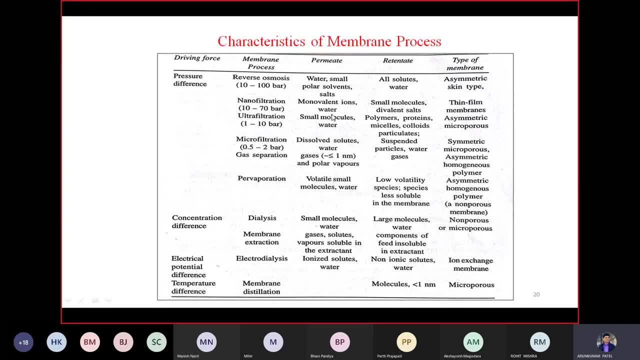 flammable right. you will get this process: water, small caller solvent shot right. that will be obtained as a monovalent and water molecules, small molecules and divalent salt that will be retinted and it will be permeated. In that case, thin film membrane, thin film composite, which is having 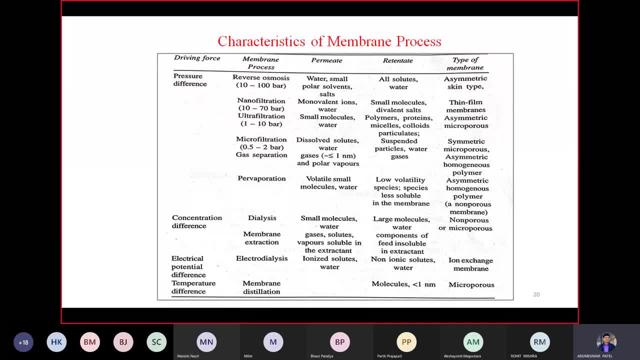 active surface layer as well as supporting layer, that kind of thin film membrane generally we are utilizing over here. So I will also share one- I mean my experience- to you right now as I come to know about that thin film composite membrane. Right now we know that we have that thin various 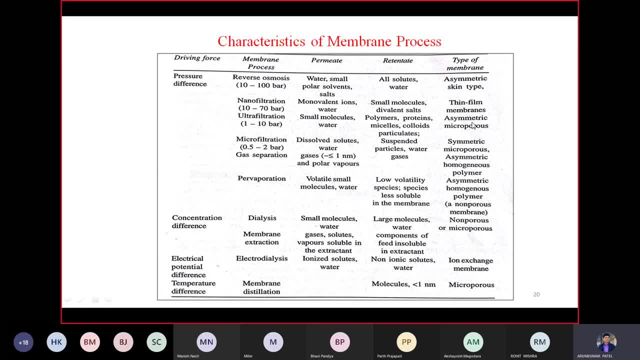 membrane modules which is readily available for the domestic applications. In that case I am right now doing that, some membrane driven processes I mean I am utilizing that concept of that membrane separation processes in my research work also. So what I have done 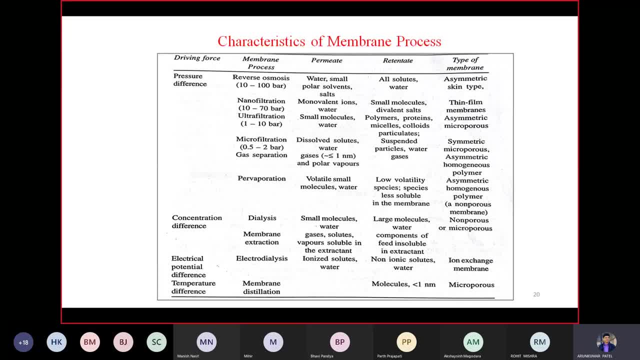 so I come to know that I mean kind of membrane which is easily available in market. I have just gone through that membrane I have purchased of approximate for I mean 500 rupees and I have just come to know whether it is working or not. So for the checking purpose I have just broken. 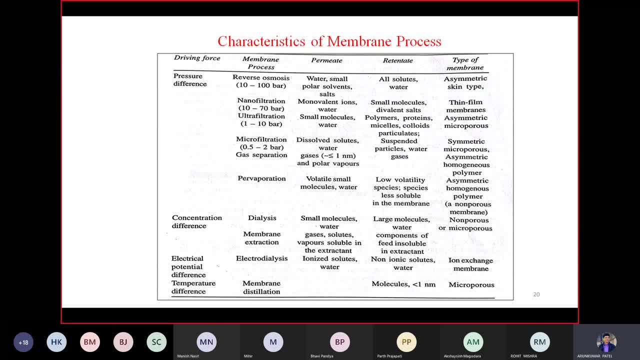 it and tested in a plate and frame module. So whenever I come to know it is absolutely, I mean active participant in participation in the separation purpose. So I come to know that with the membrane which is available in market it does not have that active layer, active surface. 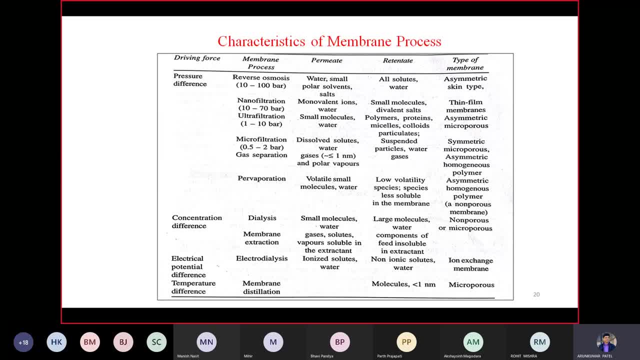 Only that membrane which we are, I mean I have utilized that was only have a supporting layer. So means that active layer which must have to retain that particles- I mean retentate it- will not, I mean- work properly. So just I come to know that, whichever local vendor they are, I mean 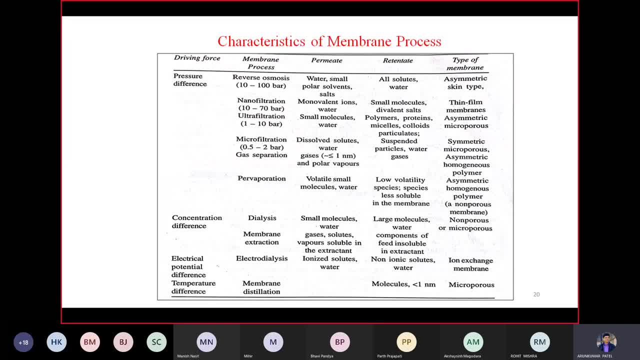 fabricating or preparing that kind of membrane. they do not have that active surface layer, which is actually costly, And this way I mean what I want to share with you. we are misguiding in certain cases, So that active layer, which is requirement for the separation purpose, which was missing in 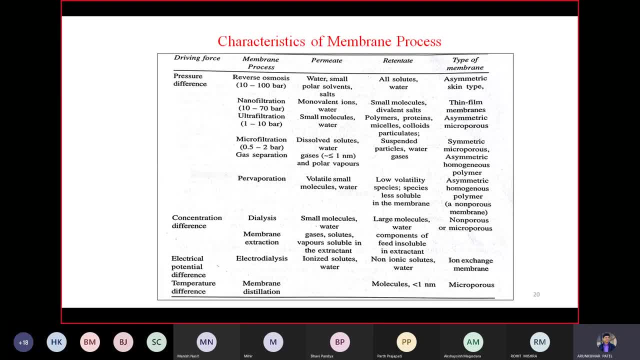 that case. So be careful about that also, because we only know that physical appearance of that module, or you can say membrane, cartilage in simple term, But it is in certain cases it is not that much actively separate that our desired separation. So this kind of things also happen with us also, So be careful for that. So just incidents which I have just 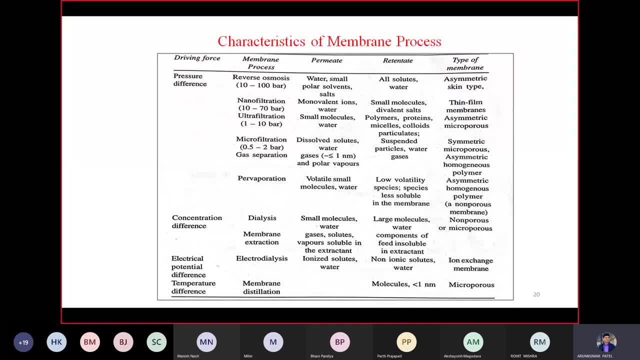 practically, I mean done and exposed to that kind of activities. So that is why, just I am, Joseph K, sharing with you. So it happens in that kind of structures also. Now, ultrafiltration, small molecules, you just go, you have seen, I think in these 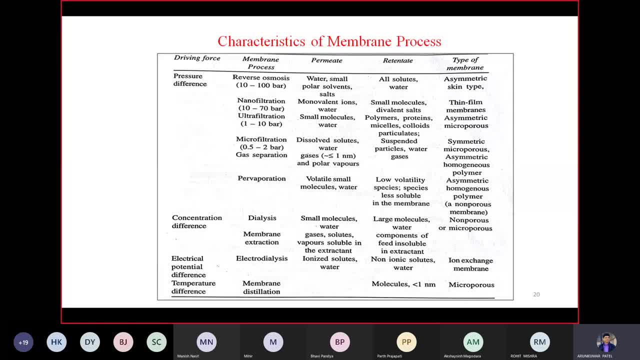 So we have the different permeate and retentate and type of membrane which we are utilizing, which includes symmetric, micro porous, asymmetric and other. also Over here per evaporation- you can see females Theater- volatile, small molecules and water permeation is a problem. 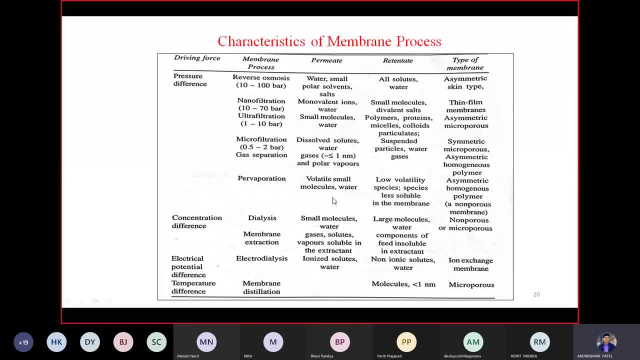 So overall chimprops dürfen sketches cannot be interviewed. yeah, That you know that is bother. Yeah, But it is very important to be sure which is not a İns requiring individual numerator, which is why you have a different function to tab mal perfection or similar to Carlo Re wedding. 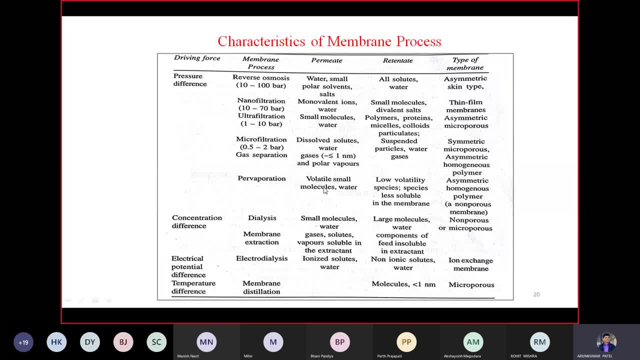 Yeah, It is tiny, Sorry- process by in which we can volatile that field solution and only vapour will pass through that membrane pore and at the other end we are applying that vacuum. and by application of that vacuum we are doing that suction of that permeate vapour, or you can say based. 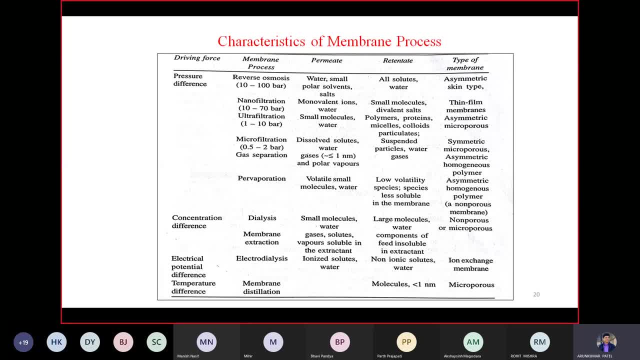 on the partial pressure difference, that because of that higher vapour pressure that will be passed through that membrane pore and ultimately we are getting that desired product, that first membrane, Based on that concentration difference, that dialysis, in case of that also, small molecules and water, it will be permeate. and large molecule and water it will be retented, but it will. 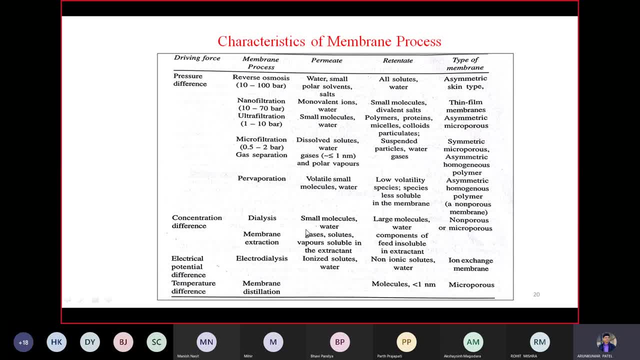 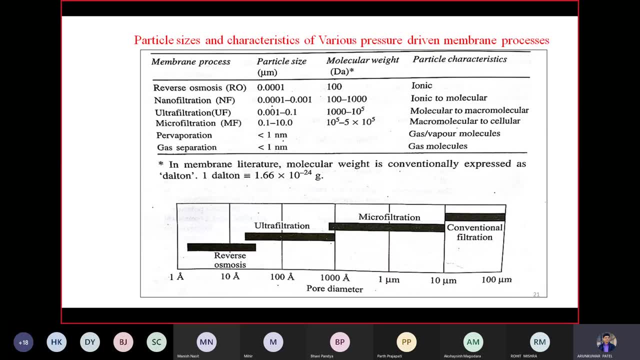 be a non-porous or micro porous membrane. These are the various characteristics and various parameters which we must have to come into mind. Over here you can say particle size and characteristics of various pressure pressure driven membrane. we have already gone through this Also: urethrosmosis particle characteristics. 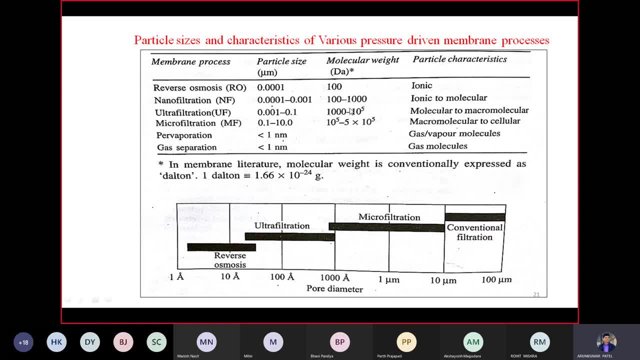 it will be ionic molecular weight, Dalton 100 to 5 over here. molecular weight cut off. one more term will be there: molecular weight cut off. whenever we are doing that separation mechanism by which we are separating So the particle which will be retain on the surface, 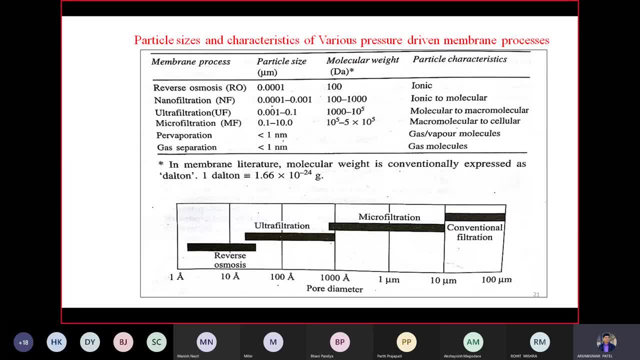 of that membrane separation. if we have that smallest particle size, if we have that smallest size, If that particle size almost 90% of, or you can say 80 to 90% of that smallest particle size, particle, if we are retaining over the surface of that membrane, that membrane, then 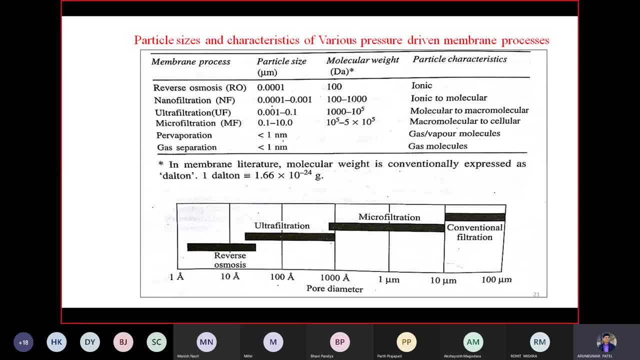 that size of that particular particle we are calling as molecular weight cut off. So this we are showing in terms of Dalton. So over here you can see the size of that particular particle. Over here you can see similar pore diameter. over here, and with that various 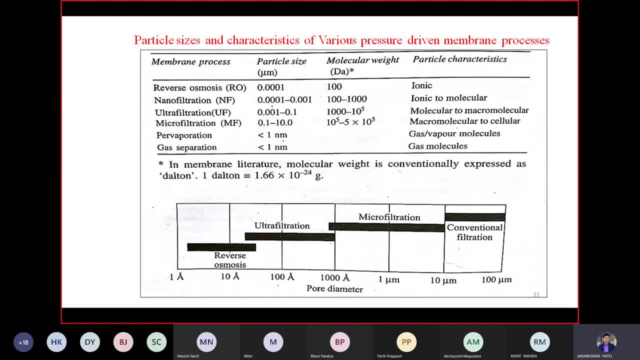 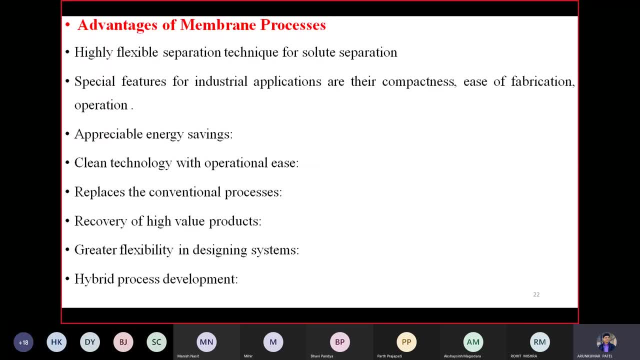 processes by which that working on that particular pore diameter over here in sagenstrom Now we will see about that various advantages of that membrane separation processes. So it is highly flexible. separation techniques for solute separation. spatial features for industrial application: 0.. peer parcel per packet per political Indonesia where you can find that sample puede ficar. 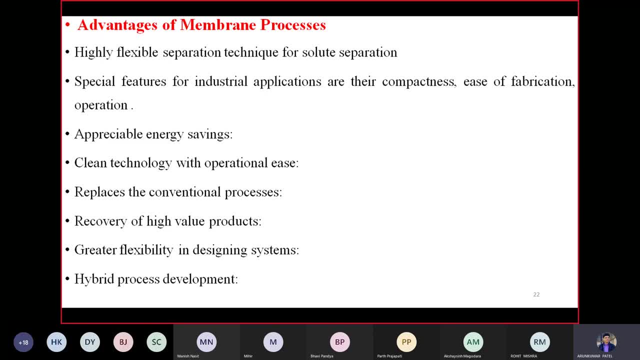 and their compactness, is your fabrication operation appreciable energy saving. right now this is the most advantageous feature. or you can say: uh, energy saving operation and because of that, uh, that only we are moving towards that membrane separation techniques. uh, by proper application of that proper method and proper membrane material we can save too much. or you can say huge energy. 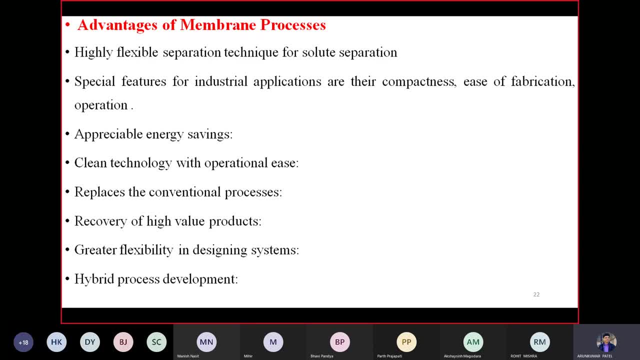 uh by selecting the proper method clean, moreover, that it is clean technology with operational easy. now we are familiar with that zero liquid discharge technology also. so with that application of primary, secondary and tertiary treatment processes, we can do that kind of clean technology with operational easy and we can uh run that kind of uh zero, zero liquid discharge plant also. 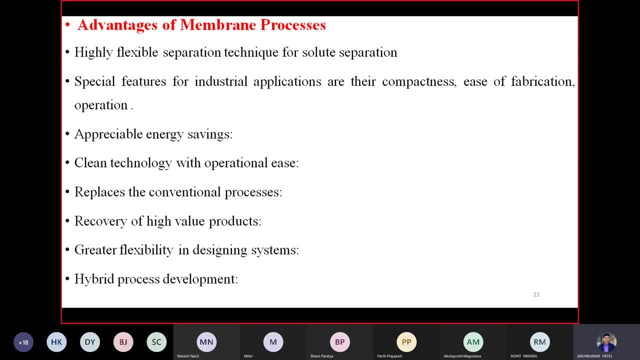 uh, moreover, that uh, once that separation, i mean membrane- processes come into existence, we are regularly replacing that conventional processes also. right, even, even even in uh uh, some study, i'm going, i'm right now going through it- i'm also replacing that conventional crystallization process yesterday. 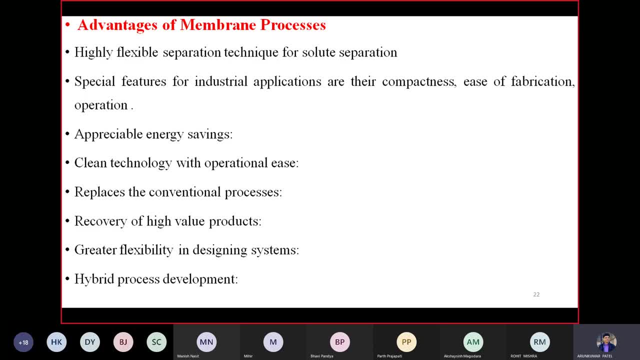 uh that dr sr patel sir was there and he has explained that the various crystallization method is integration with other tech, i mean other processes, which is also process intensification. in my case i am clubbing that. i mean uh, forward osmosis and reverse osmosis with that conventional 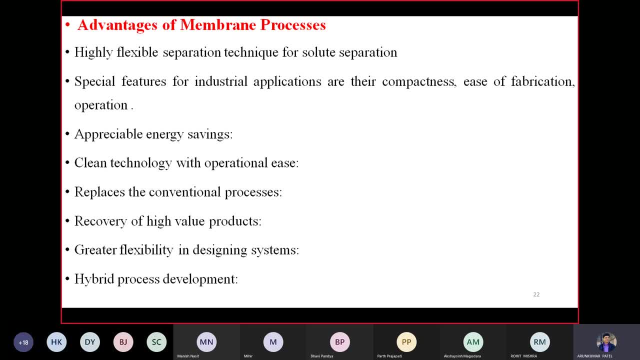 evaporation method, so kind of that feed material which you have chosen, if it will be work with that kind of separation mechanism so that we can easily uh dewatering that, whichever solvent we have to dewater, i mean uh separate out and we can easily achieve that super saturation and after 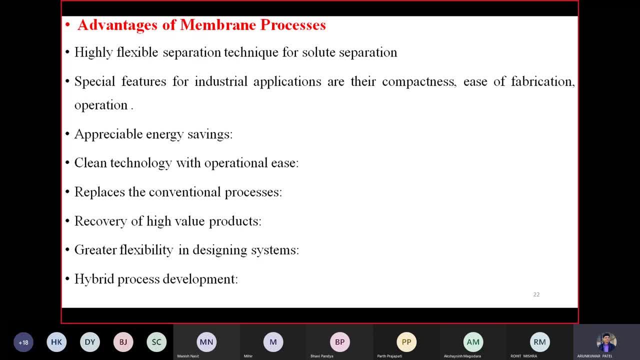 once that super saturation will be achieved, we will uh move beyond that equilibrium cow. and once that metastable zone width will be achieved, after that, uh there will be a- i mean kind of beyond that super saturation, i mean nuclei will be formation and crystallization beyond that. 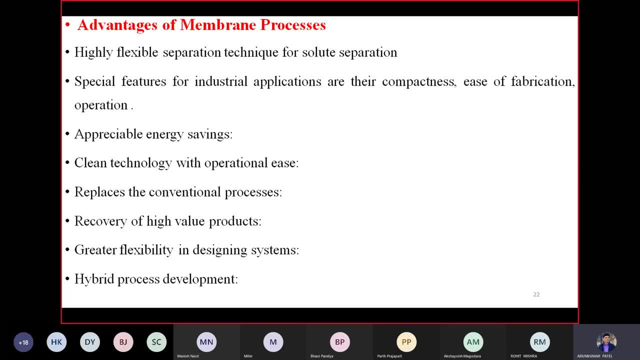 super saturation uh limit, there will be a start of crystallization process. so to remove that much uh material, um, we are using uh. we are utilizing uh, this kind of membrane technology also, so that we can easily and by only applying small amount of pressure energy instead of that much heat energy. 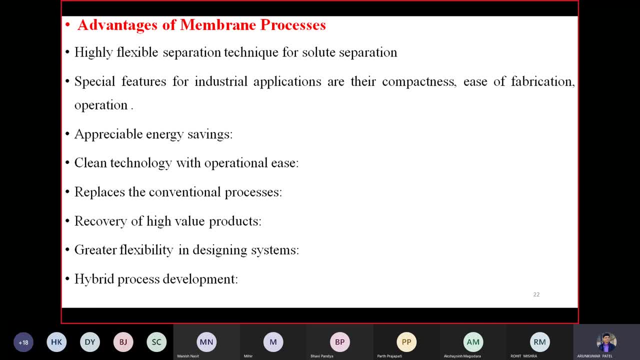 we can take advantage of energy saving. uh, this way also you can go right, moreover, that high recovery of value products in some cases, and especially in case of that pharmaceutical industry, some valuable products which may be heat sensitive also, so conventional method, which is not feasible. that much for that separation. in that case also you can go for the recovery, this kind of. 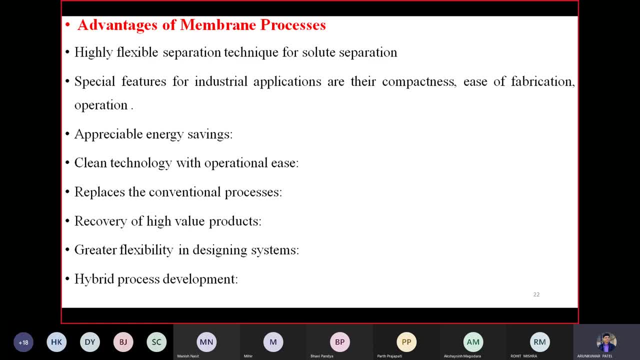 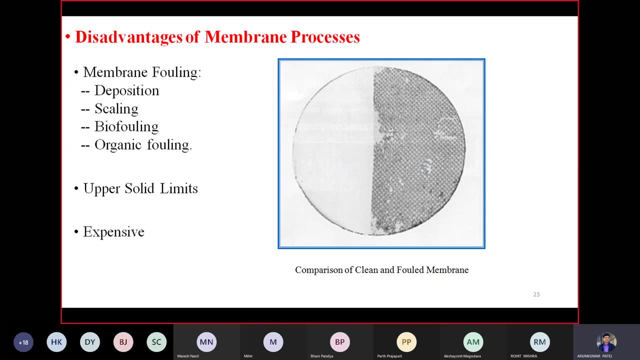 membership separation process also greater flexibility in designing system. you can change according to your requirement and, moreover, that it you can develop that hybrid process development also. but, as we know, once it has a certain advantages, it must have a certain disadvantages also, right, because then when we are talking about that membrane technology, it 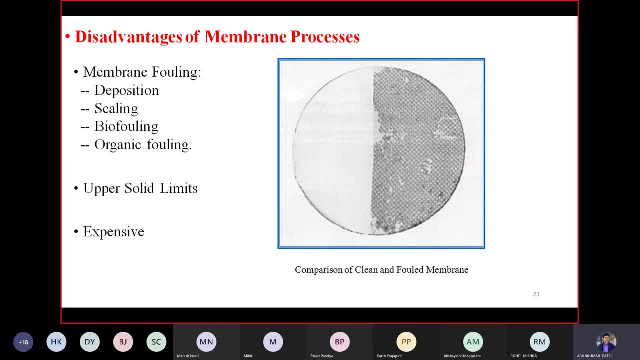 is not a kind of simple or conventional technology, because once that installation, we are planning to install it in a commercial scale or you can say at any scale- it requires too much cost. we know, uh, as we know, that simple filter, filter which, which is available in market, it is too much costly. but if you go for that membrane, or you can say membrane cartridge, 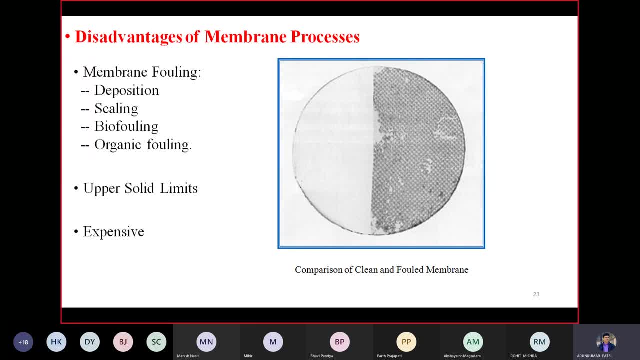 it is comparatively too much high cost, moreover, that it is not regularly i mean cleanable or replaceable or washable it it it is too much, costly as well as uh, it should have a certain drawback also. so, uh, based on that, it is costly as well as it should have a certain disadvantages, which includes: 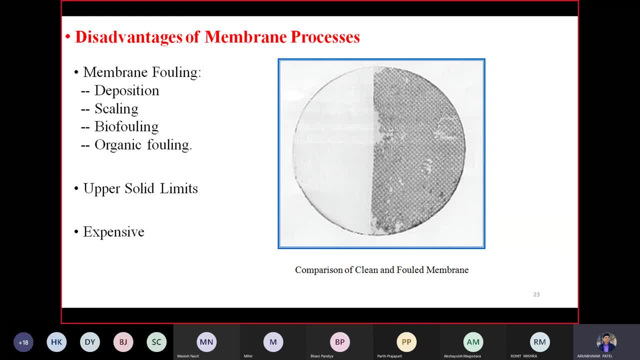 that membrane falling, deposition, which includes deposition of that particle, scaling of that particle, bio falling, some bacterial growth, or you can say algae growth, will be there because, uh, moreover, that organic falling also, so that this way that membrane falling will be happened, moreover, that there will be upper solid limit and expensive. 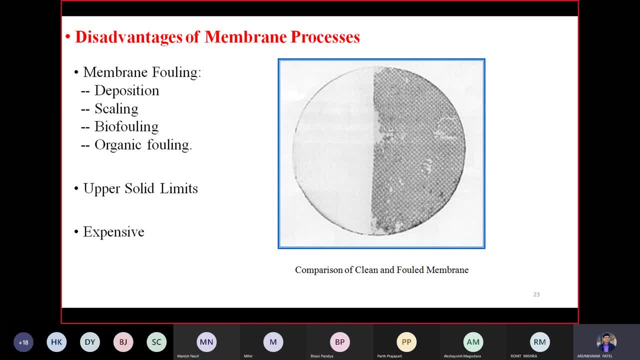 what i mean to say over here. once you are starting your that separation processes, uh, at the very early stage of that filtration we might have gone through that filtration also, we might have conducting regular lecture in case of that pressure. i mean constant rate filtration, constant pressure filtration. in one case we are increasing gradually pressure and we are 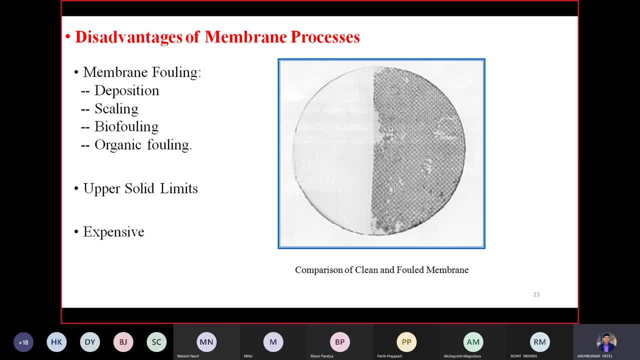 obtaining constant rate. but in other case, if we are maintaining constant rate- i mean constant uh pressure- then rate, obviously rate will be decreased similarly over here also because because of that falling and upper solid limit, gradually that deposition of that solid particles will be there over the surface of that membrane and because of that there will be a kind of 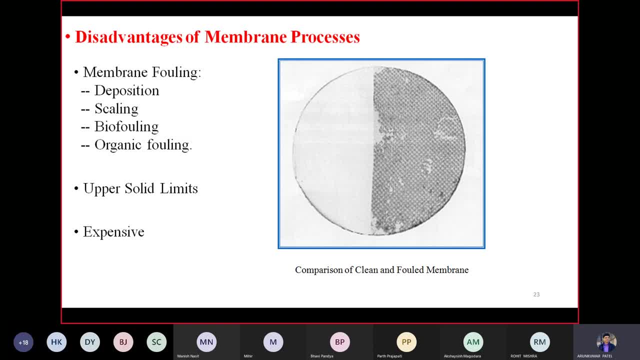 concentration polarization will be taking place means concentration. polarization is term which come into picture where certain regions on that membrane surfaces there will be concentration on, will be a too much high quantity of that particles that will be deposited and that kind of phenomena, so that there will be a no proper permeation will be taking place and that kind of regions. 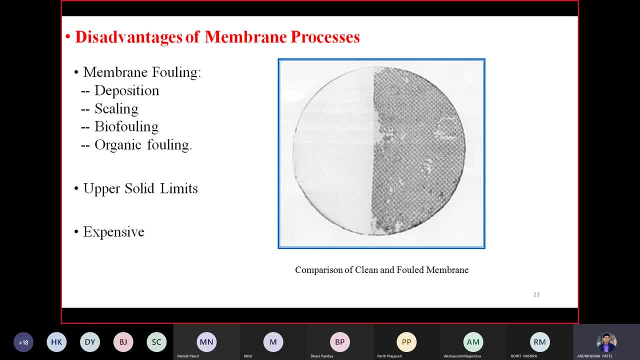 that will be happen on the surface of that membrane and we are calling it, that is, concentration. polarizers means in certain regions there will be a deposition of certain particles in a too much amount, in a huge quantity, so that there will be no further permission or there will be a difficulty in permeation process. so this kind of phenomena, 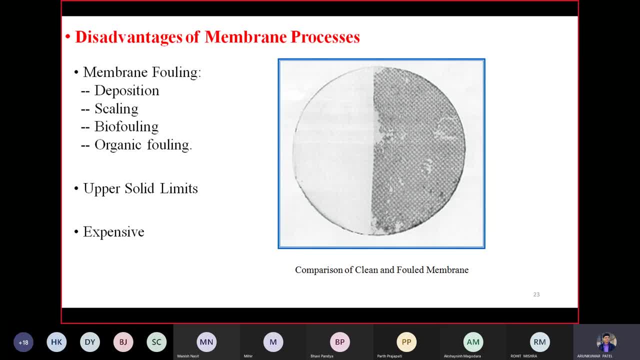 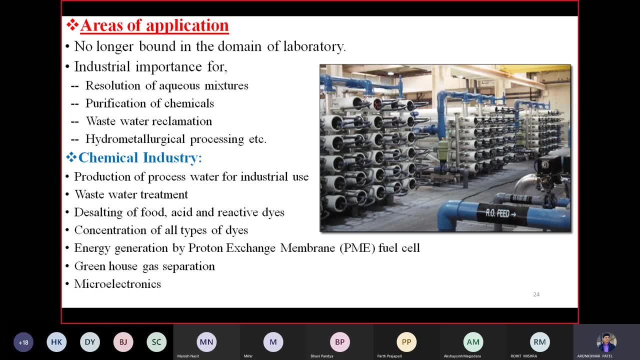 will occur and which is leads towards the upper solid limit, and, moreover, that it has advantage that it is too much costly that we must have to accept. you can see over here how that we can assemble that various- i mean module, of that various membranes and accordingly we can. 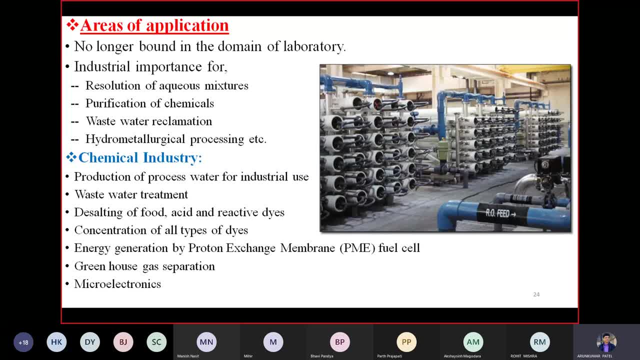 assume that goal of separation, area of application which includes it is not related to only laboratory scale but, as well as its industrial importance, includes resolution of a solution, purification of chemicals, wastewater reclamation, hydrological processing, also in chemical industry, wastewater treatment, production of water and industrial use resulting of food acid and reactive dyes. concentration of all types of dye. 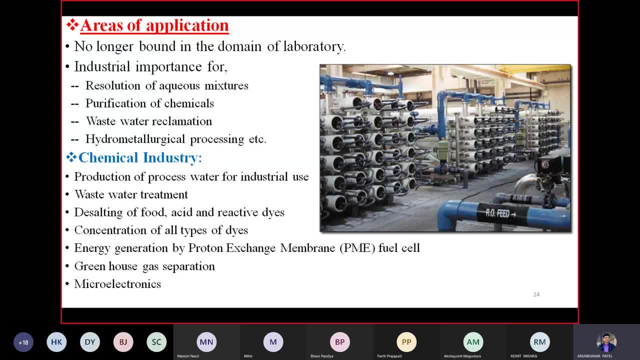 captured. so this all kinds of processes are owned, are being done on aver increasing benefits during period of time where there are a very high literature around how this integration process can also be done. so if there is a sit cancel or energy exchange, the energy generation process, important that in mixing differentOY. 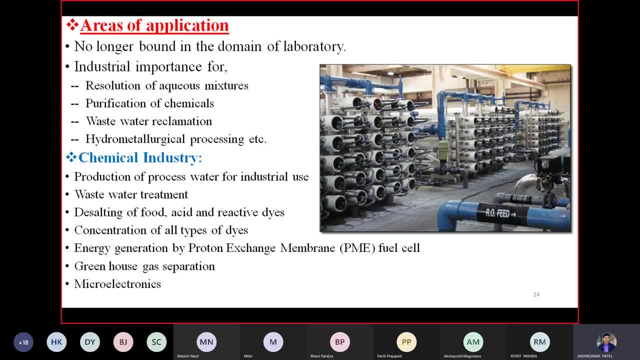 energy generation by PM. it is also one of the emerging trend of that protein exchange membrane fuel cell where we are right now using that membrane, the electrolyte. so it will be selectively allow certain- I mean charge- particle through it and it will be written in electrolytes. generally we have that positive and negative. but in case of that protein exchange membrane fuel cell, that membrane itself we have and it will be selectively. 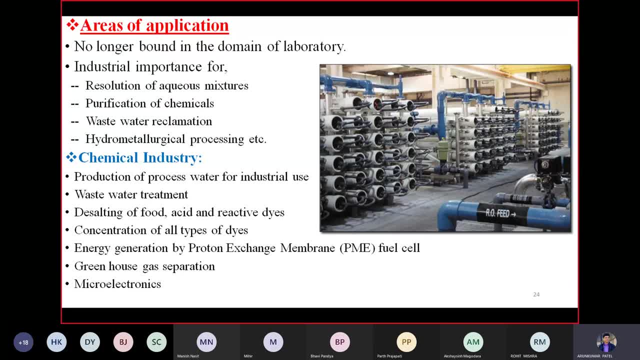 selectively allow that charged particle in a feasible way so that there will be a kind of- I mean power- current generation will be taking place, Greenhouse gases separation will be there, microelectronics in that, all chemical. in cases in chemical industry we are utilizing pharmaceutical also, as I said, because it is the one of the 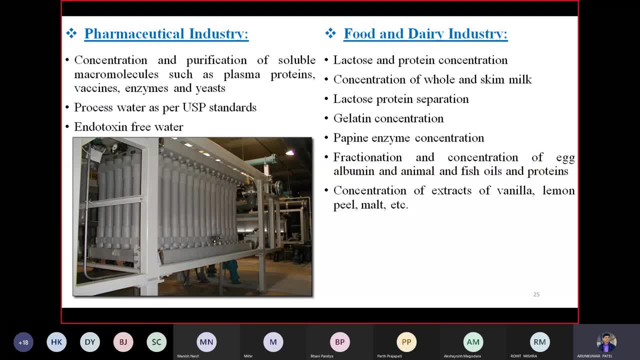 too much. we can say sensitive, I mean sensitive area or industry where we will must have to take care about that product. or you can say API, or you can say formulation of the drug. we are carried out because this drug required too much purity. Even my guide that, Dr SR Patel, also mentioned that in case of that crystallization we must 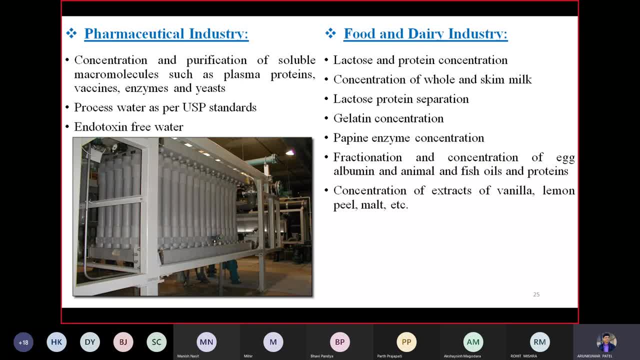 have to take care so that, whichever That crystal we are making, it must be in a purified form, it must be in a certain crystal structure, it must be in a certain crystal morphology, so that accordingly, because in pharmaceutical industry, whenever we are doing this kind of processes, 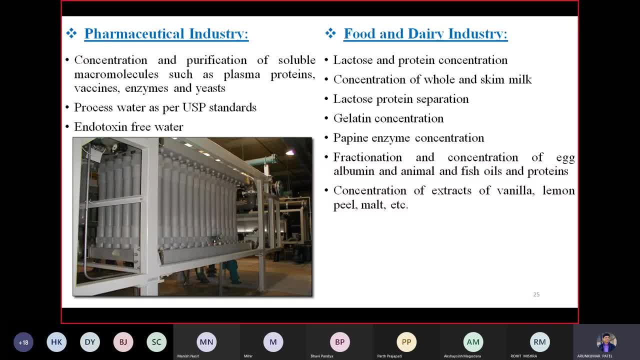 So in that case there are certain properties which must required in crystal. So yesterday you have just gone through that bioavailability dissolution rate, that terminology in which There are. There is one more terminology which we are calling as compressibility. So we must have to make crystal in a such a way that, whichever crystal we are getting, 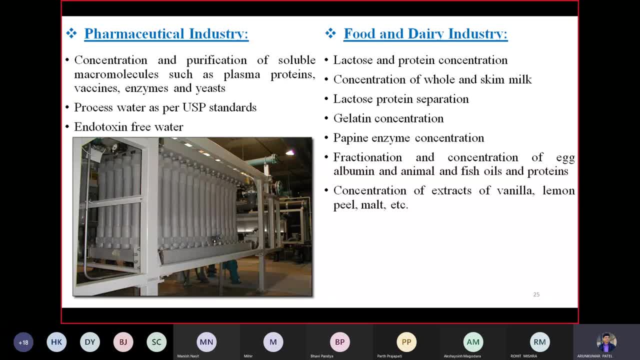 in the form of API active pharmaceutical ingredients, which must be having certain crystal structure so that compressibility will be done properly and tablet we can generate that proper. I mean compress the tablet proper and it will be dissolved in a specific time interval as per our design dissolution rate also. 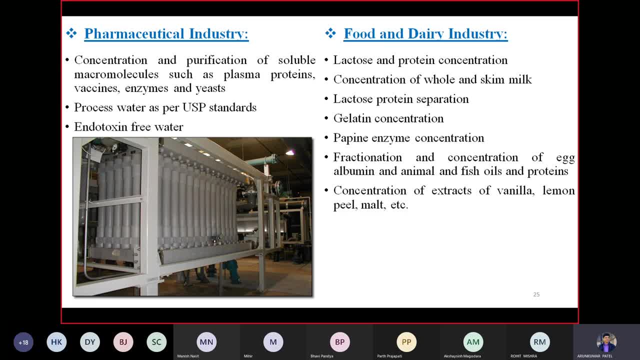 So that time permits, I will discuss in depth in that particular topic also on which I am working. So I have not included in my presentation because it is right now in, I mean, publication process. That is why I have not included that content in my today's presentation. but in situation. 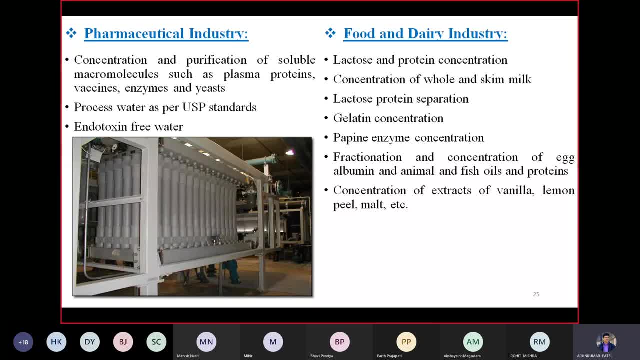 permits, I will discuss with that also. Okay, So pharmaceutically, that is why we are utilizing food and dairy industry. If you go in that, any dairy industry there is, starting from the milk to various its derivatives, or you can say various products starting from the. I mean you can say sumul, amul and other. 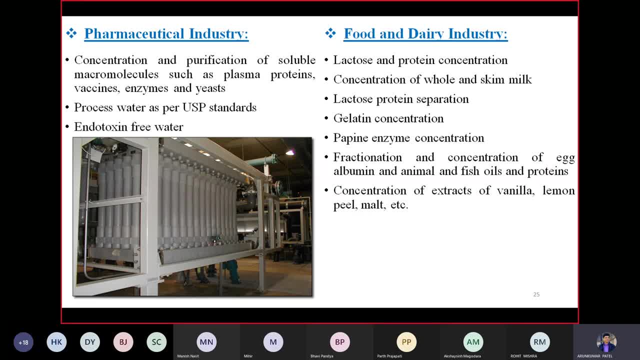 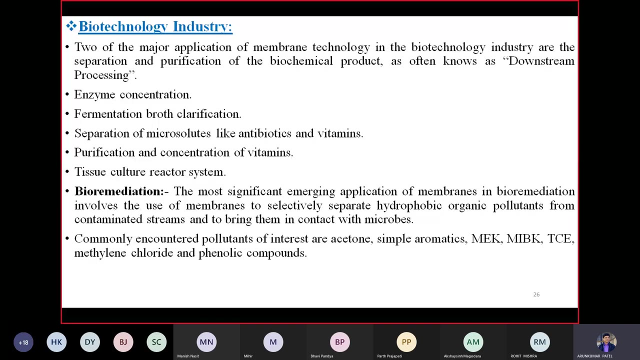 dairies. Wherever you go for visit you will find different, different that membrane separation technology only. So, apart from that only they are doing that separation of that various products right and they are preparing that various desirable products based on that separation. So, food and dairy industry, biotechnology industry, also enzyme concentration, fermentation. 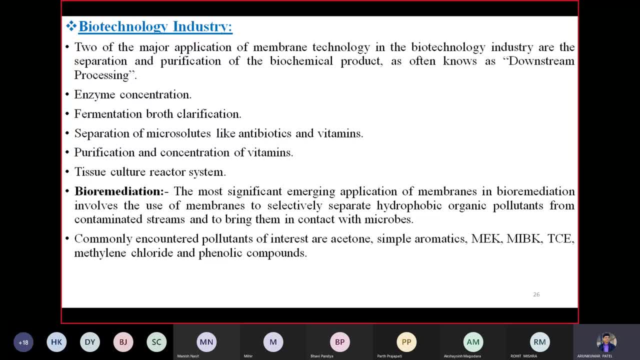 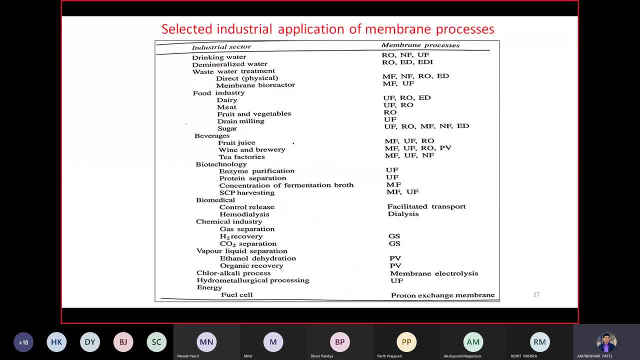 cross clarification. separation of micro solute like antibiotics and vitamins, purification and concentration of vitamin. I mean this is also applicable, right So over here. industrial application: whenever you have that, various industrial sectors which, in starting from the drinking water or you can say waste water treatment plant, we can. 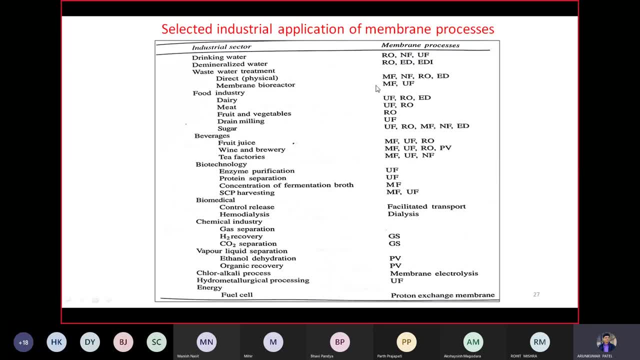 utilize RO, NF, UF right in certain cases for the matter. I mean heavy metal and other metal removal also from the waste treatment. We can go for ED and EDI. also direct physical biomembrane, bioreactor, food industry, in which also UFR, RO and ED, beverages and juice from where we can, we can do that concentration. 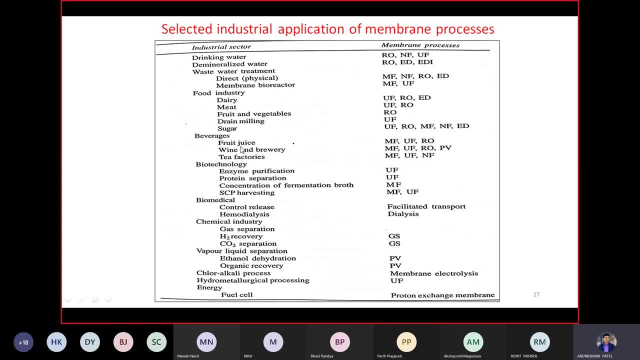 of that particular juice. You might have familiar that in fruit juice concentration in sugar industry what we are doing, We are doing that evaporation only. We are evaporating in that sugar can. whichever juice we are extract, I mean extracting from that sugar can. 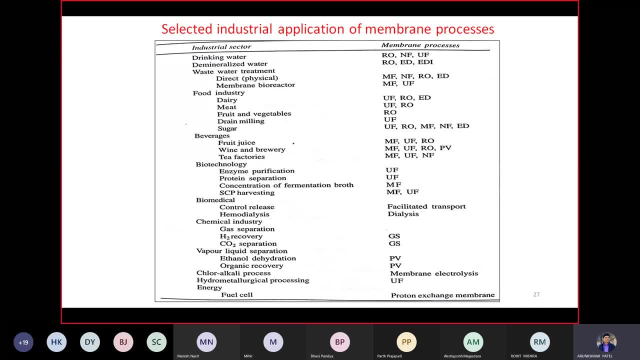 That contains only 5 to 10 percentage of that sucrose. remaining that will be water only. So in our sugar industry we all have must visited and we are familiar with that. there will be a kind of stages in which we are doing evaporation: first evaporator, second evaporator. 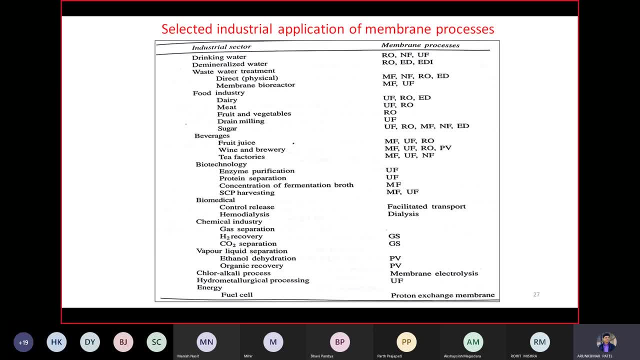 third, evaporator. I mean 40 percentage concentration, 60 percentage concentration, various stages and huge amount of that energy we are wasting for the evaporation. instead of that, if we are utilizing this kind of separation technology- MF, UF or RO- in that case also you can separate out that I mean. 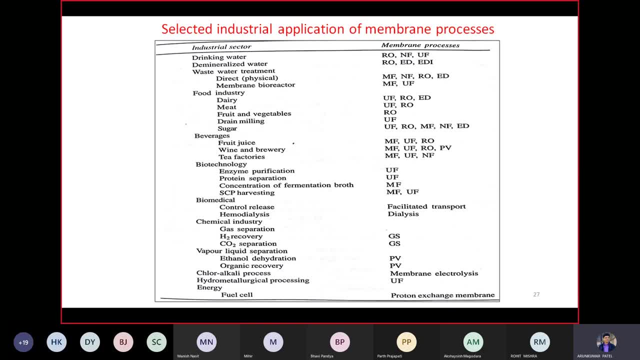 water component as a separate and you can retain. it may be possible that retain it may be your product or permeate may be your product, based on your product requirement. it may be possible, in case of that concentration, you can get that water as a permeate and that 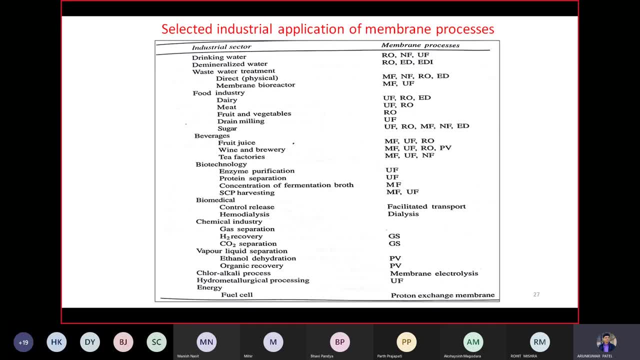 whichever other component that will be remain as a retentate. So it may be possible: permeate will be your product, retentate will be your product. but you can utilize or you can club this kind of technology and you can utilize it In biotechnology also: enzymic purification, protein separation, concentration of fermentation. 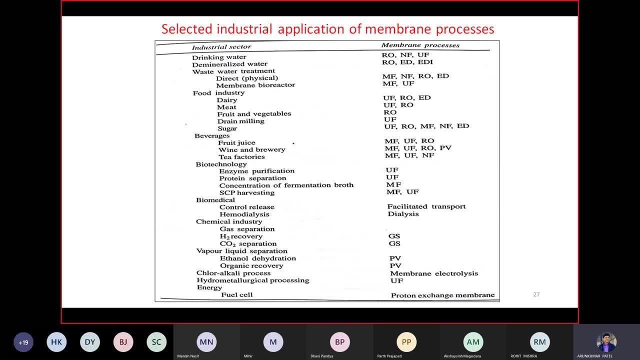 growth and other. So I have not that much concentrated with that enzymic purification and other technology So I will not explain you this stage in that way. But these are the applications in various industrial sector and various membrane processes which we are adapting Over. here you can say vapor, liquid separation, ethanol, dehydration per evaporation. 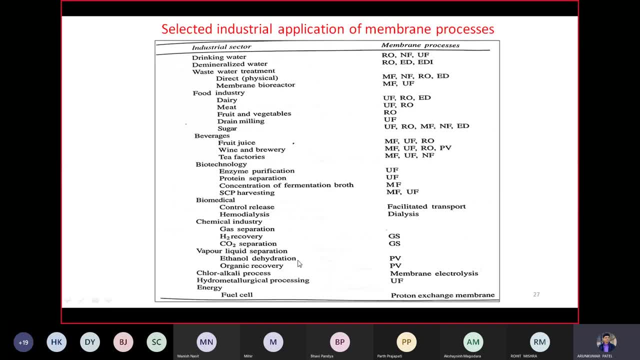 So, whenever that ethanol will be our requirement and dehydration- of that I mean water evaporation- we can achieve through that per evaporation process, which we are separating in the form of vapor, We are converting, By giving that high temperature, into a vaporized form and that vapor will be passed through. 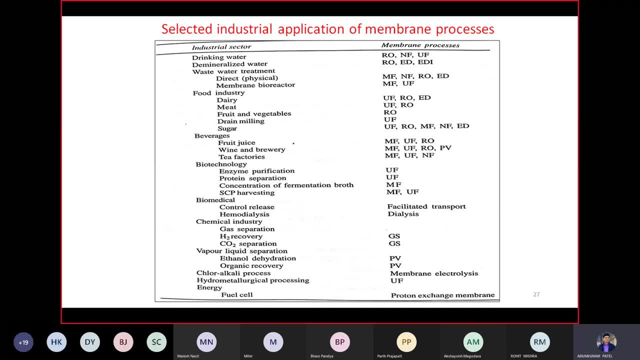 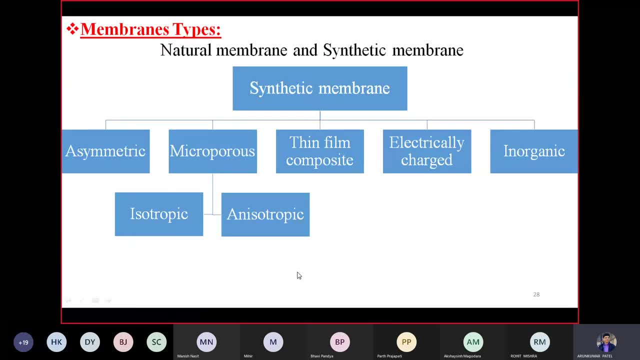 that pore and ultimately we can apply vacuum at the other end and we can separate out this. So these are the processes. Now we will come to that membrane types. So which are the different types of membrane which is we can utilize for the membrane technology? 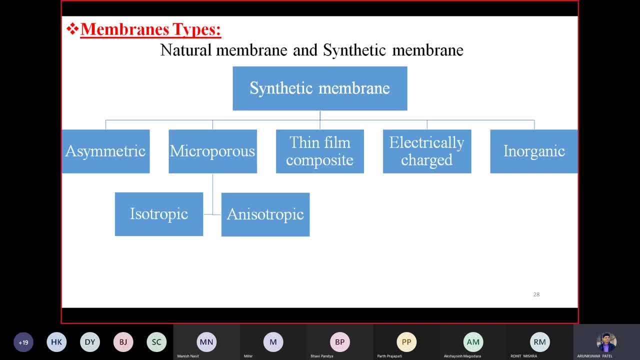 So generally there are so many membranes which is naturally available as a synthetic membrane. But in commercial scale we cannot depend on that naturally available membrane, So we must have to synthesize as per our requirement. So based on that synthetic membrane we can classify the asymmetric membrane microporous. 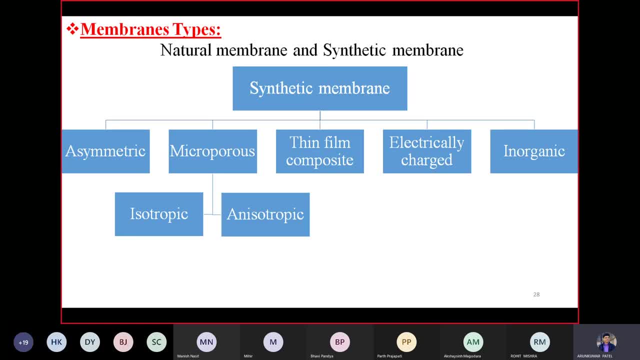 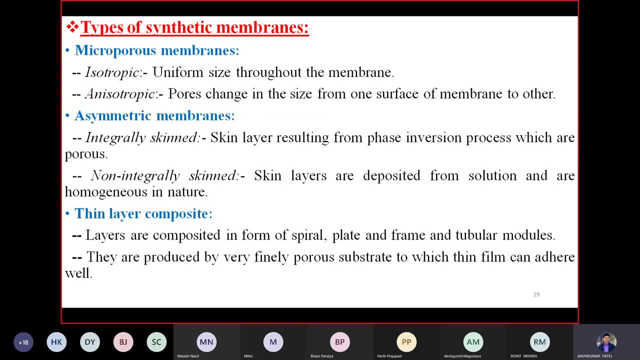 membrane. moreover, the thin film composite membrane, electrically charged membrane, inorganic membrane, microporous, further classified into isotropic and anisotropic, based on its characteristics. we can classify So: micro porous, uniform size throughout the membrane on that membrane surface. anisotropic pore size: pore changes in the size from one surface. 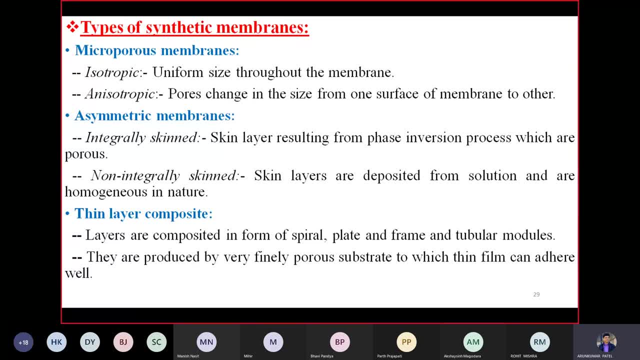 of the membrane to other. that means there will be a kind of change in that different, different layers which we are applying on that membrane in this way. moreover, that asymmetric membrane integrally skin and non, So it is a whole term which is related to that characteristics. 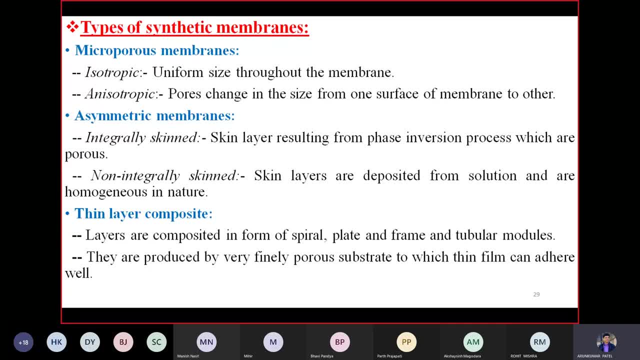 of that: membrane surfaces and pore size. We are playing with that pore size and ultimately we are developing this kind of synthetic membrane right: thin layer, composite membrane, which is having multiple layers right. So these are the various types of membrane by which we can maintain that pore size and we are utilizing over here right So electrically. 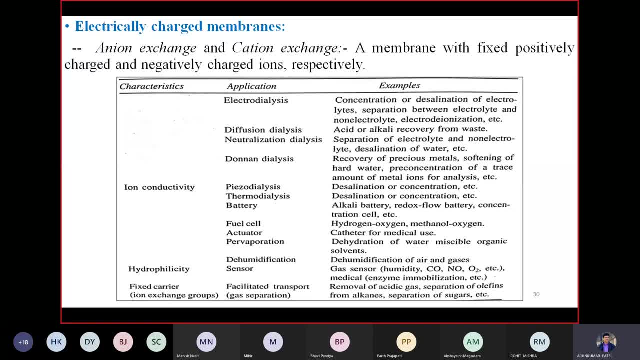 charged membrane, also anion exchange and anion exchange, Then cation exchange membranes. that separation process will be taking place based on that charged anion and cation and based on that we can stuck up certain particles on that charged particle on specific ionic charge and this way we can separate out that various 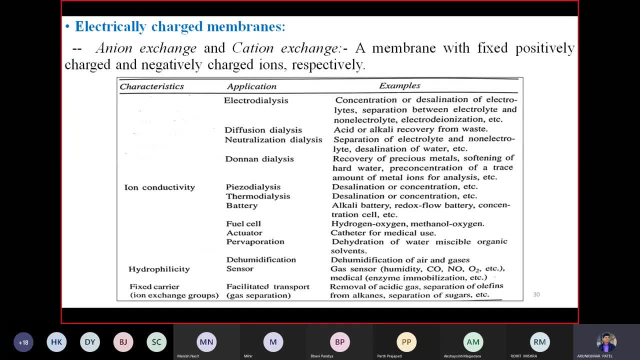 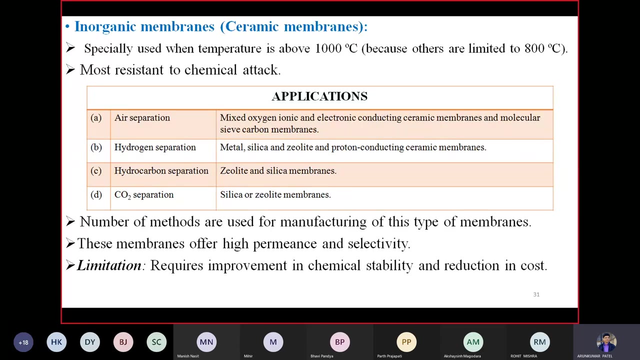 ions which is having specific charge right, and ionic conductivity will be there. So for dialysis and other processes which we are utilizing, for utilizing this electrically charged membrane and we can separate out that our spaces right Inorganic membrane, which is one of the type of special kind of membrane which we are utilizing. 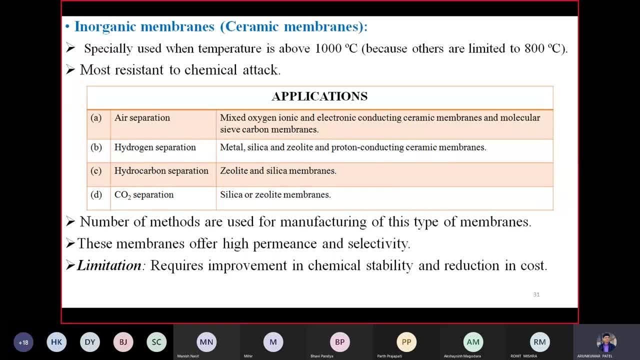 as a high temperature, because in our processes, as we know, we have certain limitations in membrane technology. we cannot go beyond certain temperature. But in case of certain cases, if we will have to go beyond that certain temperature limits, in that case we must have to choose that membrane. or you can say ceramic, ionic, inorganic membrane or, sorry, ceramic membranes. 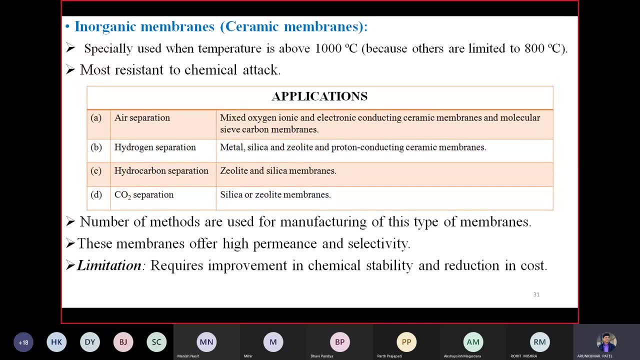 right, but it has characteristics most resistance to chemical attack. it right. So certain applications: air separation, hydrogen gas separation, hydrocarbon separation and CO2 separation- right, We are utilizing. these are the different types of membranes right, Metal, silica, zeolite or proton conducting ceramic membrane. These are the different. 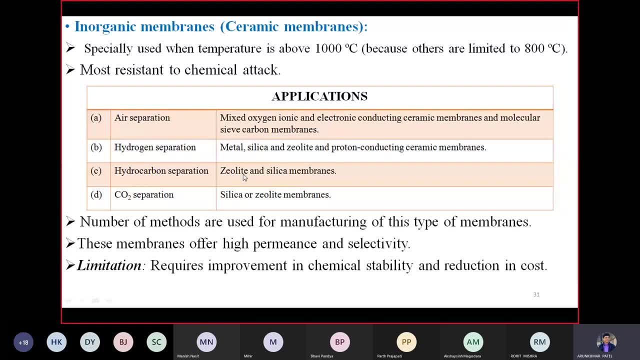 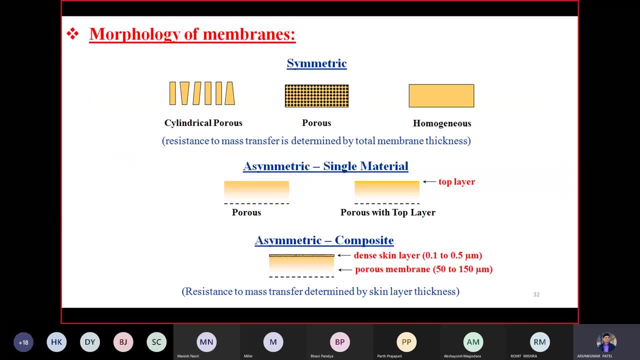 types of membrane which we are utilizing: zeolite and silica membrane. also silica and zeolite membrane sources which we are utilizing for the specific application of that various gases separation right. So this is about the ionic membrane, The structure which we have discussed. 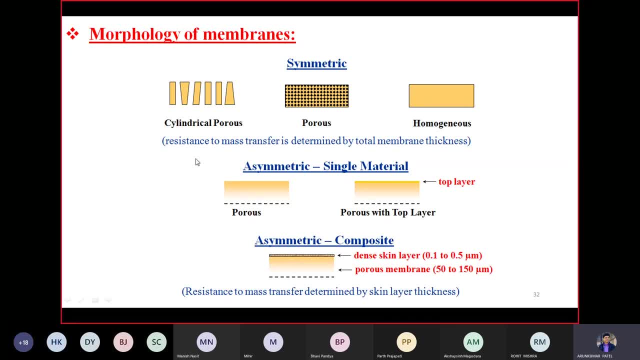 previously. that morphology which I have shown: cylindrical porous- porous, homogeneity, which we have discussed previously. that morphology which I have shown: cylindrical porous- porous. crystallised membrane, asymmetric single material. it will be a uniform. you can see over here it is a little bit top layer which is having a small pore size, which has been synthesized. 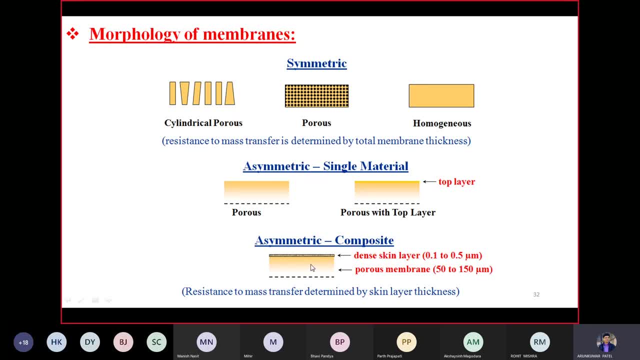 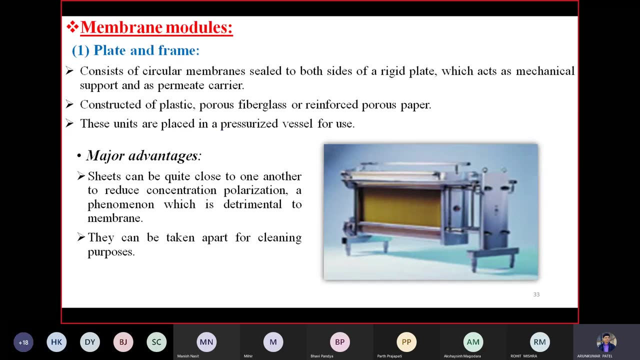 with that poly asymmetric membrane. It has a different three layers. This way we can have to ultimately play with that membrane technology. Ultimately, in our all cases, membrane will be hard for the separation. Whichever kind of membrane you are utilizing or you can synthesize, 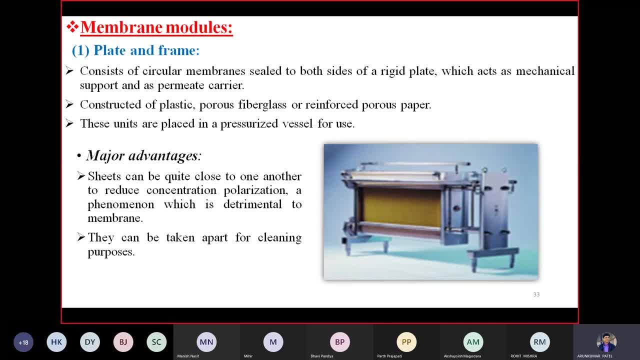 synthesized based on your application. you can use it for the various applications. So membrane will be heart of this whole processes. Once you are preparing, as per your desired requirement of the process, that particular membrane, after that you can achieve your goal. So these are the various modules which we are utilizing: plate and frame module, as we 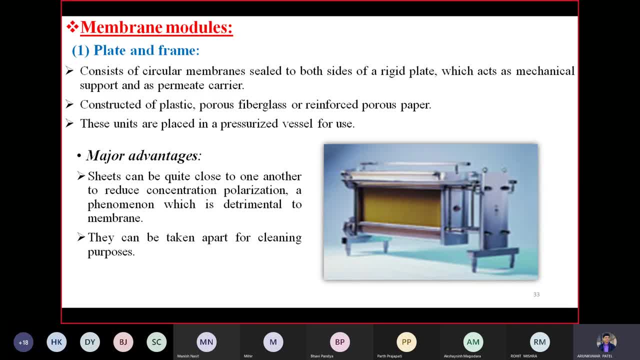 are familiar with that plate and frame module because ultimately, whenever we are selecting that various module, in that case surface area will be come into picture. So we can have to think about that, sorry. So, membrane modules. so we, sorry for interruption. So whenever we are, think about that membrane and its module. so, whichever membrane we are, 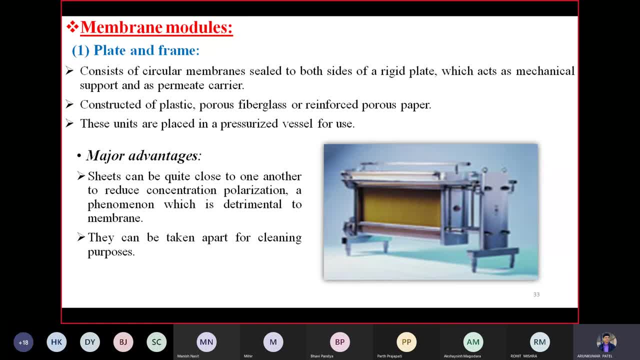 utilizing. so we must have to think about that surface area which we are providing for the separation purpose. As that surface area will be increased, then separation will be easy and that more permeation will be taking place and permeate flux we are getting more and more. 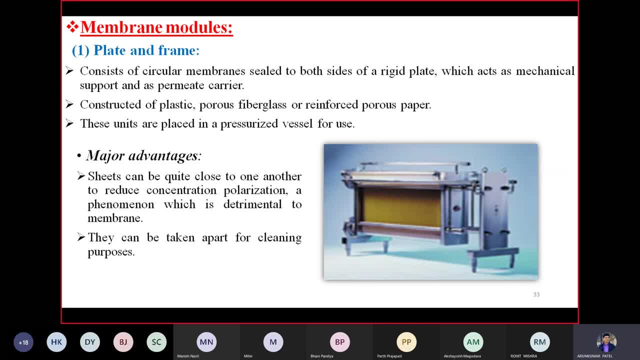 So based on that you can see plate and frame. it is kind of plate and frame filter. even that conventional filter place, Okay, This kind of structure in between that we are putting that membrane and taking advantage of that. also, seat can be quite close to one another to reduce the concentration, polarization. 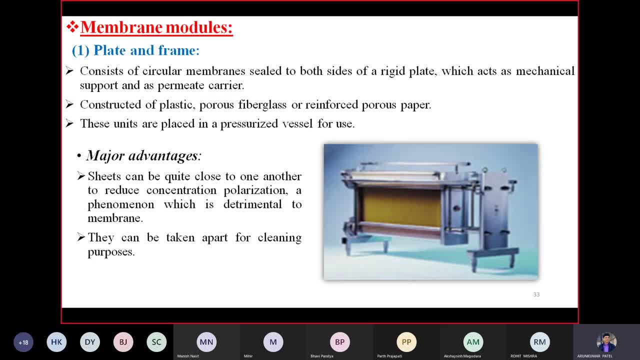 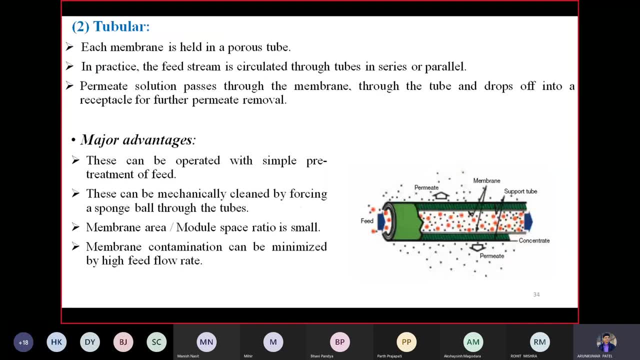 So we can avoid that concentration polarization by simple application of that plate and frame membrane module. So these are the plate and frame, apart from that tubular it is kind of simple heat exchanger. We are familiar with that silent tube heat exchanger. So over here we will see in the diagram also you can see feed material which will be passed. 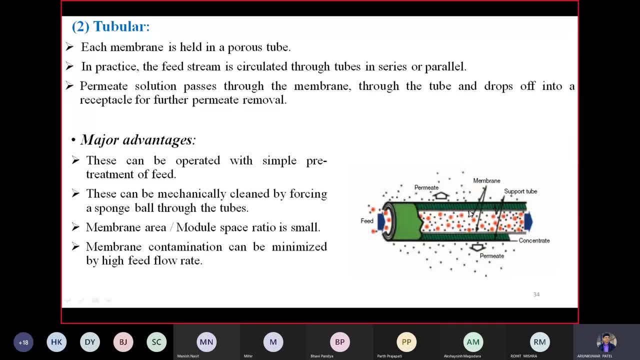 through that you can say kind of tube side in between that surface. we are keeping that membrane and at the other side, whichever permeate which we have to- I mean we have to pass through it- that will be passed through that membrane and ultimately we will get permeate from the 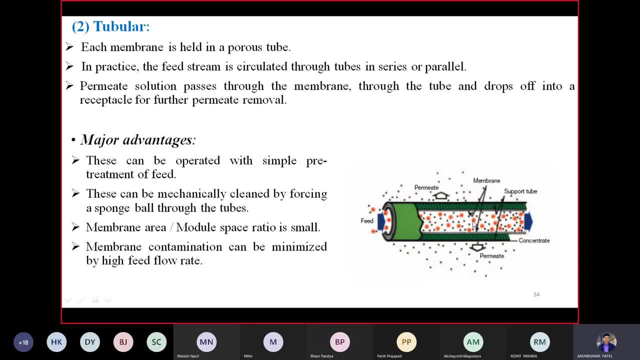 outer side And inner side that whichever feed or you can say concentrate, that will be retained. and to support this membrane we have to kept that support structure also. So this way that tube will be, we have like porous tube from which that permeate, only permeate, will be passed through that membrane surfaces to tube, to cell side and the remaining 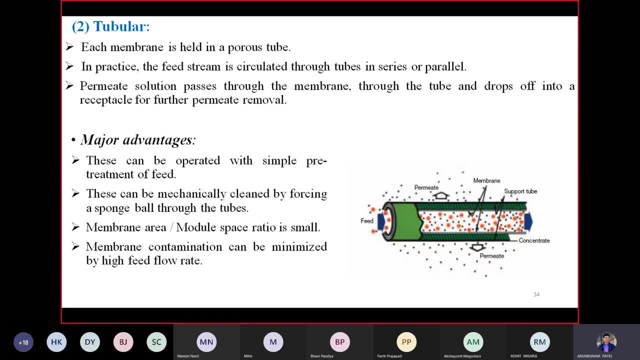 that retentance will be remain as it is inside of the tube And it will be flow, Okay, Okay. So what happens? So the tube will have that main membrane. it will flow towards that cell side that permeate. It is similar will be happen through in case of that membrane reactor also. that also we. 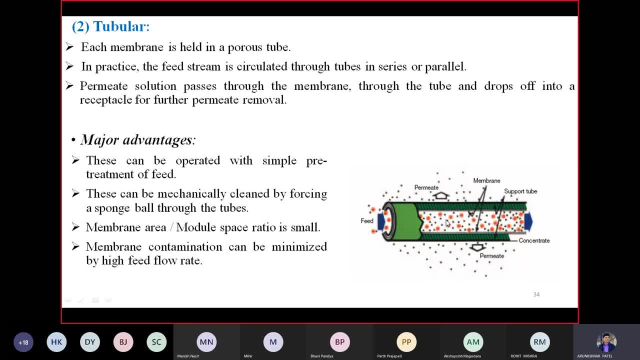 will see in that hybrid technology. it has also certain advantage. this can be operated with the simple pre treatment. with this can be mechanically clean by forcing sponge and ball through the tube. I mean it is. it has an advantage that we can clean up it in a properly and proper way. membrane: 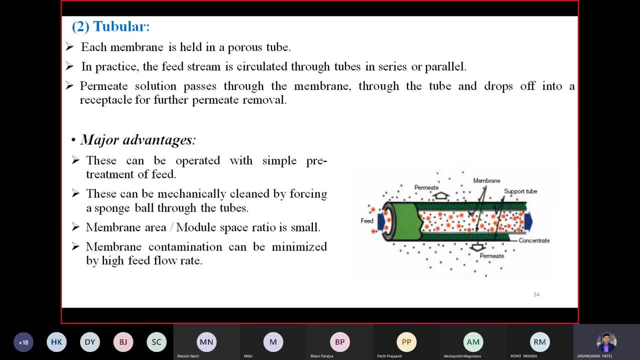 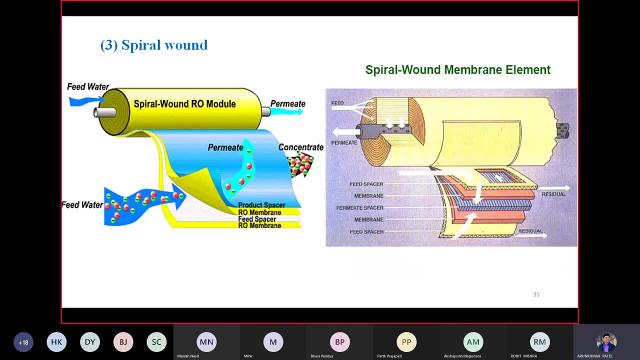 area. model space ratio will be small And membrane area space ratio will be small and membrane contamination can be minimized by high feed fluoride right, so we can maintain this also. it is the one of the most advantageous membrane which we are industrially right now- industrially as well as domestic application we are utilizing. it is the most convenient. 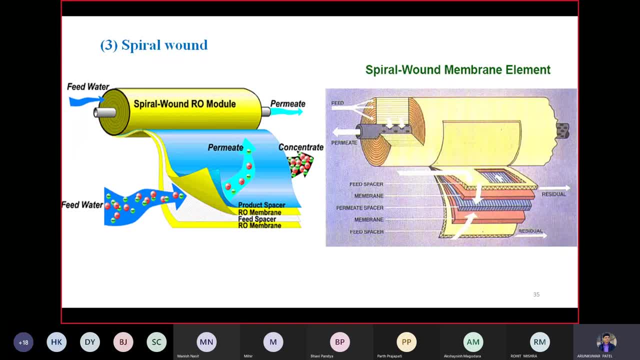 and most appropriate module which generally it is utilized for the industrial aspects also. over here you can see how that, whatever that previous, I was explaining to you. that membrane over here you can say pink, pinkish color, it is membrane, right, moreover, that it is. you can say: 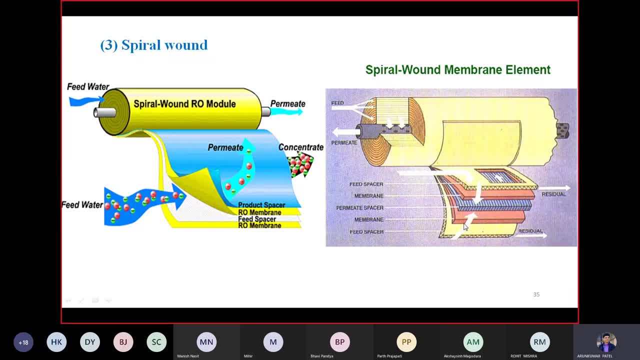 permeate spacer, by which from- and it is your feed spacer in between that you can see over here- you have to apply feed in this direction. so once you are passing feed from here, it will be permeated in a this way and I am sorry, whichever retentate will be there, it will be not pass through that. 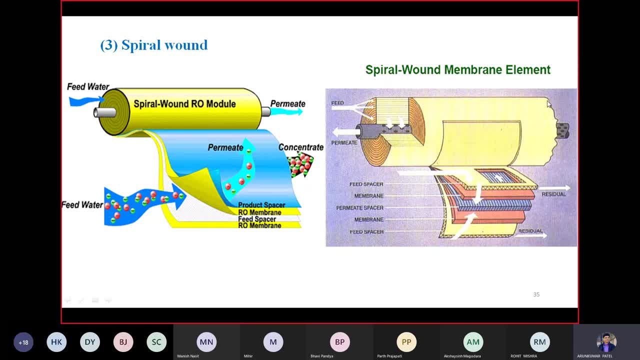 membrane and it will be pass in this direction, over this membrane surfaces. I mean to say over here, he, over here, you can see, over here it is your membrane right and you are passing that feed through this. so what will happen, whichever permeate will be that it will be spirally, it will 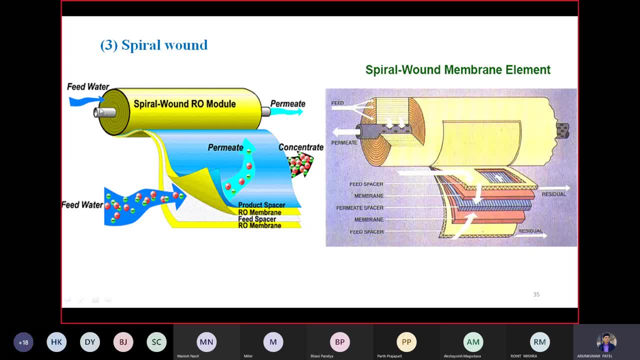 be moving this direction spirally. it is kind of just like a vertical coil and it will go to center point right and whichever retentate will be there, so that permeate will be my all in this direction. over here you can see that field water that will be move, whatever retentate will be that, or you can say concentrate it. 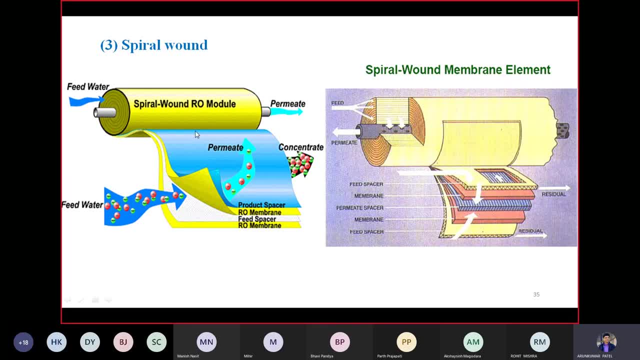 will be moving this direction because name: it will go inside of that spiral to this pipe which is connected at the center over here, which will be porous in through that. we will touch that in that moment, that piece of tell the8325. yet again, this is according to what 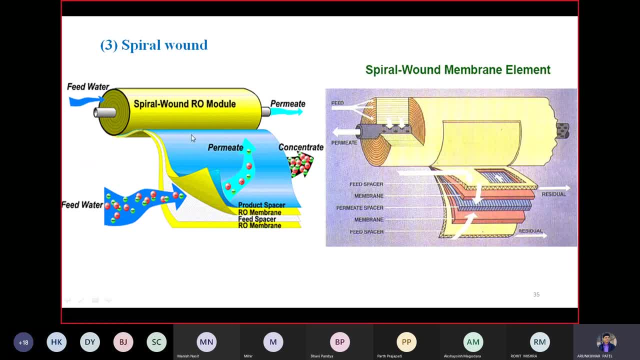 I am saying, within this capsule, the lateral part, and then as a Brian same in term of zapal, are obtaining that permeate. But whichever that rotated particle will be there, it will be, remain on this surface and because of that cross flow mechanism, So various mechanism. 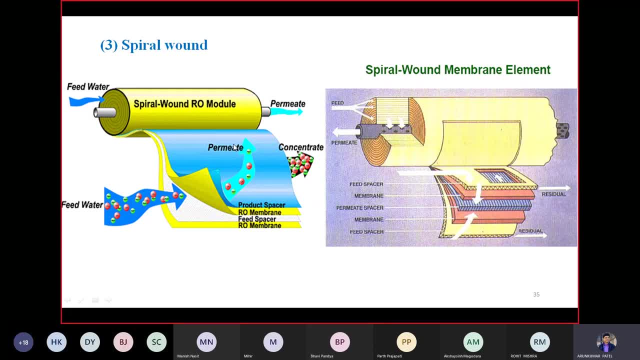 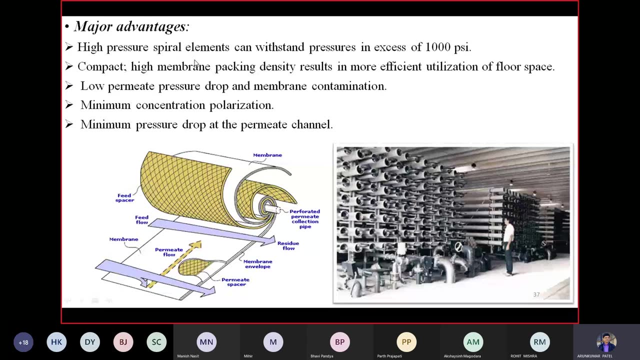 also we will just go through that and that concentrate which will be retained on that surface and it will be passed over here. So this way this module will be work. So basic mechanism I have discussed over here and high pressure spiral element can be withstand pressure. 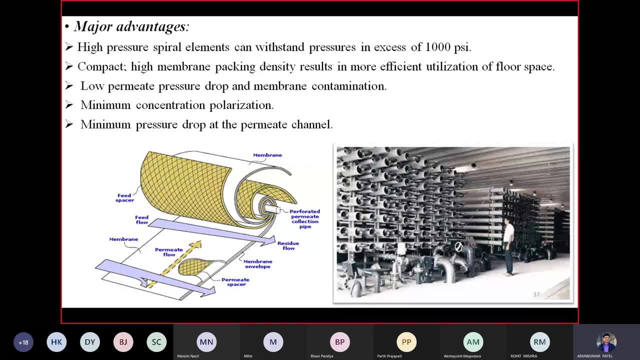 It can sustain pressure of you can say thousand psi. So in pressure driven process it is most important aspect whenever you are selecting that various membranes which must retain certain pressure and it also compact, high membrane packing density result in more efficient utilization of lower space means it is related to that membrane surface area. In small- I mean compact- region also we can 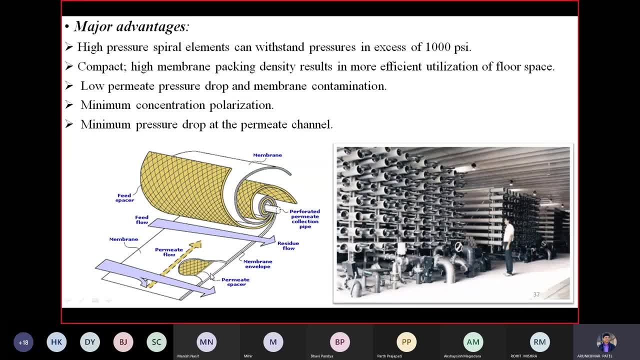 utilize as it is spirally wound, you can imagine, you can say it is multiple. you can see over here it is clearly visible. permeate will be moving this way under direction and it will be gradually moving this way and ultimately reach to that perforated permeate collection pipe and ultimately, 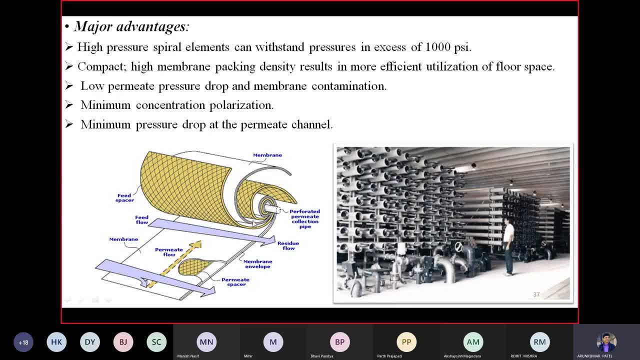 we will get permeate or you can say clean water over here and whichever retentate once that feed will be passed through it, whichever retentate will be that it will be not moving this direction through that membrane and it will be residue flow. you can say that rejected flow which we have. 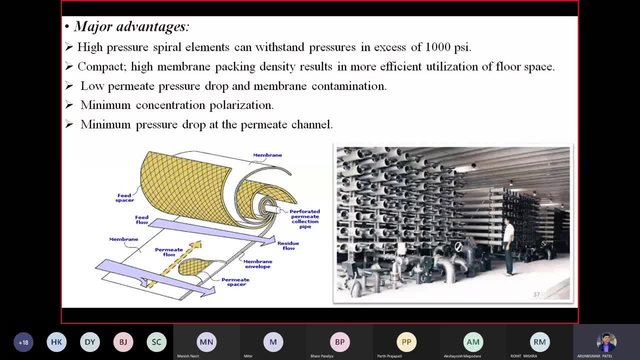 observed in our domestic application also. whenever we are utilizing that plant, there will be a much more rejection will be there compared to that pure water. there will be a- I mean 60, 70 or more than that. there will be a rejected flow and only you can say 10 or 20 percentage that will be. 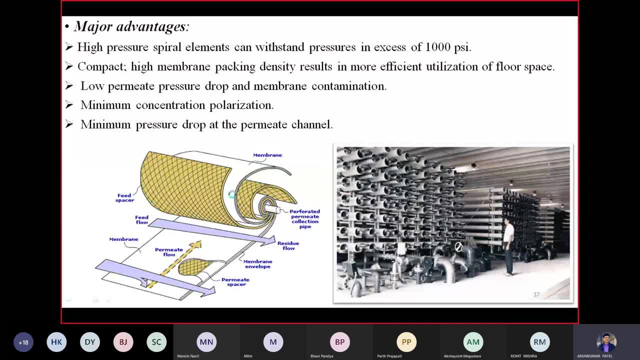 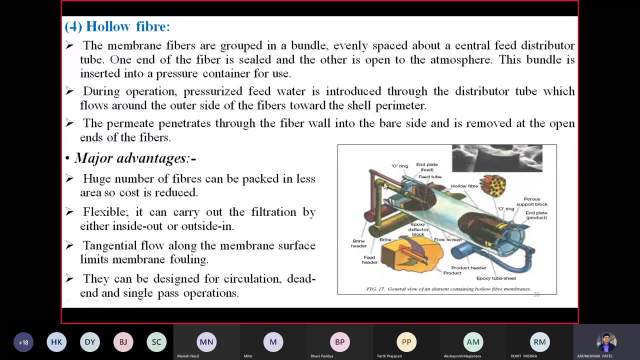 a drinkable water which we are getting, but still it has advantage. it is also hollow fiber. it is kind of, you can say, various fibrous material which we have compactly. you can see over here. these are the hollow. I mean construction of that whole of various fibrous material which we are. 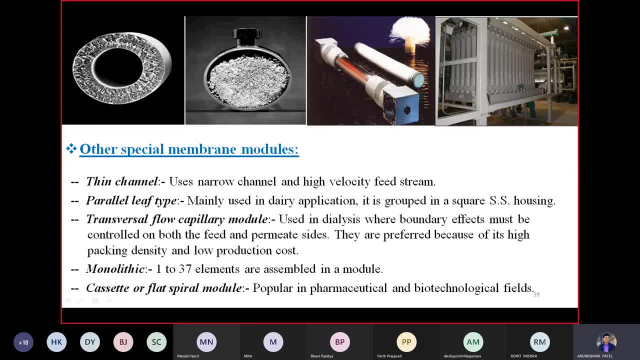 keeping into that module over here. it will be a porous, fibrous material inside of that. I mean into outer, out to. in that kind of mechanism will be happen, in that permeation will be taking place in that kind of high burst material and we can separate out that pure product from that retained. 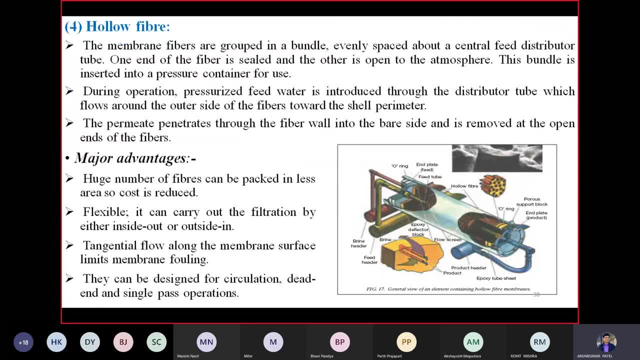 space tented and this way we can have. we can utilize that hollow fiber also, but over here you can say it should have a certain flexibility. it can carry out the filtration by either inside to out or outside to inside. so that depends on requirement how we can introduce that. 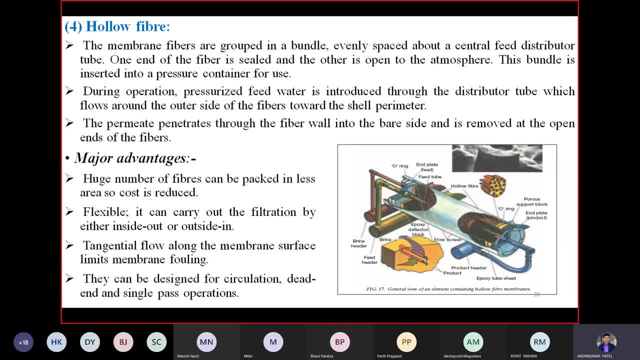 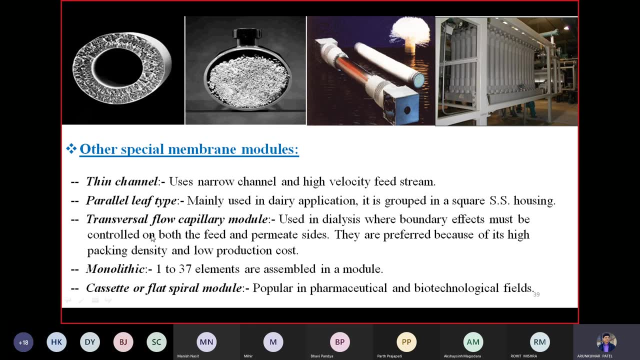 feed material and we can separate out that our desired product. it is depends on the material, but which also utilizes the tangential flow over the membrane surface to minimize that membrane falling. other special material which includes thin channel, parallel lift type transverse flow capillary in module, monolithic and flat spiral module. these are also important modules. 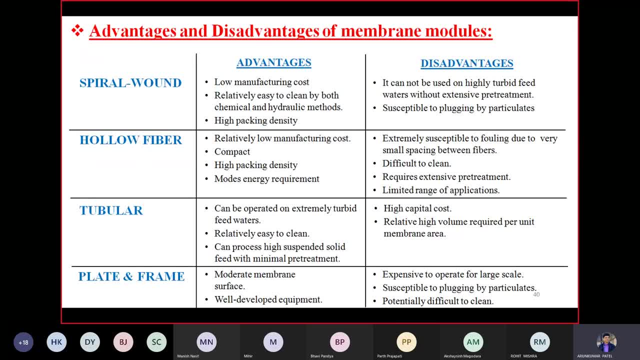 which we can utilize right. these are the advantages and disadvantages of membrane module. spiral wound module. seen in that advantages and disadvantages, although also spiral wound, low manufacturing cost, relatively easy to clean up right. high packing density in case of the spiral work. but disadvantage, it cannot be used in highly turbid fluid water without extensive pre-treatment. 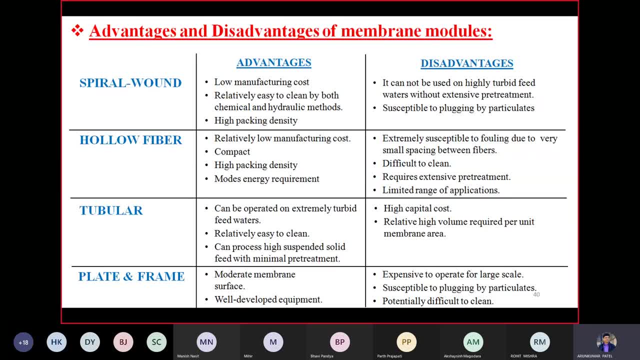 right hollow fiber membrane. relatively low manufacturing cost. it is compact, high packing density. these are the certain advantages. but it has a difficulty in cleaning. these are the disadvantages. tubular also in care we can operate, exploit turbide feed water. even you have the, we have the turbidity. in that case also we can utilize. but 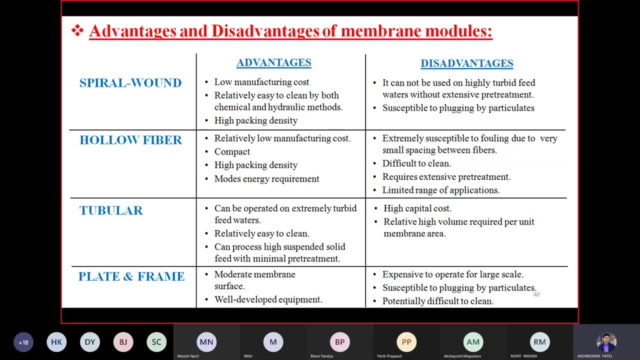 it. it is costly, high. it has a high cost right. apart from that plate in frame module, well developed equipment, expensive to operate for a large scale. it has certain limitation because we- that plate in frame module- cannot provide that much surface area and because of that we you cannot. 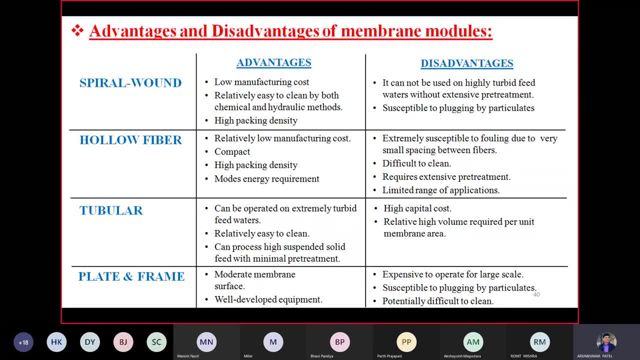 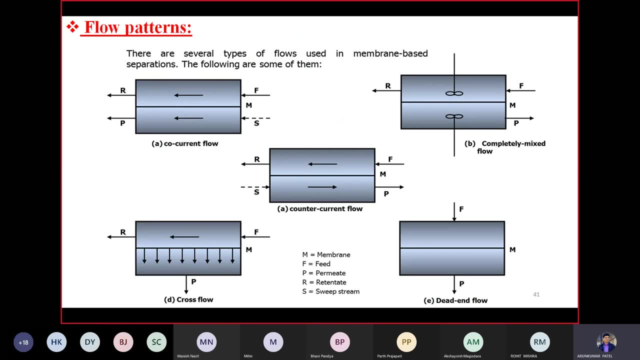 have a very, you can say, laboratory scale to pilot scale, to commercialize scale. it has a certain difficulty. so for the r? d purpose and other small research work only we can go through that plate and frame module, otherwise alternative modules we, we just have to go through it. it is uh, flow patent we. 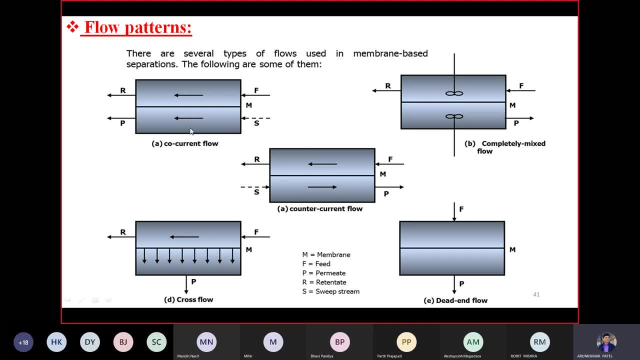 are familiar with, uh, these ones, so we will not much more go into detail. co-current mechanism: you can have to understand. it is your membrane and how you can. which is the membrane and how you can, uh, you can pass your uh feed material right and how that, uh, i mean uh, that feed material will. 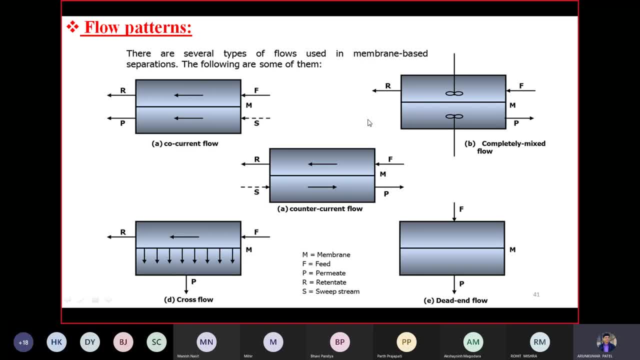 behave in that flow mechanism. but uh, over here you can see once uh, that completely mixing flow. once you are passing your feed material over here, then the retentate will be get from here and permeate which we are getting over here. it is very easy uh to get from the material which is being passed to the 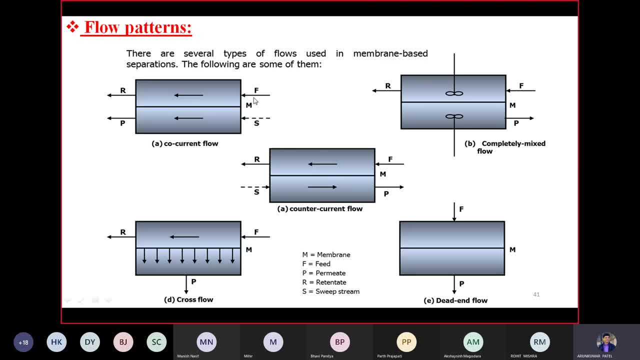 will be completely mixed mechanism, but over here you can pass feed material and retentate will be even. even your product will be moving this direction only, so it will be retented as well products. it is moving in a common direction, so that's why we are calling this co-current. 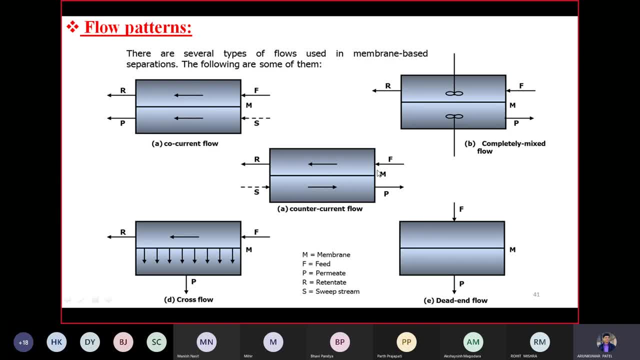 counter current which will be obtained in reversible mechanism, complete mixing also. even it is most viable technology of cross flow mechanism in all cases. generally we are utilizing this, not in the counter current also, but in our almost all technological aspects. we are utilizing cross flow mechanism. once we are passing this feed material and retentate will be. 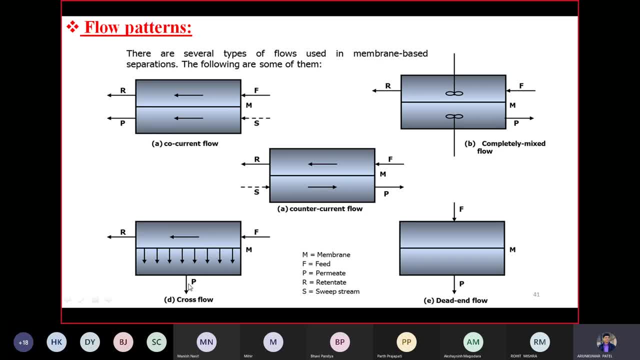 getting at the other end, but that, whichever permeate, we will allow to pass through it. it will be permeate through core and it will be at, you can say simply, in a 90 degree angle. so, once, what is the advantage of this cross flow mechanism? so, in this cross flow mechanism, what will happen? 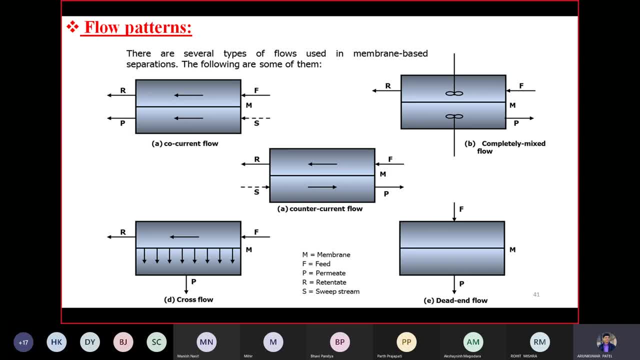 so in this cross flow mechanism that permeate it will be passed through it. and whenever you are applying force pressure, if it is pressure driven technology, then whatever retentate that will be deposited over that membrane surfaces, so that membrane surfaces, the whatever that particle it will be deposited, that will be washed out through that feed material at the high pressure. 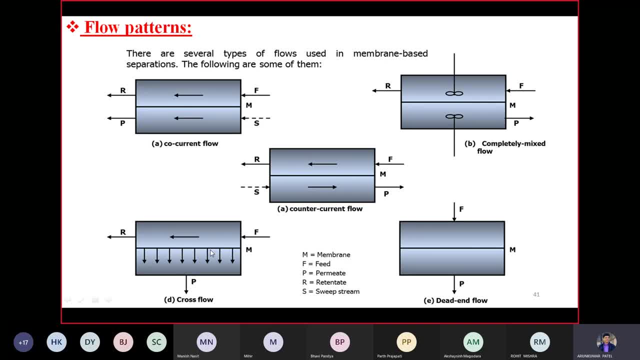 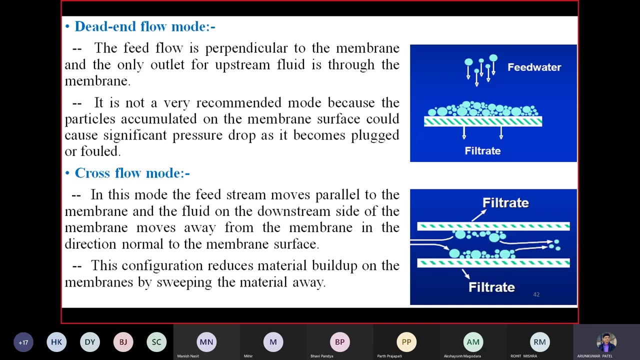 of that cross flow mechanism we can avoid certain concentration polarization or you can say particle deposition over the membrane surface and a regular interval, even though there will be a scaling and concentration polarization as well as membrane falling also. but in certain up, to certain extent we can uh shaft it by this kind of cross flow mechanism. right, it is certain technology dead. 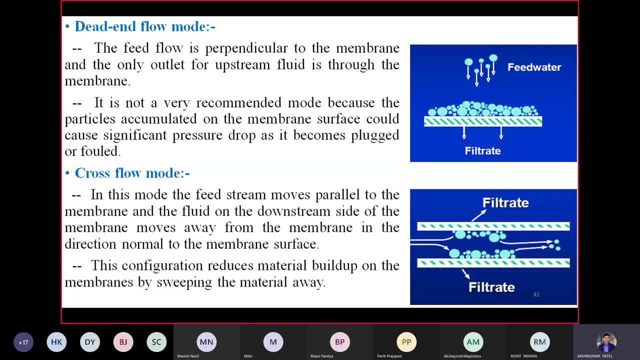 end flow, once it is simply a conventional filter mechanism, where we are applying cross flow mechanism directly, pressure over here and we are getting that filtered from the bottom, and cross flow mechanism you can see over here, as i explained earlier also, so we can choose either of that. 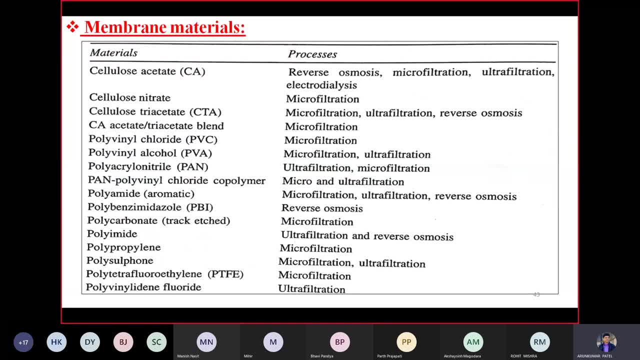 mechanism. these are the different materials: cellulose acetate, cellulose nitro, i mean. whenever that thing, i mean material- come into picture, we must have to uh see that cellulose and its derivative. it is one of the most efficient material which regularly we are utilizing for in membrane technology, ca ct. cellulose triacetate. 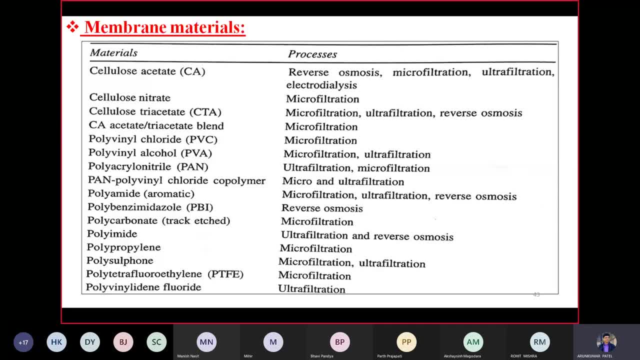 cellulose acid, polyvinyl chloride, pva, also pvdf also. pvdf is also, i mean, strengthened material, which also we can utilize- uh for the membrane separation, pa and polyvinyl chloride polyamides, even polyamides also, which we are using. based on our application. we must have to go for the 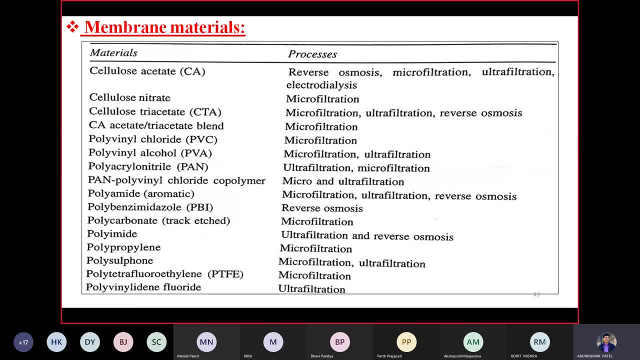 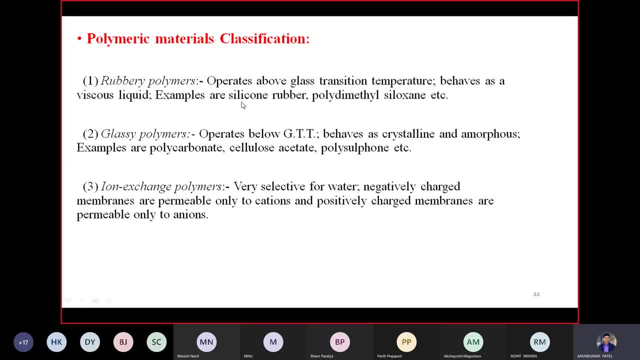 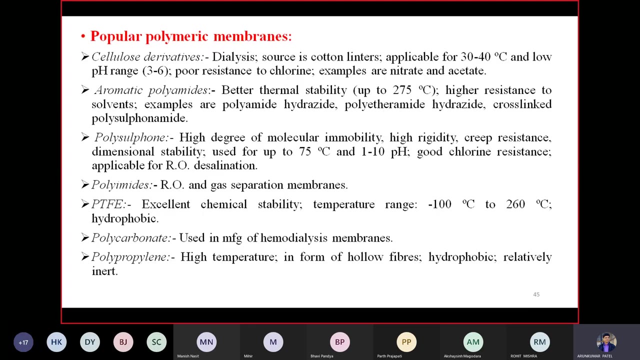 uh product which we have desired and accordingly we can have to select uh, that membrane material for the different different processes. right polymeric material, it may be rubbery polymer, glassy polymer, ion exchange polymer. based on its- i mean- characteristic behavior of that polymer. we can classify according to its temperature and its sustainability. we can classify it. 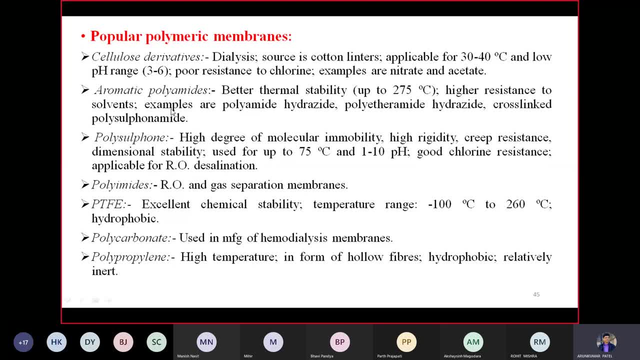 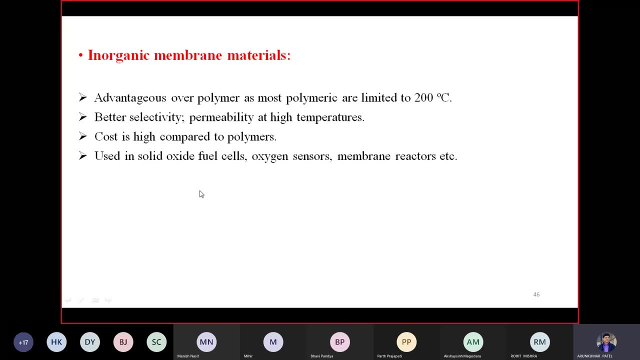 right. well, yes, as i shared. cellulose and its derivative aromatic polyamide, polysulfol, ptfe polyamide. these are the materials which is mostly highly utilized for the membrane technology: polycarbonate and polypropylene. these are the material which we are utilizing. inorganic membrane material, as we have already discussed, it is uh. 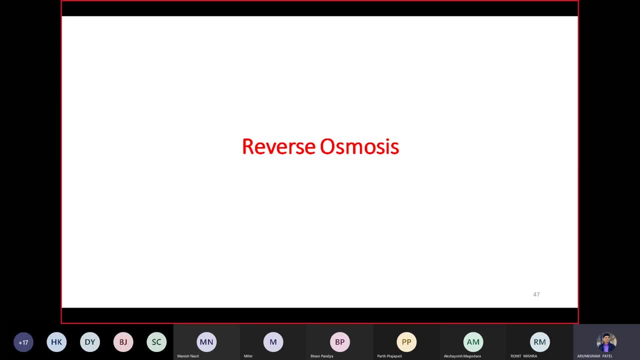 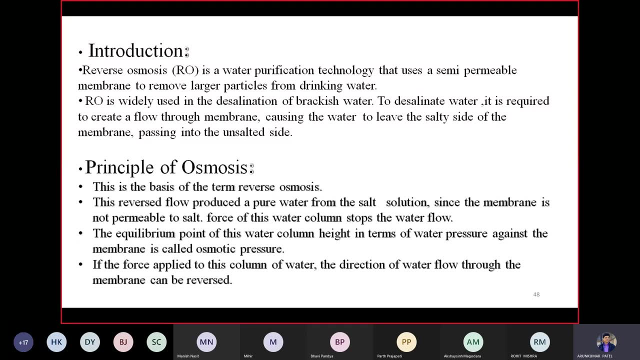 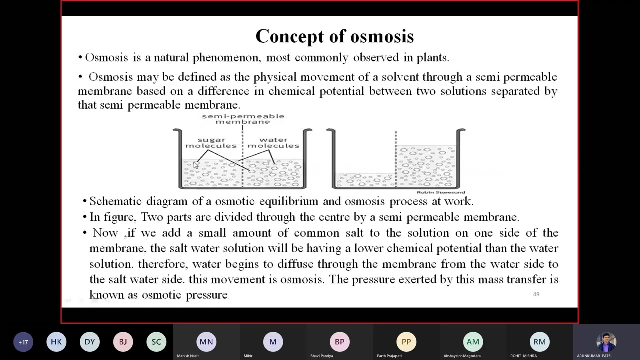 used for the higher temperature purpose, right? so, uh, you might have uh gone through that. i mean you now we are familiar with that various component. now we will uh quickly go through that various processes which we have adapted. uh, reverse osmosis: you might have familiar that reverse osmosis technology over here. i will go through that conceptual because 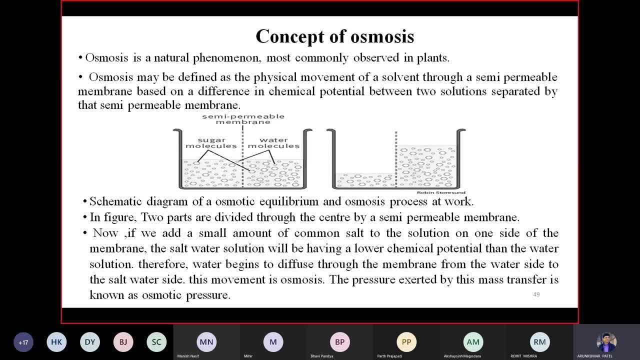 right now i am on 50. i have more than 125, if it is so, i i have just not covered only 50 percentage of my content, so i will go a little bit fast right. so over here i will just concentrate on conceptual only and after that we will move a little bit fast. right now, uh, 3, 20, 3, 22, 9 mm. is there please? 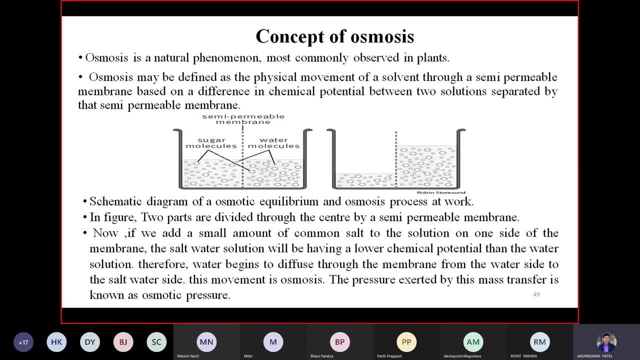 hello, okay, he will. i mean, she will join very soon, uh, but because of uh one, the speaker's absence, second session will be conducted by naina mem, our one of the second coordinator of this cdb. i mean, apart from me, uh, they will be conducting. So I will take little bit time and I will whatever I have targeted in my presentation. 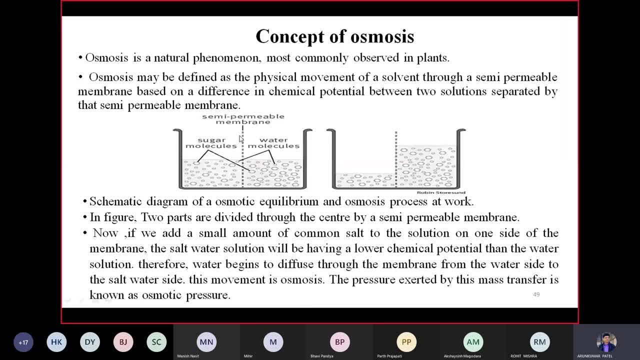 I will go to that. So over here you can see, over here we are putting that semi-permeable membrane. We have that different concentration solution over here, different concentrated solution over here. You will observe whenever you are putting that kind of that membrane you will observe.